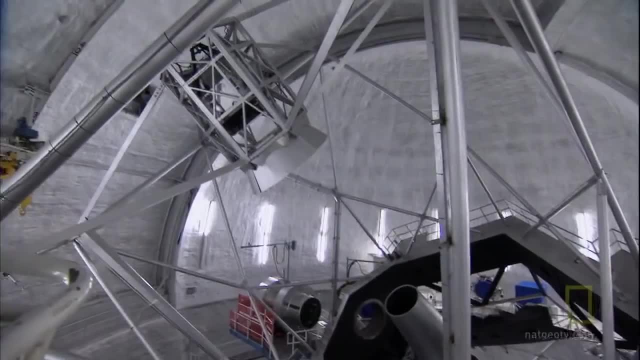 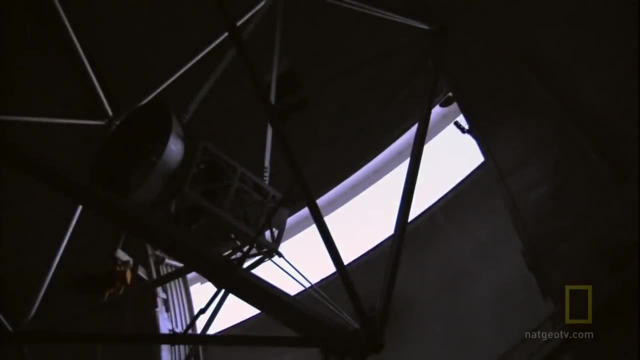 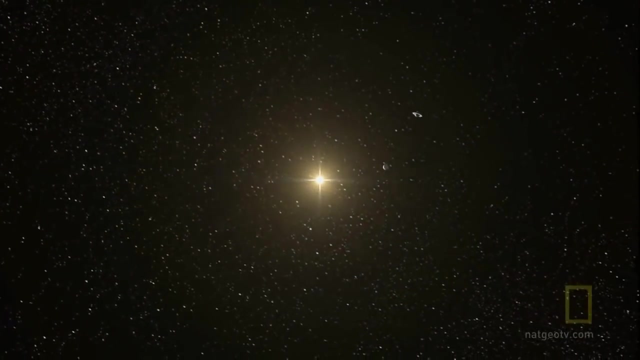 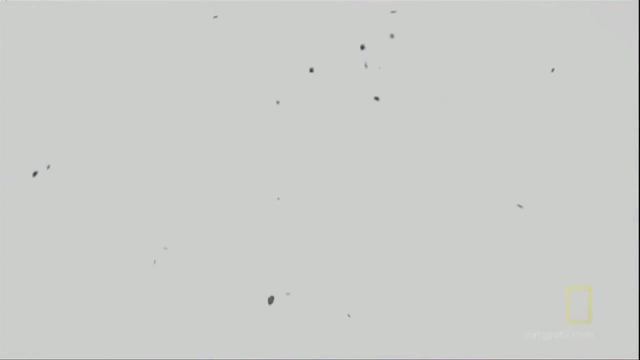 Figuring out how it will end is the challenge of astrophysicists around the world. They're pointing high-tech equipment out toward the heavens to unlock the secret of our fate. The possibilities are frightening. In one scenario, gravity pulls the universe back into itself, similar to air being let out of an inflated balloon. The universe goes back to its original size. This is the Big Crunch. That would be the end of the universe in a big fireball, as all the matter collapses onto itself. That would be pretty dramatic. Then there's the Big Chill. The universe expands until the nuclear furnaces that power all the stars burn out. The universe grows cold and dies. A second possibility is actually kind of sad. The universe will continue to expand forever and it will just grow into an increasingly cold and lonely place as the expansion removes our nearest neighbors from us and we just end up a single isolated community of stars and galaxies. 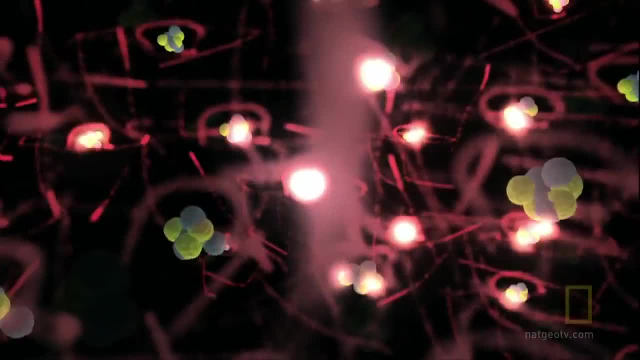 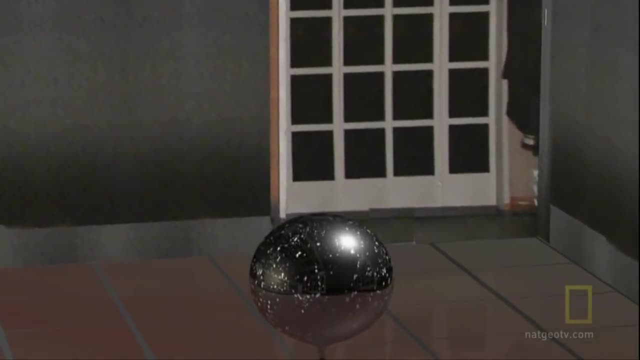 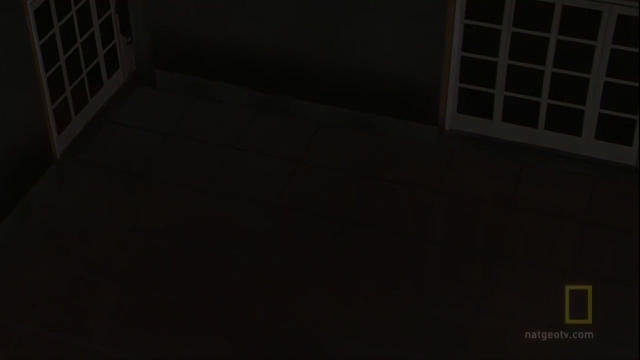 Then again there could be a much more spectacular end in which everything is ripped to shreds, down to the last atom. Think of it like a balloon that is filled with too much air: It pops. It's much more dramatic than the Big Chill and just as fateful as the Big Crunch. 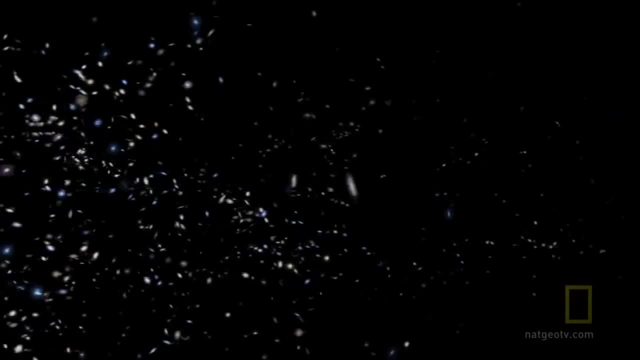 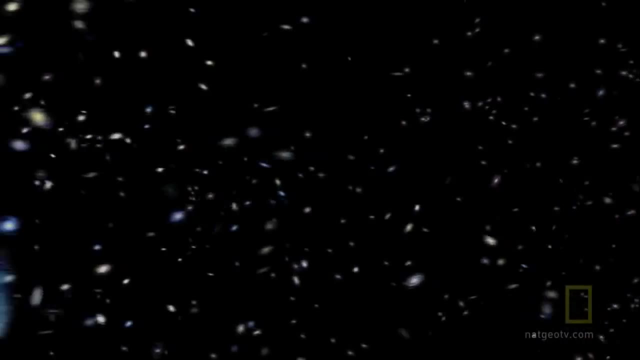 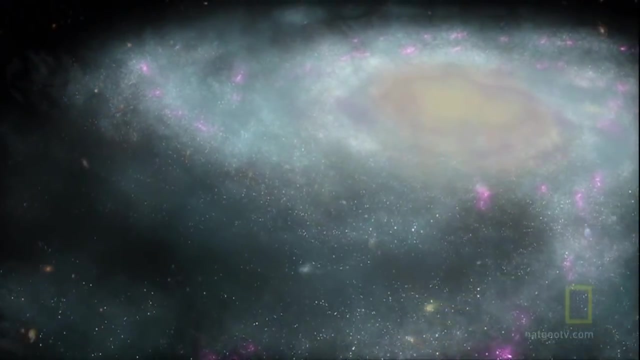 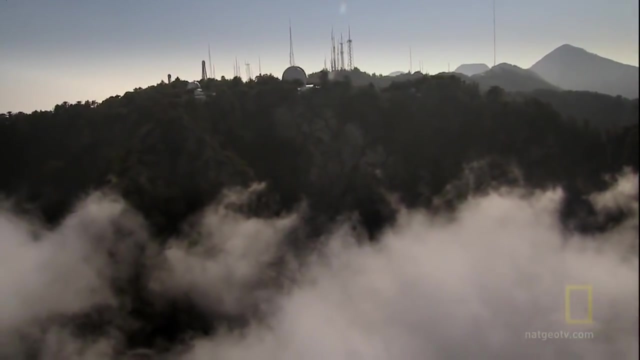 The universe continues to expand, but at an ever-quickening pace, And in fact the pace is so great that even the space-time fabric cannot hold the universe together. However the end comes, it will be a dramatic conclusion To understand how it all could end. scientists turned to how it began. 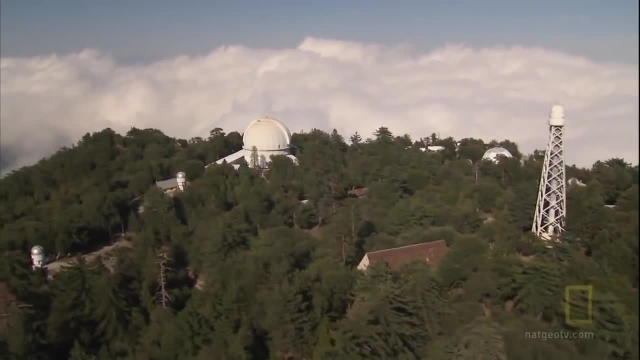 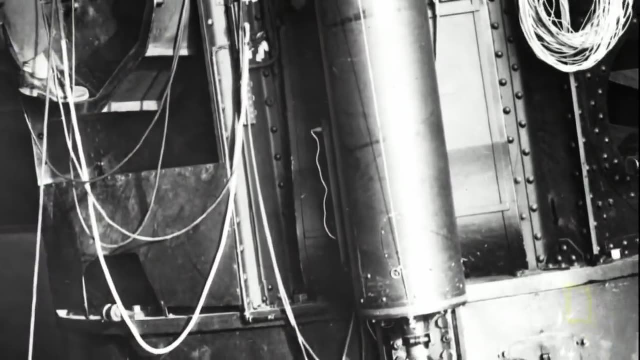 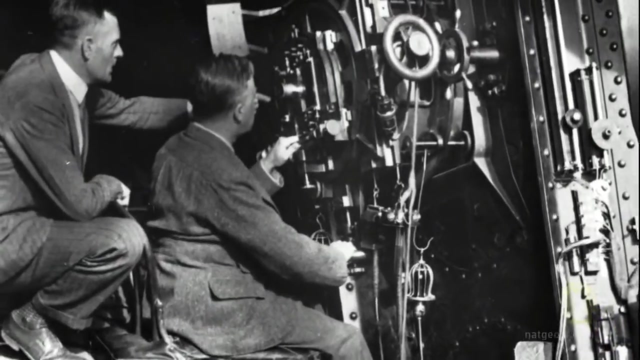 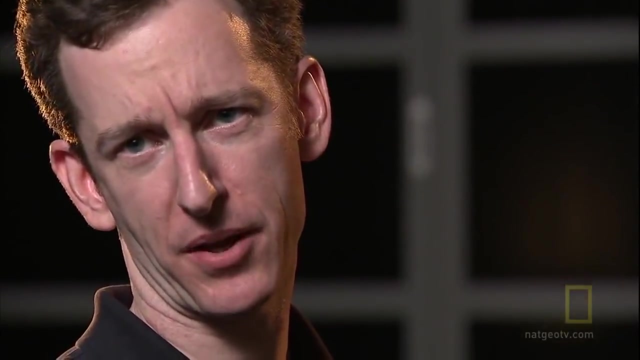 The mystery starts to be solved here, at the Mount Wilson Observatory. overlooking Pasadena, California, In 1929, while looking through what was then the world's largest telescope, Edwin Hubble makes a strange discovery: The universe is expanding. Hubble's discovery led to a whole new picture of the universe: that it was a dynamic environment and that it evolved. 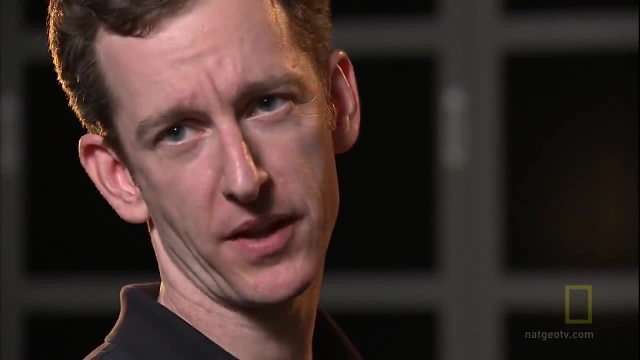 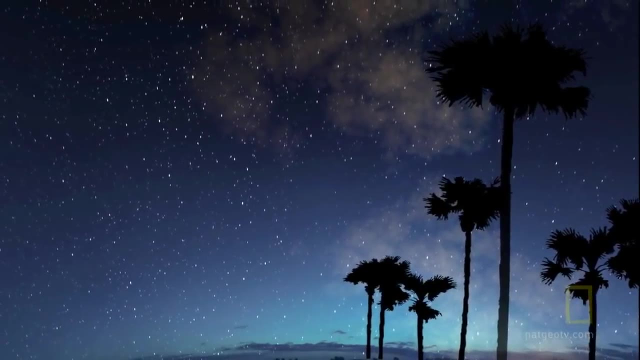 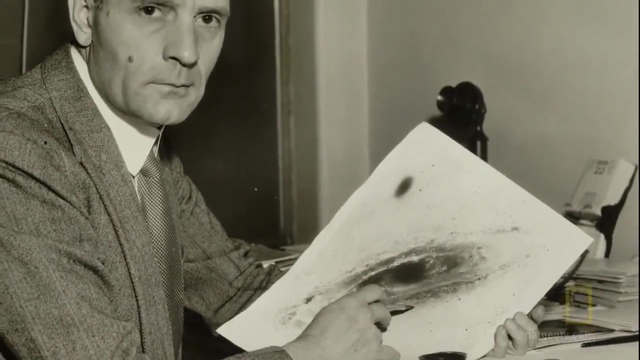 It changed in time and that's different from pictures that people had of cosmology previous to that. Before Hubble, scientists said that the universe was static and unchanging. Hubble's discovery that the universe is expanding meant it had a starting point. 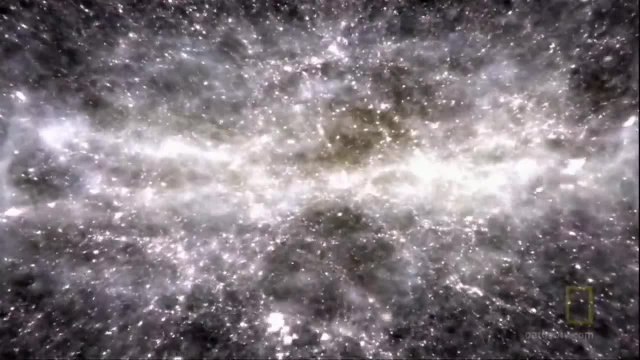 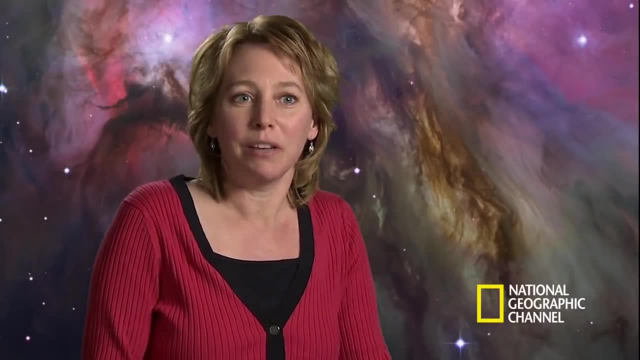 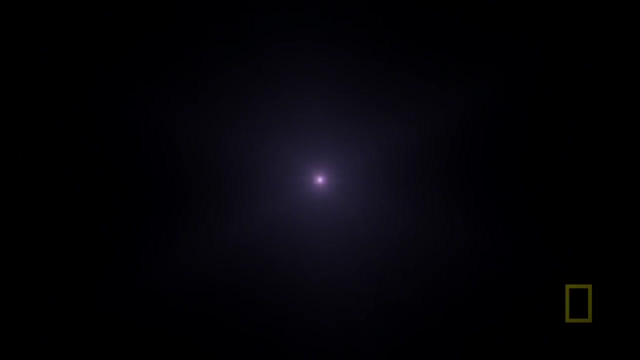 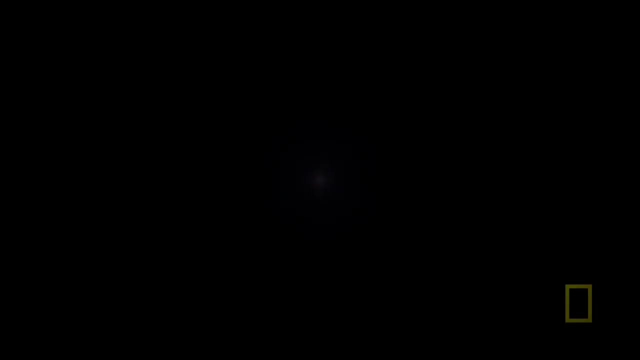 A beginning That brought the idea forward that, hey, what if we ran the film backwards in time and found the point at which that began, The Big Bang, That fraction of a second when the universe and everything in it exploded into existence from a point smaller than an atom? 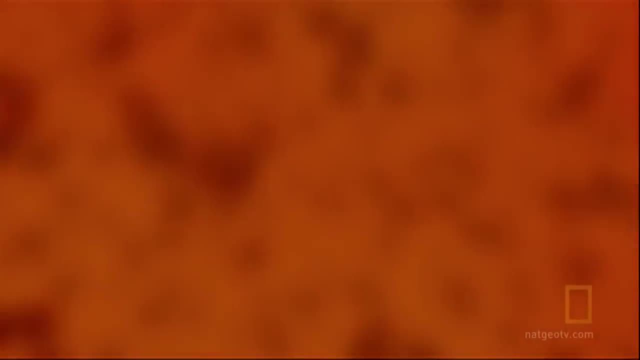 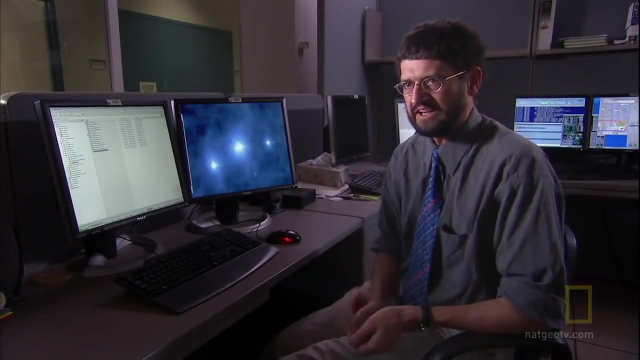 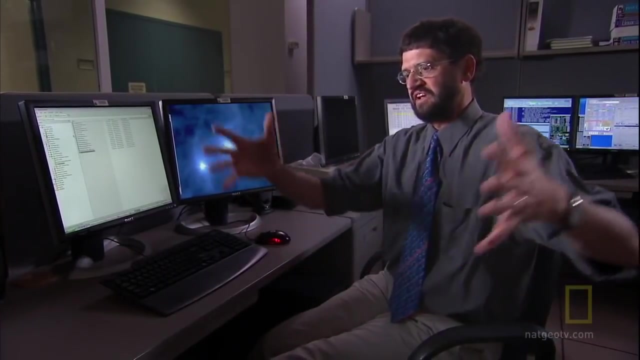 The Big Bang. One common misconception about the Big Bang is that we can identify a point in space where the Big Bang occurred, But in fact it's more appropriate to think of the Big Bang as a simultaneous creation everywhere in space, which is then continuing to expand to the present day. Scientists theorize that at the moment of the Big Bang, the first small particles of matter called quarks were produced. They collided to form the building blocks of the universe. These floated in a thick fog of hot plasma for about 400,000 years. 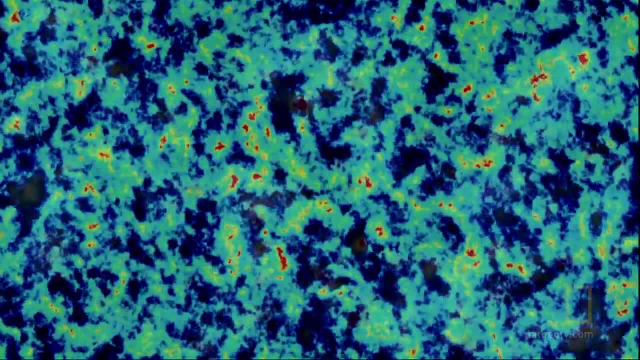 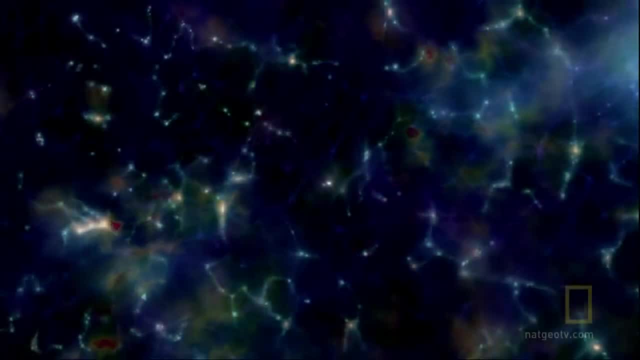 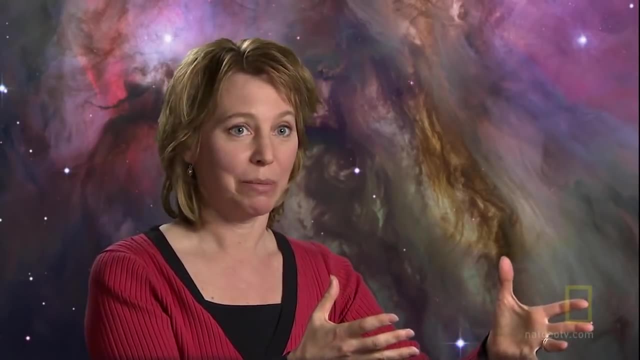 Gravity, also created at the Big Bang, drew the particles together, eventually creating the first stars and lighting up the cosmos. The theory of the Big Bang is a very solid theory. What happened at the moment of the Big Bang is still something we're working on. We don't really understand. If the universe has been expanding since the Big Bang, scientists must consider that it will stop expanding at some point. The question is how, How? The most obvious answer involves gravity: What goes up must come down. 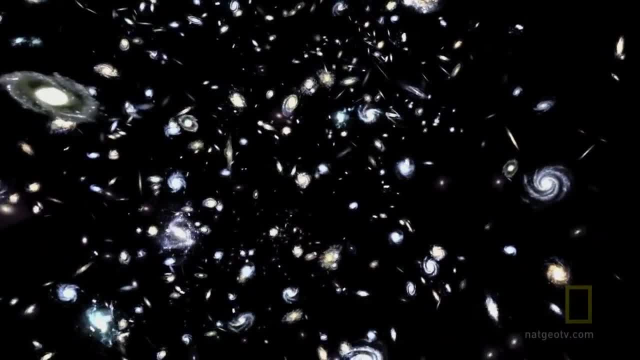 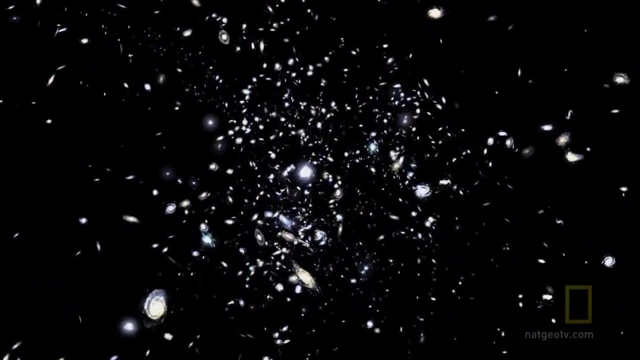 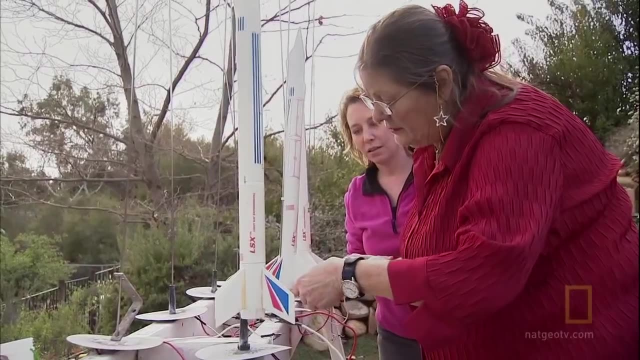 Stars and galaxies and everything else might reverse direction. The universe would collapse in what some scientists call a big crunch. Take the top and then see the other handle and just jerk them apart. A model rocket offers clues to how the big crunch would work. 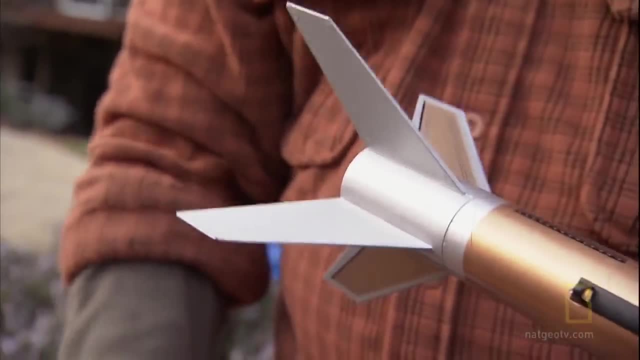 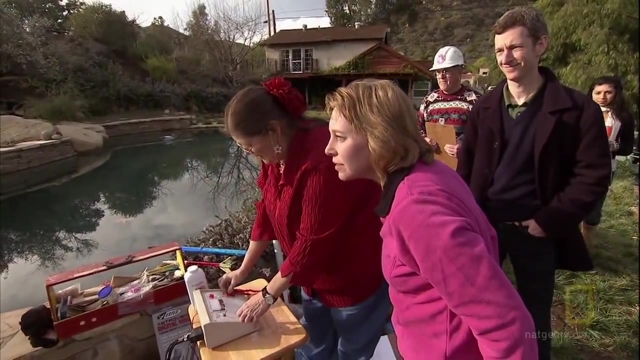 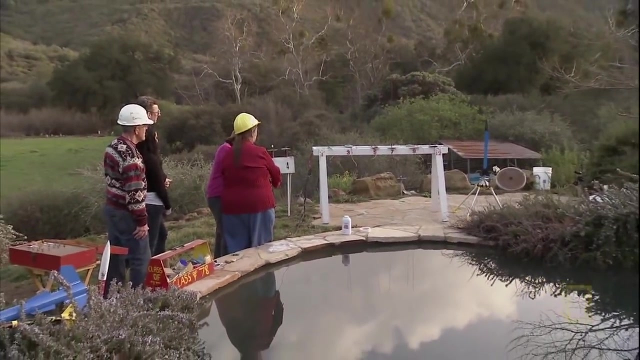 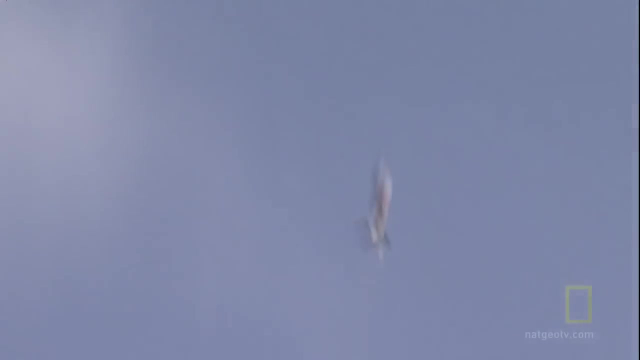 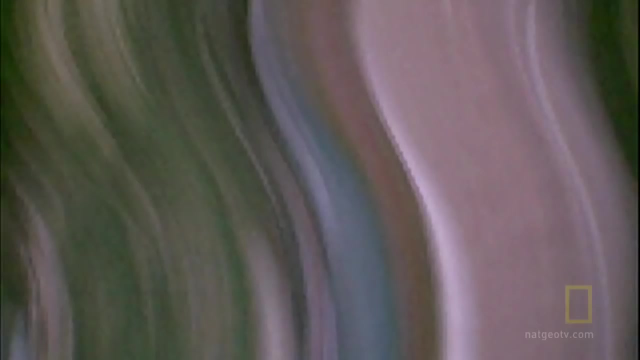 The rocket is like the universe, expanding into space out of the Big Bang. An initial bang allows the rocket to overcome the pull of gravity: Five, four, three, two, one. Eventually, when the fuel is exhausted, the rocket coasts a few feet higher, stops and is pulled back to Earth. 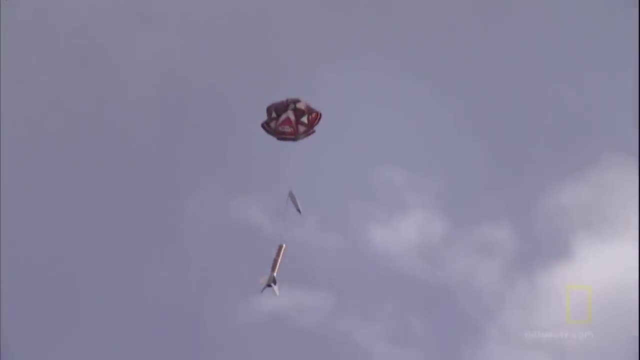 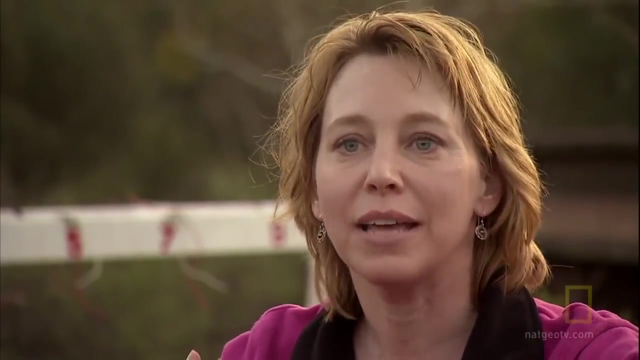 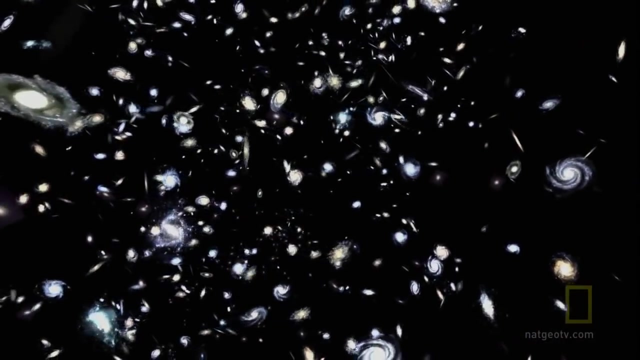 This is what would happen with a big crunch: The entire universe is essentially pulled back to its launch pad. The universe itself has its own momentum, its own energy. It's moving outward, But eventually there's a point where possibly the universe will stop that moving outward. 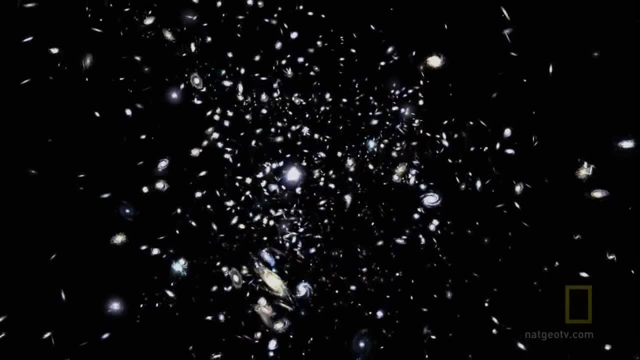 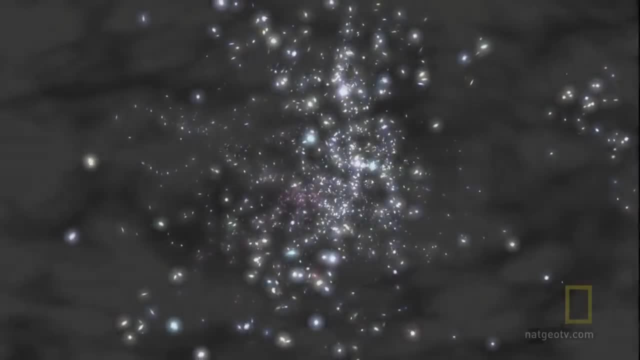 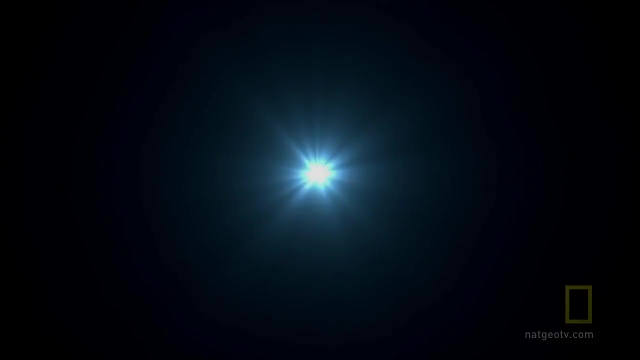 just like the rocket that we saw, and have to fall back in upon itself and collapse again under the force of its own gravity. In this scenario, the universe could return to its original state just before the Big Bang, setting the stage for a perpetual seesaw of creation and destruction. 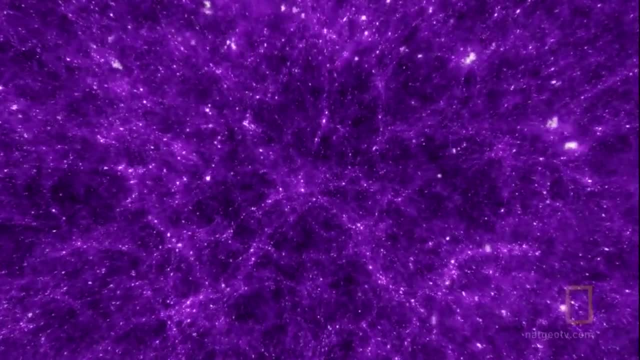 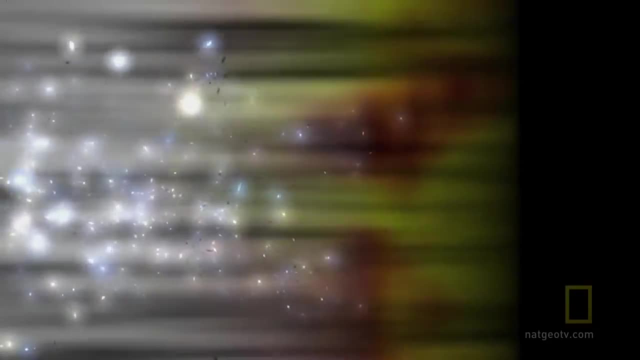 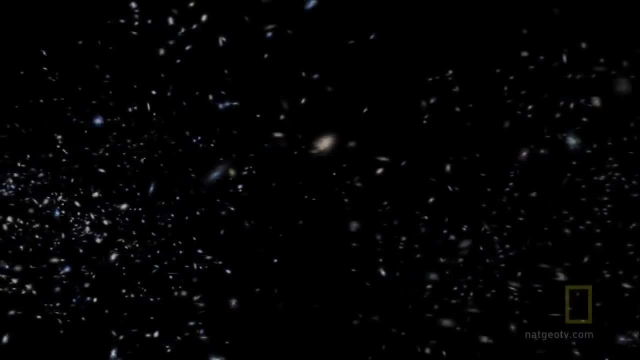 The big crunch theory moved to a scientific backburner. Cosmologists figured out that there must be some form of energy that keeps the universe from collapsing. The existence of such a force leads to new theories about what the universe is made of and how it might end. 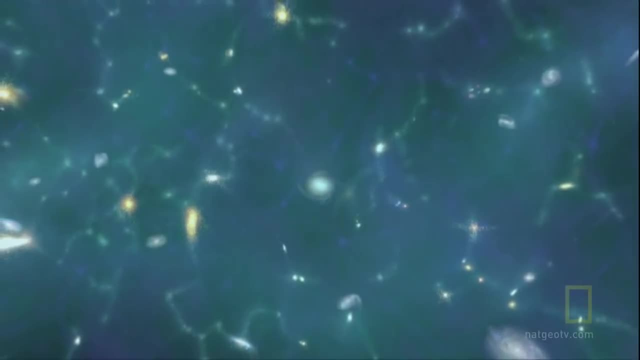 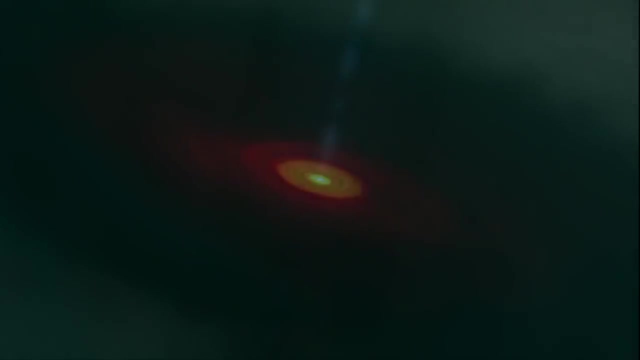 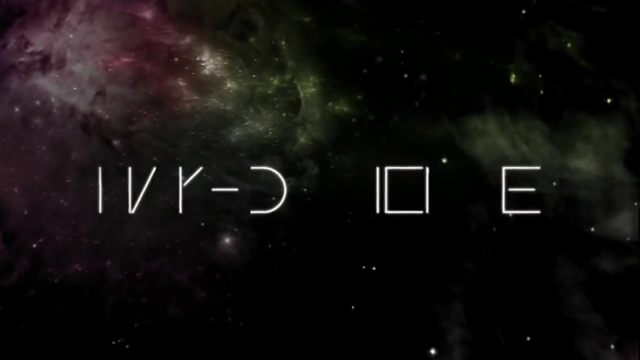 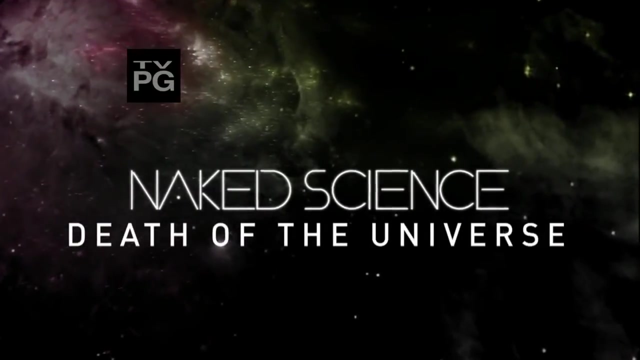 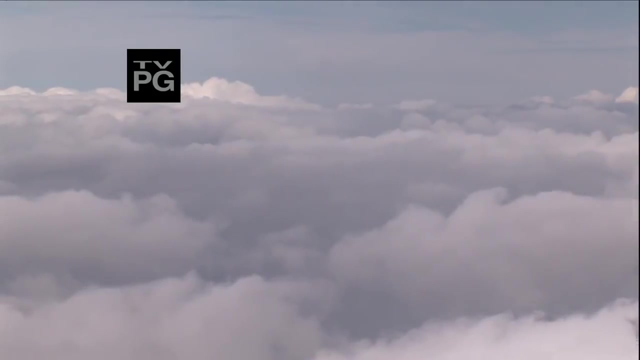 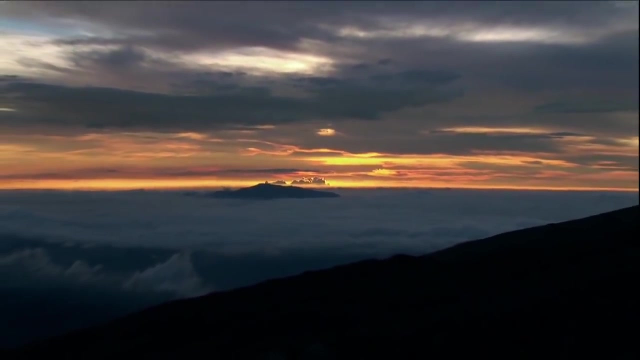 And evidence about how this might play out is found in some of the most powerful and mysterious phenomena in the cosmos: Black holes. Predicting how the universe will end involves some of the most advanced technologies known to man. On a remote volcano on the island of Hawaii, astronomers are monitoring a battle in space. 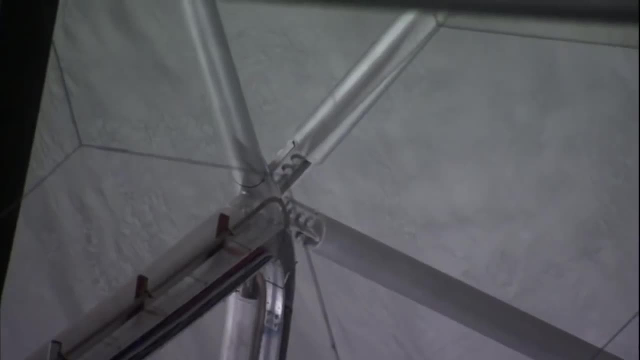 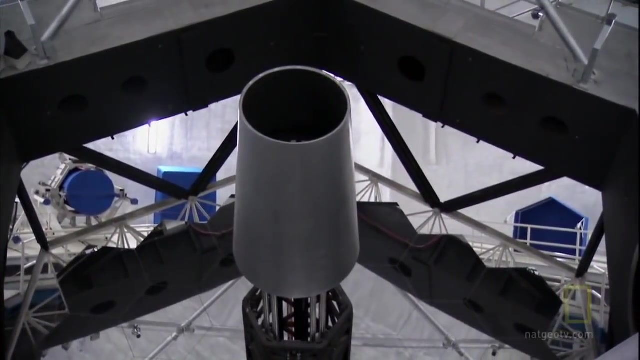 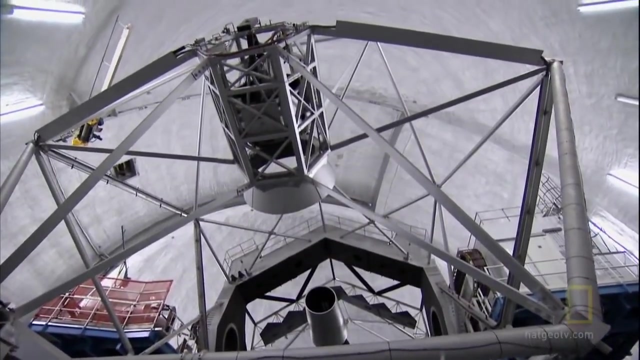 that is shaping the fate of the universe. At an elevation of nearly 14,000 feet, the Keck telescopes bring astronomers from all over the world nearer to space for a clearer view of the cosmos. They come here because the telescopes work best far away from Earth. 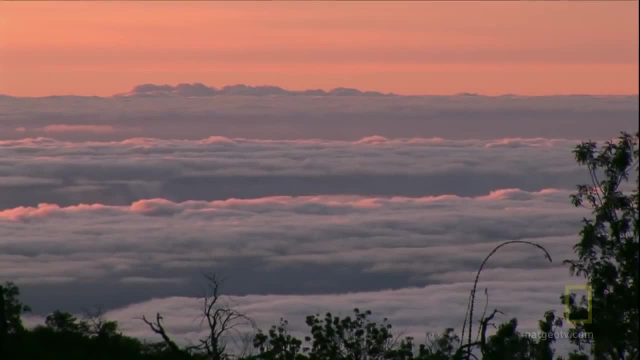 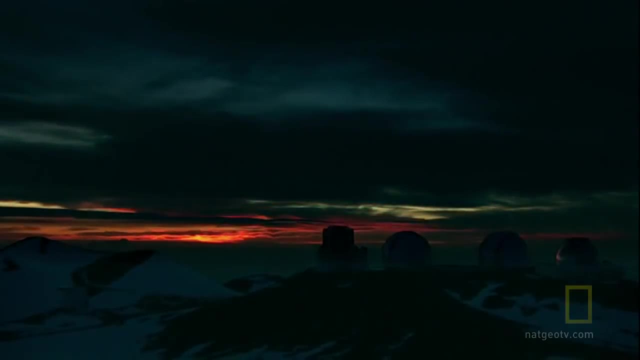 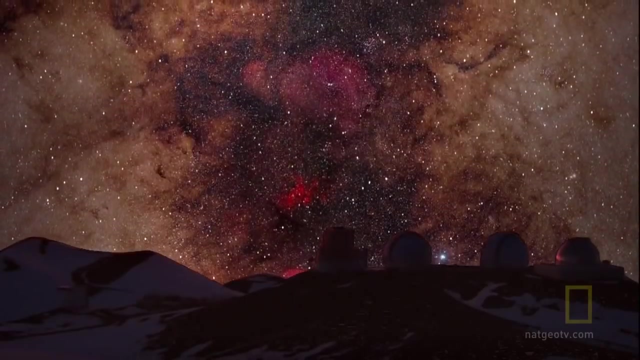 They work best far away from city lights and as high as possible above Earth's polluted air. Harsh conditions make it difficult to work here, but for scientists in pursuit of the great mysteries above, it's paradise. So this is a remarkable location. 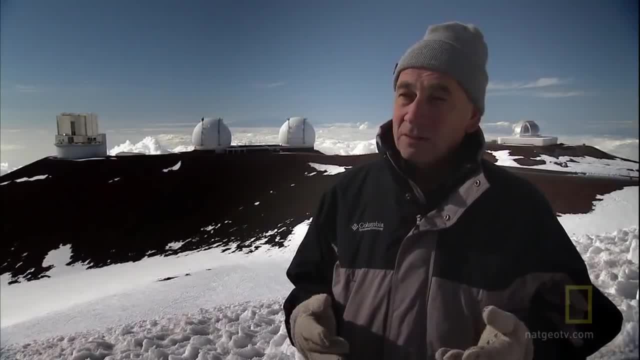 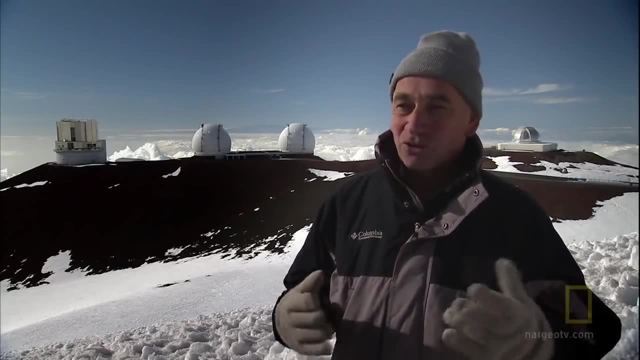 But of course the air is very thin. it's extremely hard to work here, But these telescopes are amazingly powerful. But we're ambitious astronomers. We don't just stop looking at easy objects. We try hard to look at the very faintest objects. 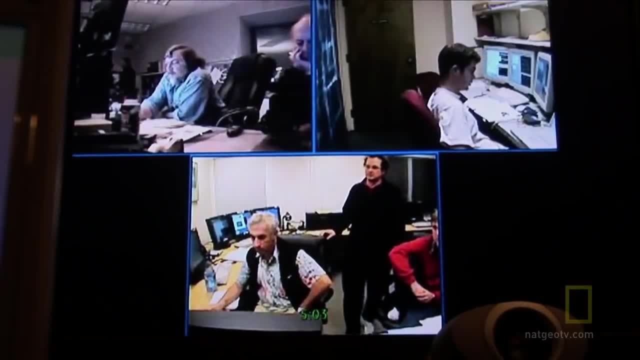 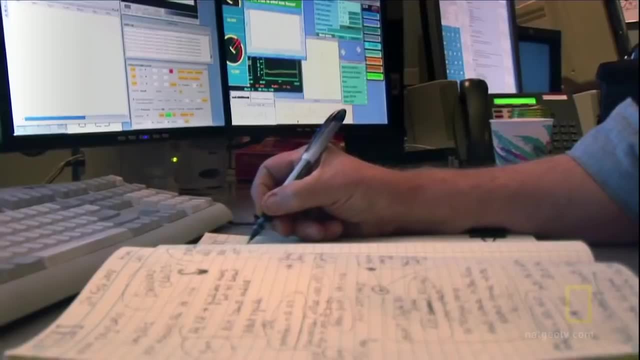 so we can understand the extremities of the universe. Here, astronomers like Richard Ellis are working on a problem that has been all-consuming for cosmologists since Edwin Hubble. They know the universe is expanding, but what they don't know is how fast. 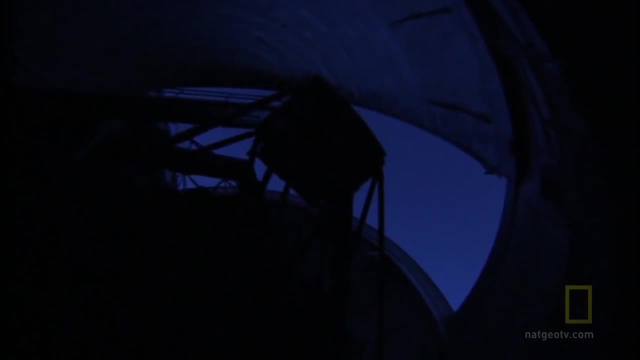 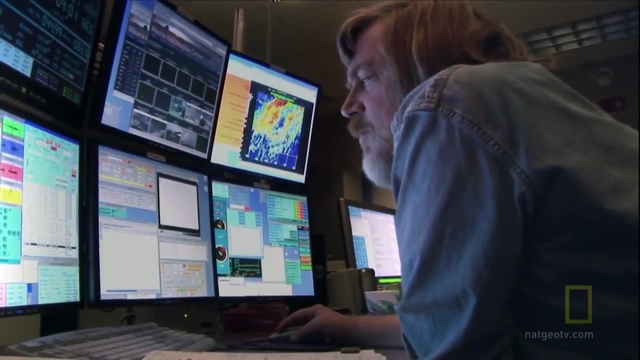 It will be difficult to predict exactly how the universe will end until they solve this mystery. The answers lie in the past. Now, what we were looking at, what I did the focus on, was a V equals 12.. Okay, that's the right star. 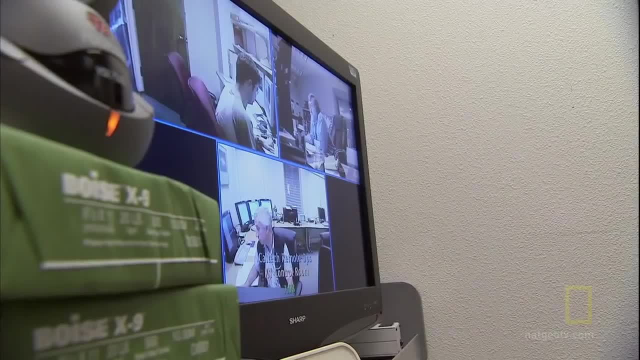 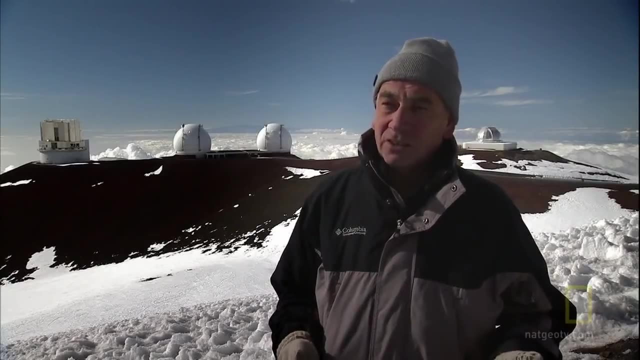 We'll get a better focus now. That was worth doing. An astronomer like myself uses a ground-based telescope as a time machine. We're looking back in time to study distant galaxies seen as they were a long, long time ago. One of the distant galaxies that astronomers found 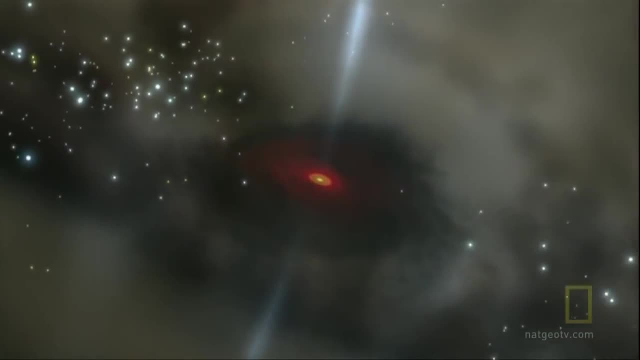 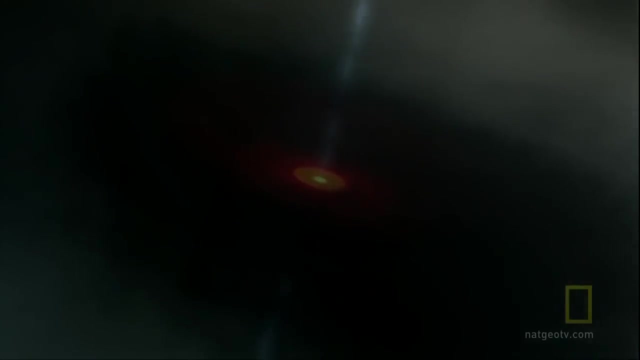 revealed a powerful source of X-rays from something that they could not see. It was in the constellation Cygnus and emitted no light, But something was there, Whatever was emitting. these X-rays had a mass about seven times that of Earth's sun. 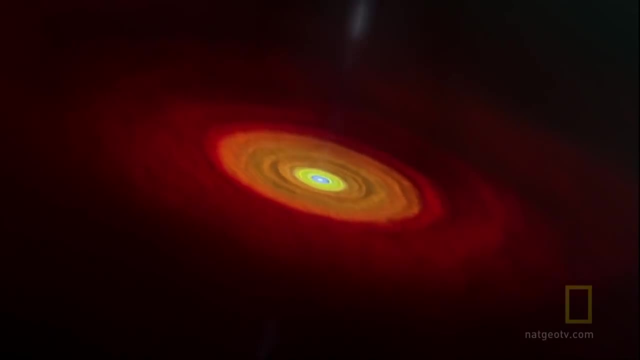 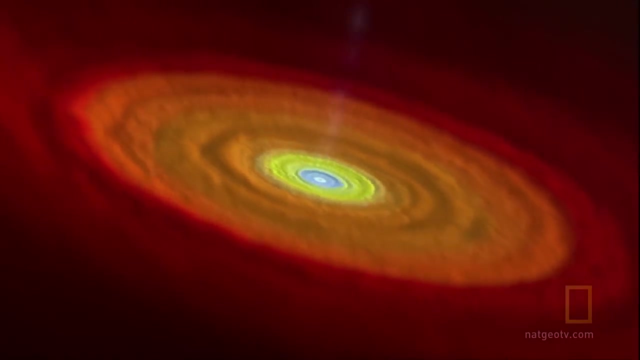 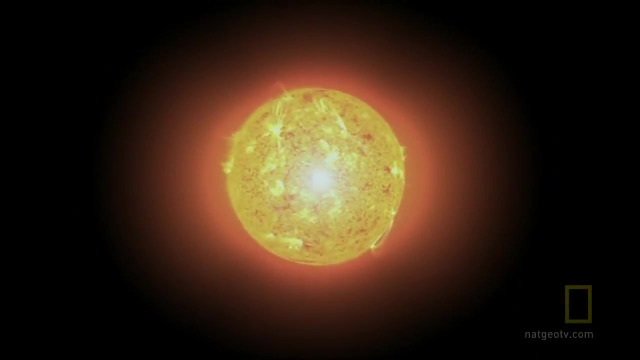 There wasn't a name for it, so they called it a black hole. Black holes offer scientists an analogy to how the big crunch theory works. When certain stars run out of fuel, they collapse in on themselves into a smaller and far denser mass. 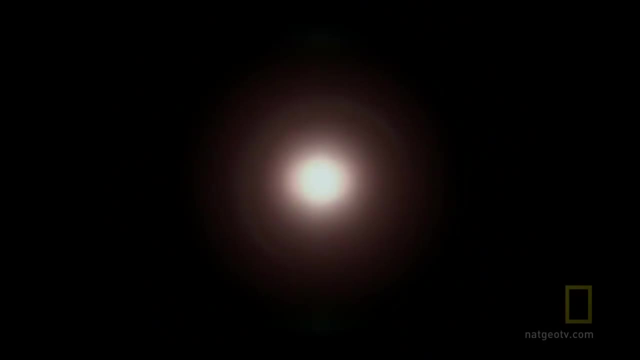 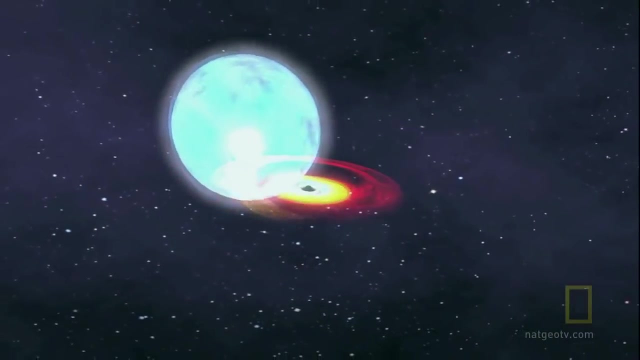 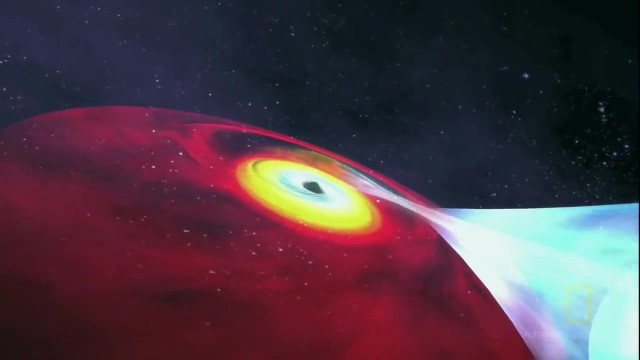 that attracts more and more matter. just like the big crunch, The gravitational pull is so powerful that anything that falls near a black hole will be forever trapped. Not even light can escape. It's a mind-boggling concept that something invisible is detectable. 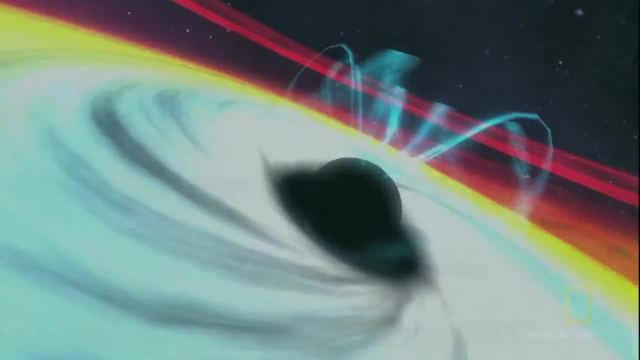 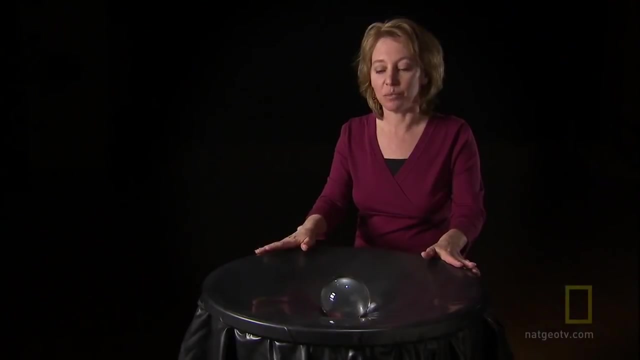 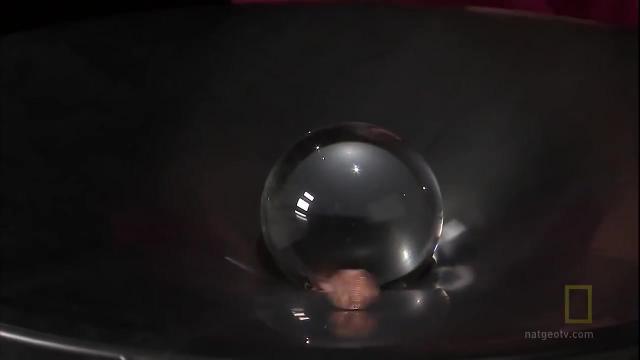 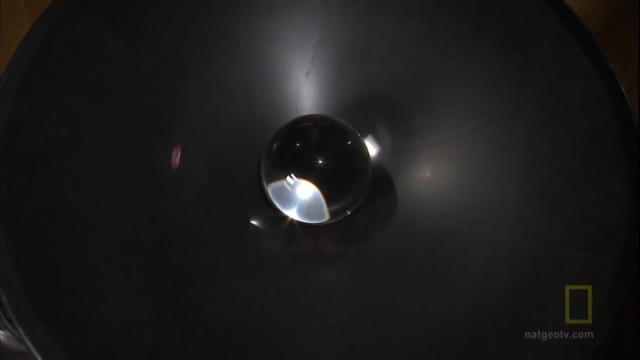 and offers a view to our ultimate fate. This black tarp represents space, And space is relatively flat, But when you put a massive object into space, it curves it. This is a penny, And notice how it comes into a really beautiful circular orbit. 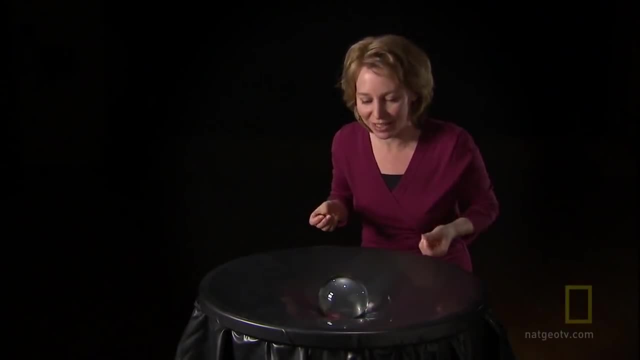 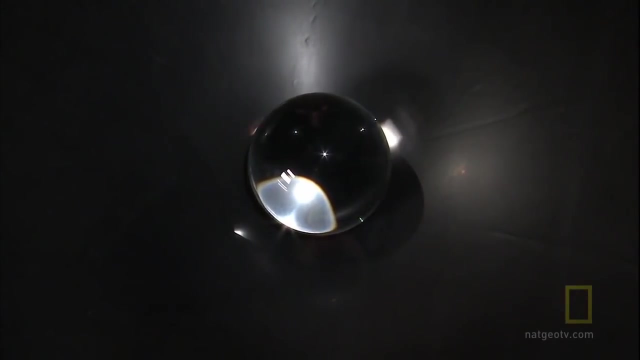 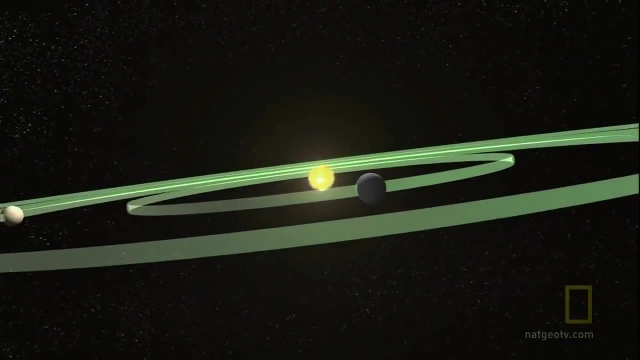 Basically, the black hole trapped it into an orbit around itself, And that orbit becomes very circular as it gets closer. And now the penny will eventually disappear. go inside the black hole. Earth's sun warps space similarly to a black hole, only it's a cosmic wimp by comparison. 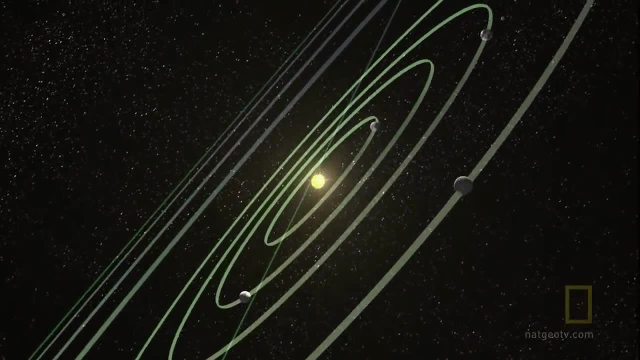 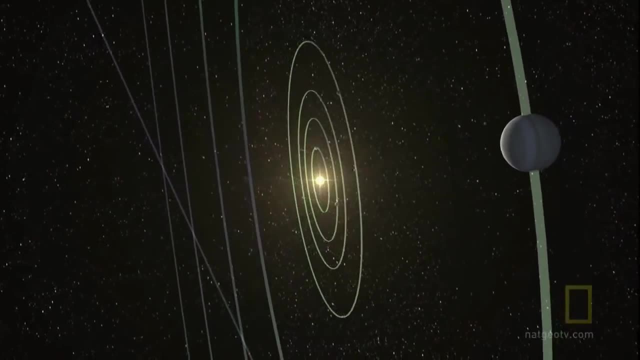 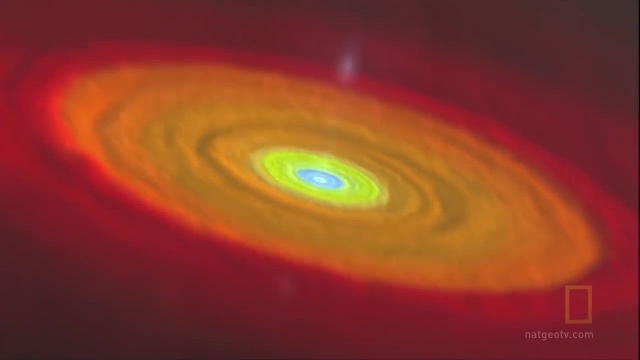 The gravitational pull of our sun is much weaker. Earth and all its nearby planets are trapped by the sun's pull, but it's so mild that it just stays in orbit without being sucked into the sun. The mass of a black hole can be a million times the mass of the sun. 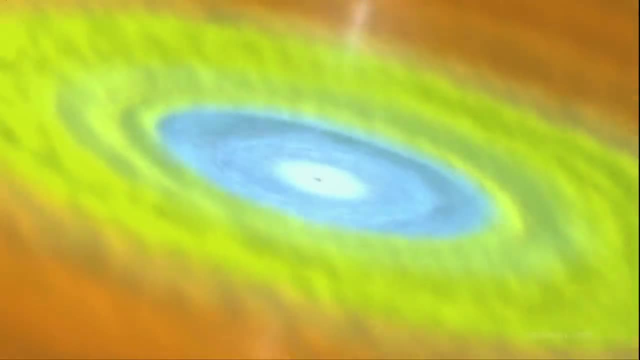 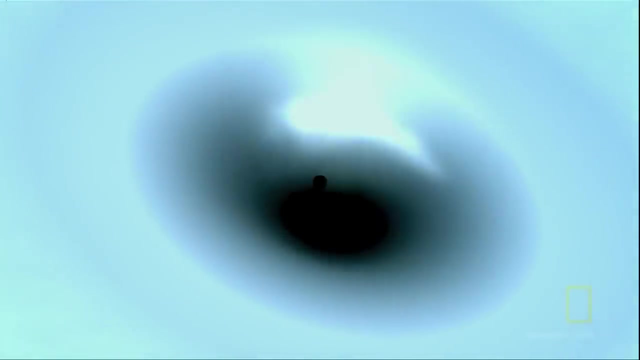 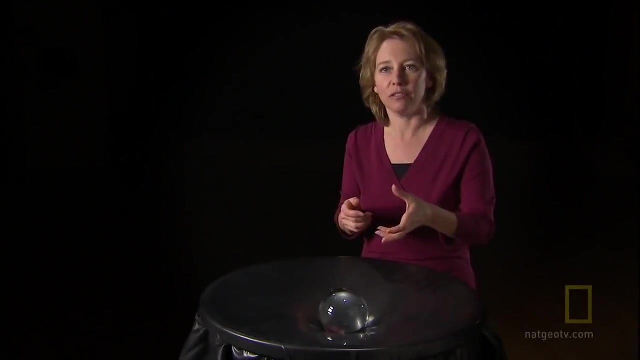 or more, causing a huge warp in the space around it that consumes everything that comes near. That black hole wraps space around itself, And so if material falls near it, it falls inside and gets trapped forever. Black holes exist in isolated areas throughout the cosmos. 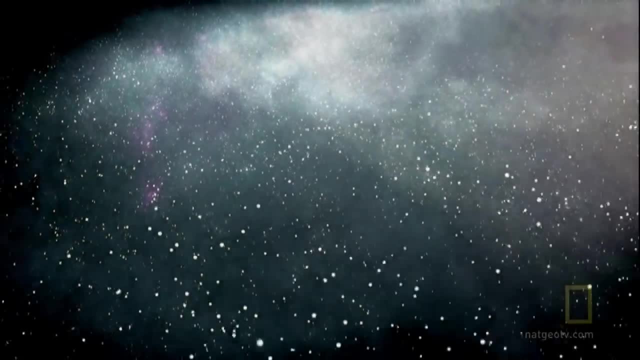 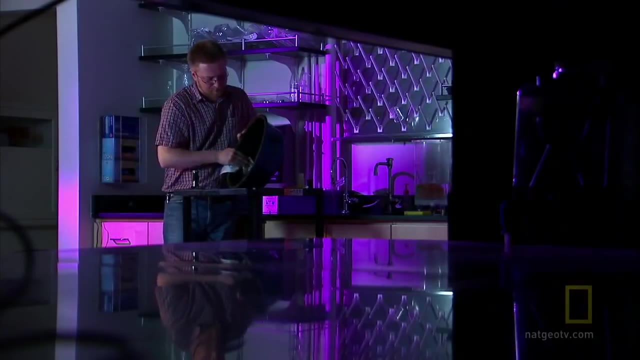 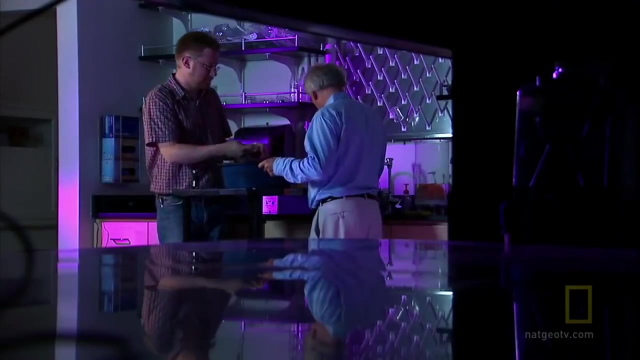 A black hole's gravitational pull is a scaled-down version of the force that could cause the universe to collapse. That force is dark matter, And dark matter is what scientists often call cosmic glue. Hi, Matthew, So let's do some cosmology here. 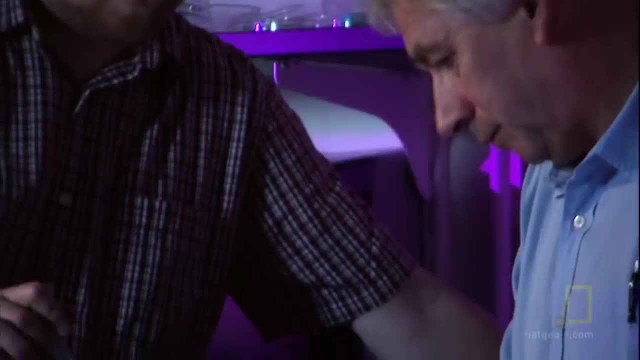 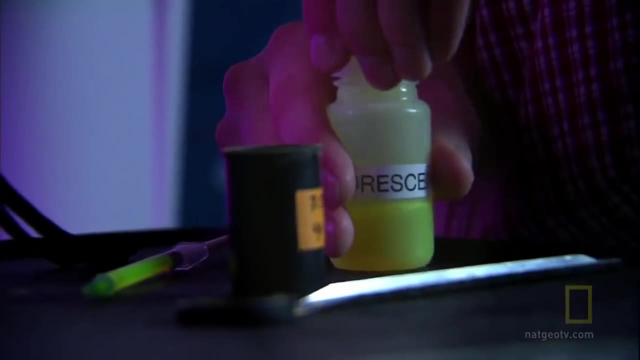 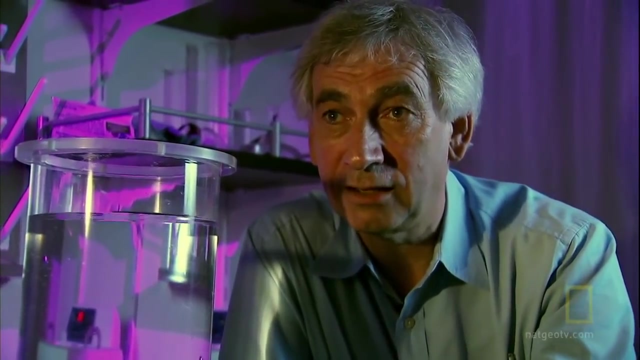 Dark matter attracts other objects via its gravitational attraction. It's a positive force. There's another force that opposes gravity, And that is dark energy. Dark energy- we don't really understand what it is, but it's a negative repulsing effect that pushes galaxies away from each other. 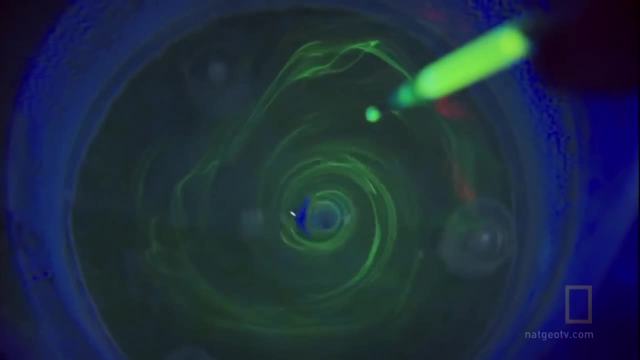 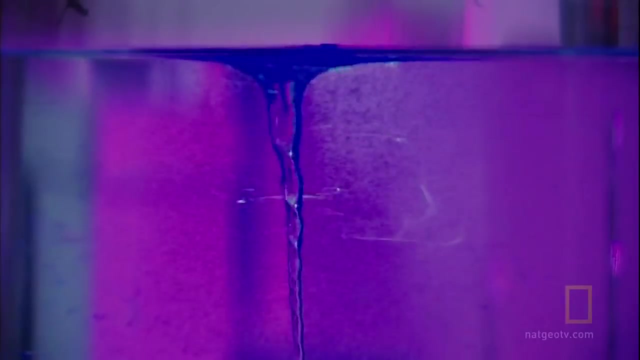 The whirlpool in Richard Ellis's demonstration represents the gravitational force of dark matter. The green dye coming out of the syringe shows how the stuff of the universe collapses under the force of dark matter. The presence of dark matter is the gravitational force of dark matter. 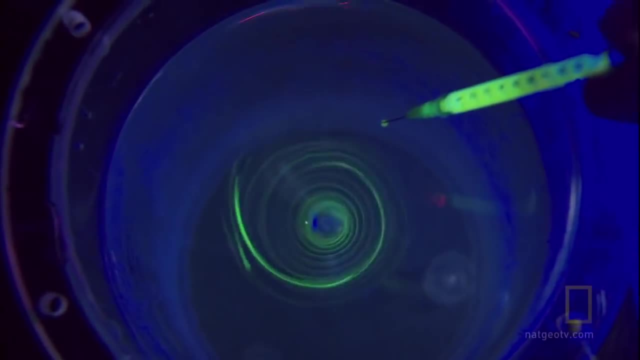 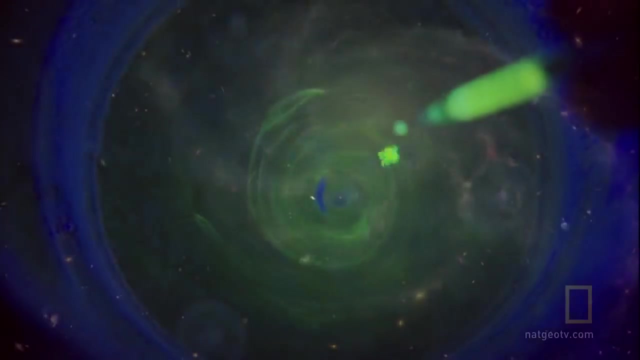 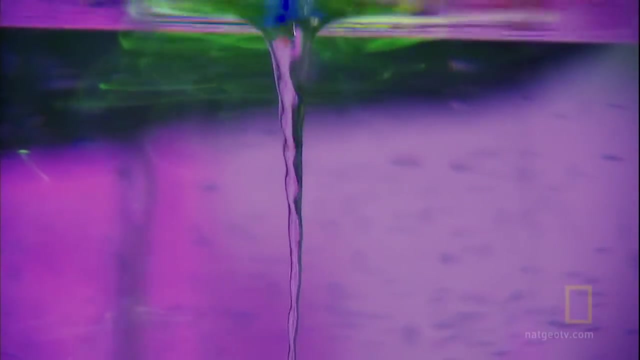 The presence of dark matter acts as the focus for the gas in the universe, bringing structure together. This is how the Milky Way developed as the universe expanded, Little things merging into big things. The positive, constructive force of gravity. Now if this was the only force in the universe. 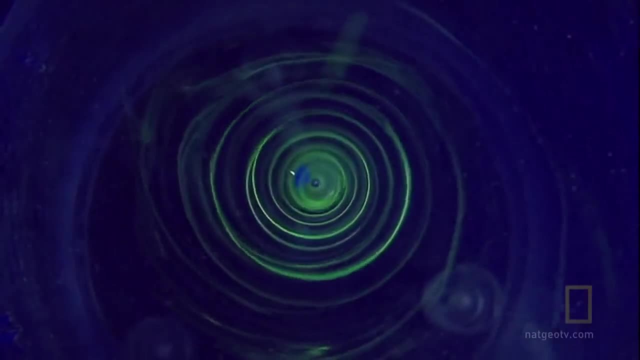 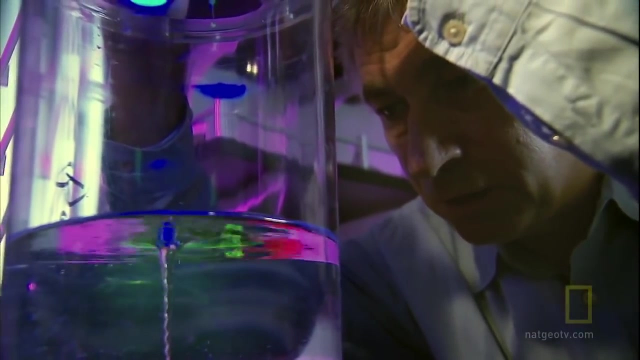 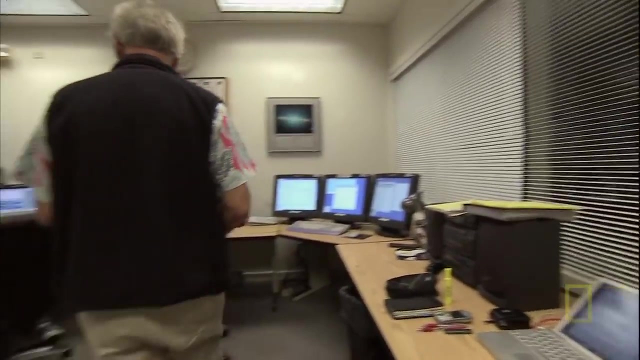 the universe would stop expanding at some point in the future and eventually the universe would start collapsing. Gravity would eventually halt the expansion, bringing it back together in a big crunch. Yet the universe continues to expand and isn't showing any signs of collapsing. 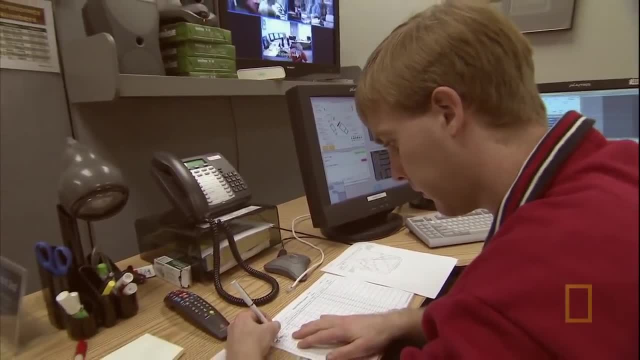 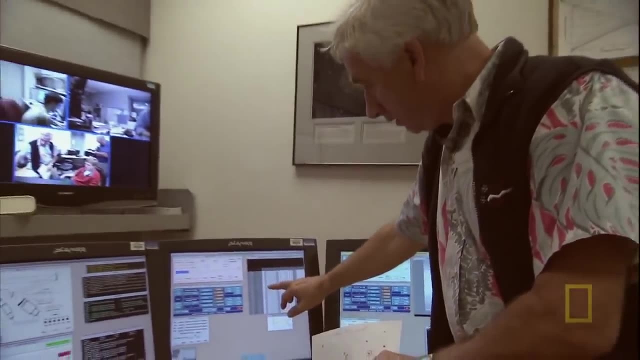 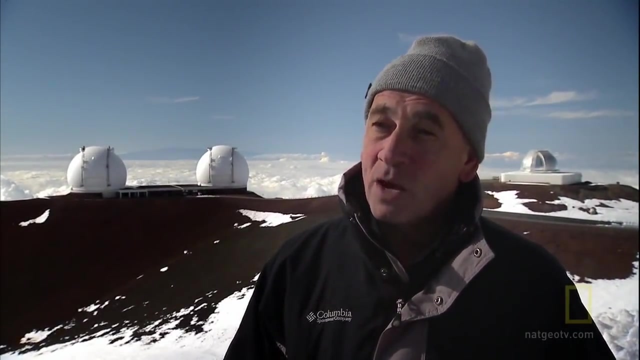 This suggests the opposing force of dark energy could be stronger than dark matter, But it will take scientific detective work to find out. They look to one of the most violent forces in the universe for clues. We're studying exploding stars to try to understand if they can tell us the rate at which the universe is expanding. 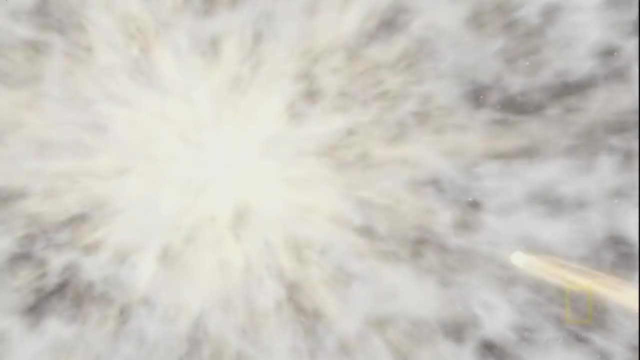 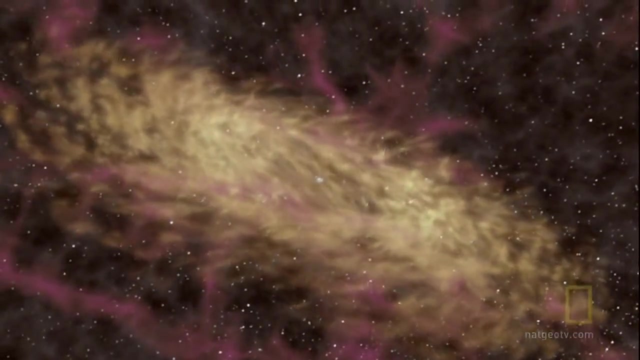 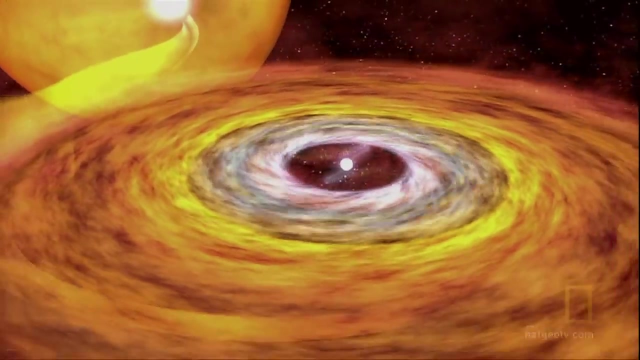 These are explosions at the end of the lives of stars. not unlike our sun, The fuel that these stars have in their centers is spent. The star collapses, the outer part expands and the star becomes something called a white dwarf. White dwarf stars sometimes have other stars orbiting nearby. 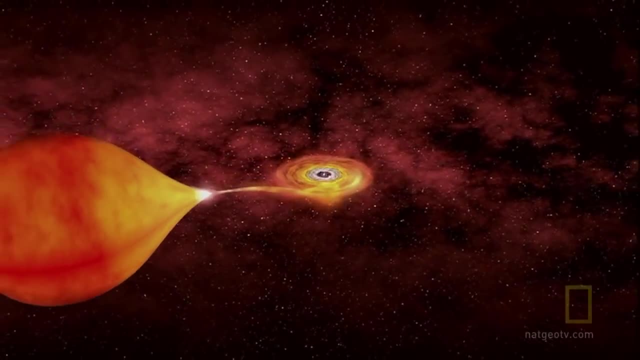 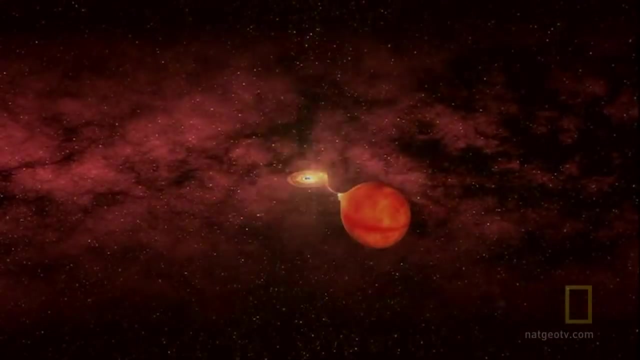 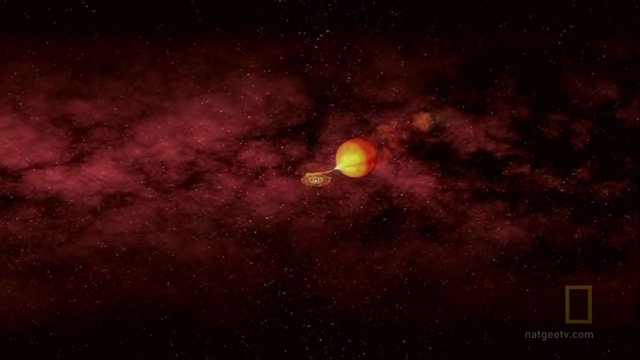 a companion star. A massive explosion could happen if the companion star's debris falls onto the white dwarf, causing a spectacular fireworks display in the cosmos. Scientists consider exploding stars or supernovae, like in these images captured by the Hubble telescope. 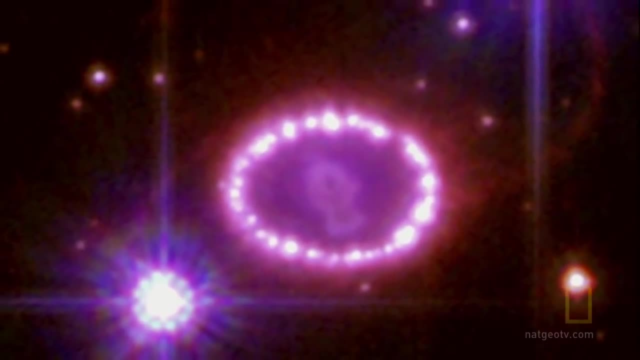 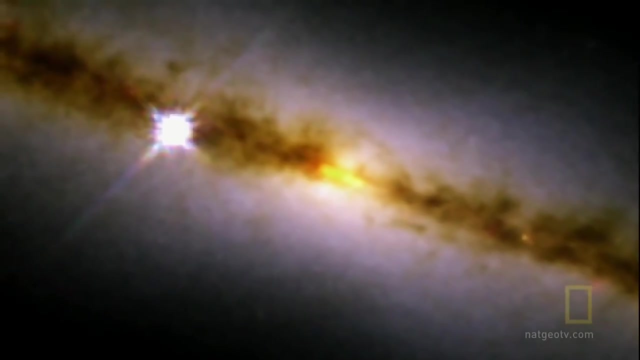 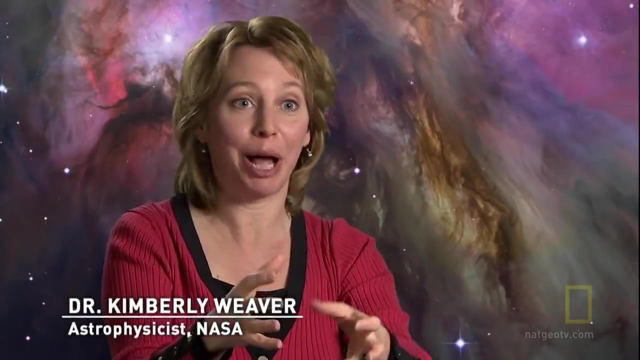 to be reliable telltales of how fast the universe expands. Their brief and bright explosions allow scientists to track the universe's expansion and give them a way to measure its speed. Essentially, they are white dwarf stars that become nuclear bombs. They explode with a certain brightness. and a certain length of time. It takes a certain amount of time for that brightness to dissipate. They are essentially standard candles. Any one of these will look the same no matter where it is in the universe. Astronomers measure the distance and speed. 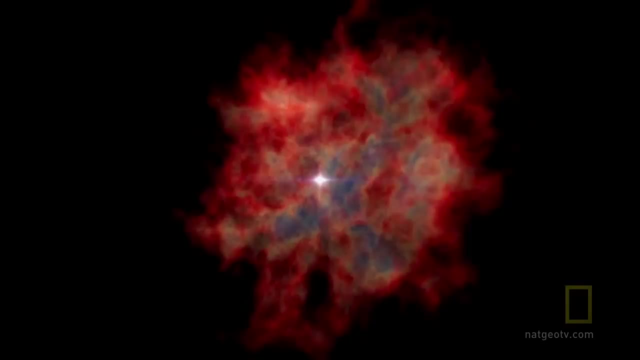 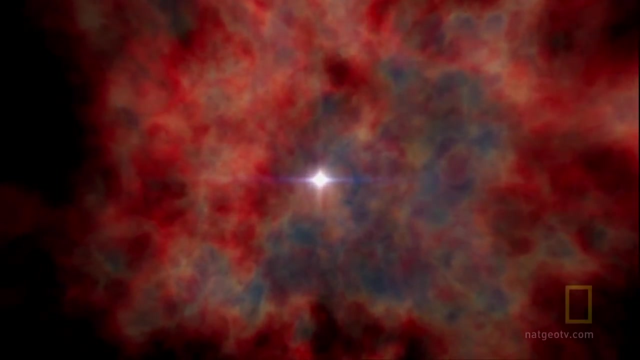 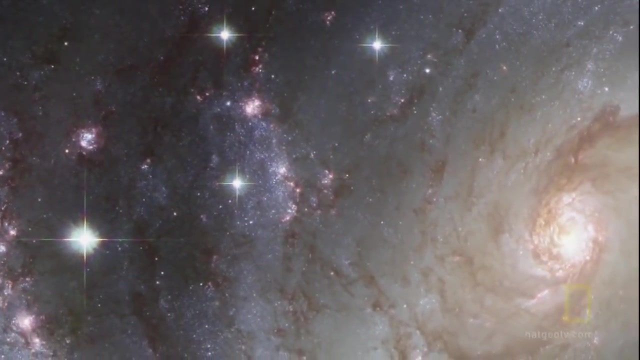 of these exploding stars by measuring the amount of red light they emit. The faster the star moves away from us, the redder its light appears. The expansion rate of galaxies containing stars like supernovae can then be used to interpret how the rest of the universe is moving outward. 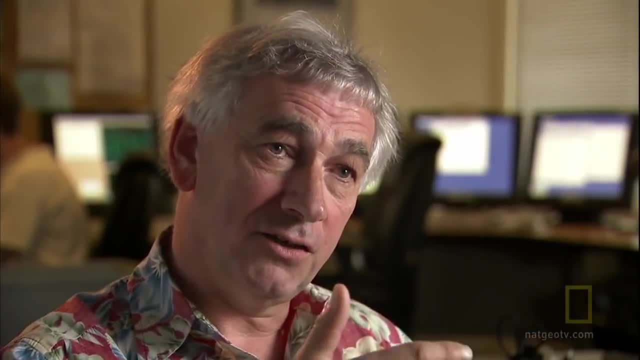 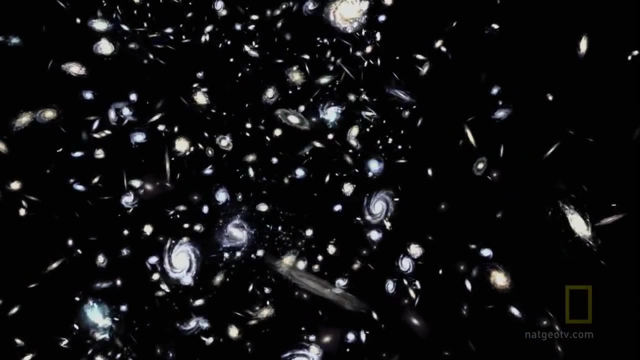 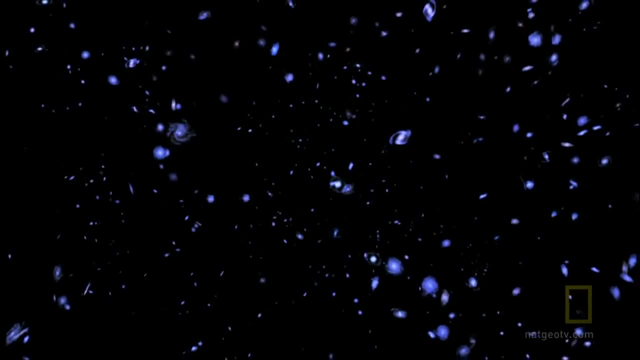 We know this because we can compare the velocities of galaxies with their distances. These are the clues that lead astronomers to answer just how soon the universe will reverse direction and come back together in a big crunch. Or this information might lead to an entirely different conclusion. 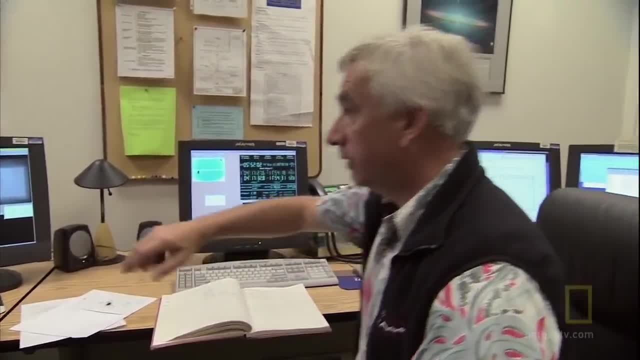 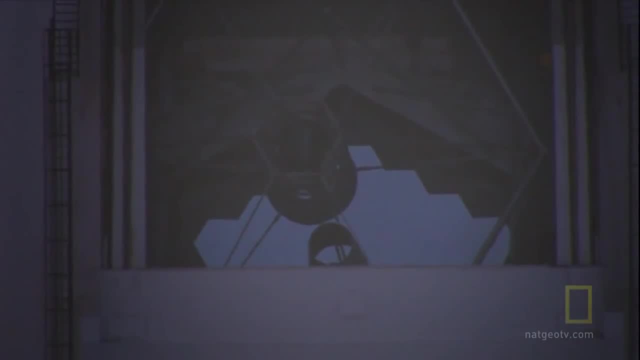 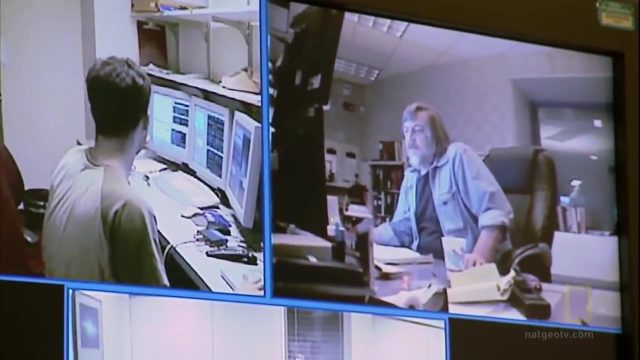 Dr Ellis is looking at clues at the Keck Observatory in Hawaii. While the telescope is on the top of a huge volcano, he's in a viewing room on another part of the island. Hey, emission lines, Johann, In the red, in the red side, I think. 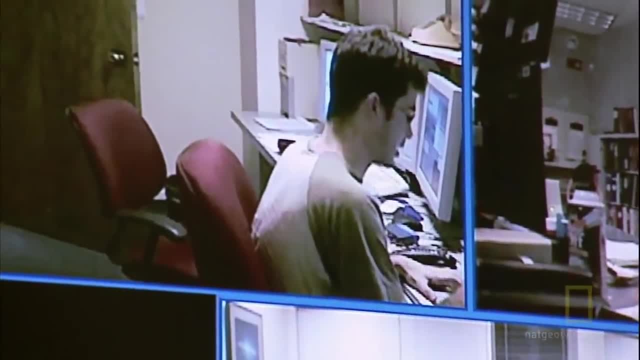 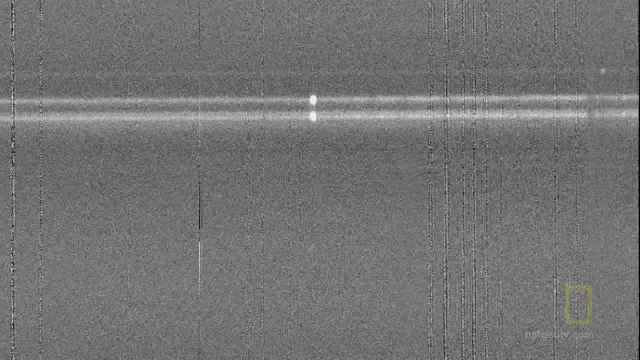 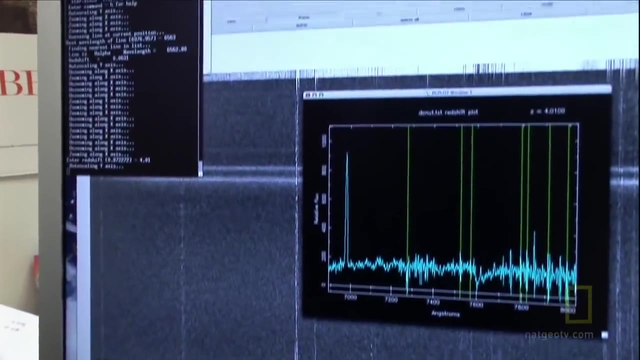 At the same time, Johann Richard is at the California Institute of Technology in Pasadena, California, evaluating the light from a distant galaxy that the Keck telescope captured in Hawaii. He's looking to see if any of the known elements coming from the galaxy are in the red spectrum. 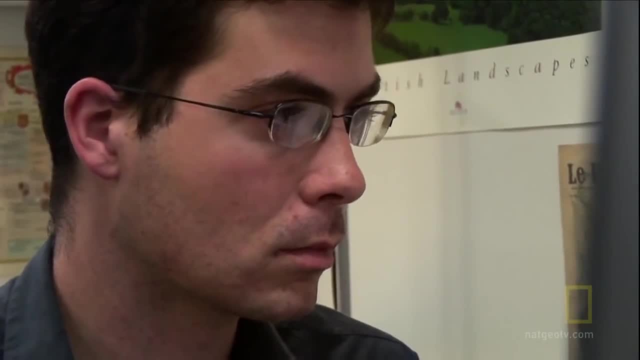 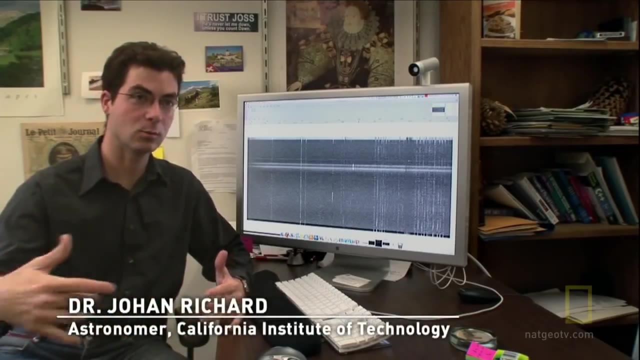 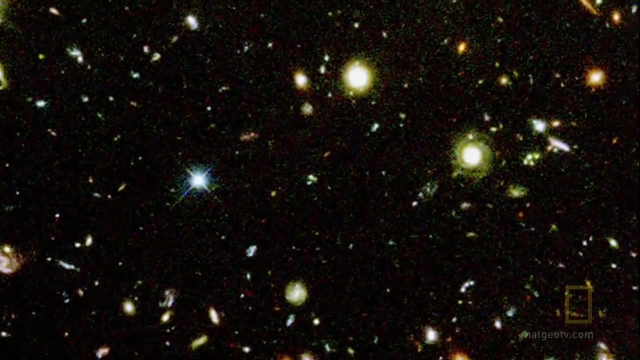 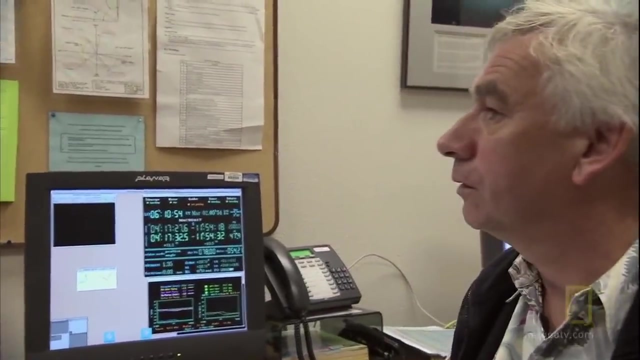 and moving farther away. We can interpret that as a velocity, as how much the galaxy is moving away from us. We can really interpret how the entire universe is behaving, is expanding. Interpreting redshift is the cornerstone of the quest to pin down the fate of the universe. 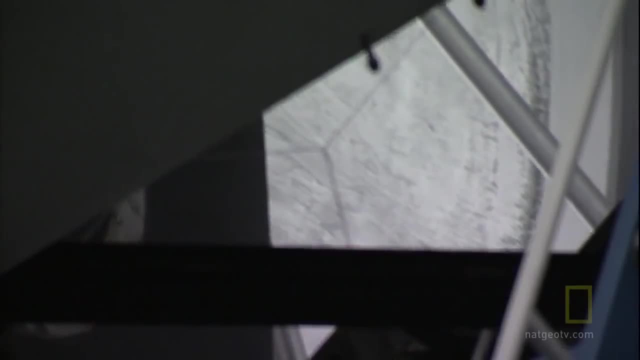 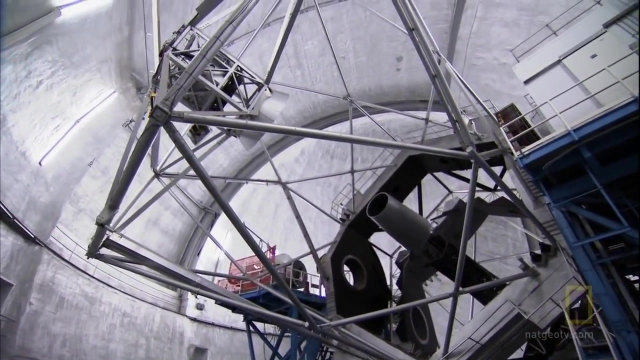 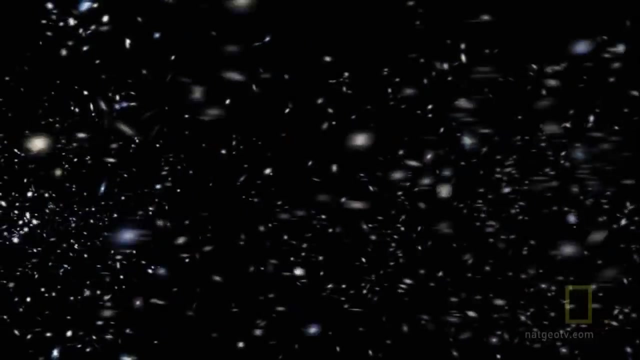 Clearer pictures of the universe that have only been possible in recent years have led cosmologists to conclude that the redshift of distant galaxies is greater than predicted. This is startling. Not only is the universe expanding, it's speeding up. Nothing in the observable cosmos 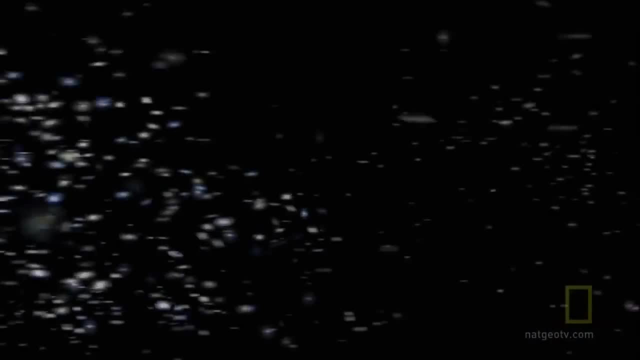 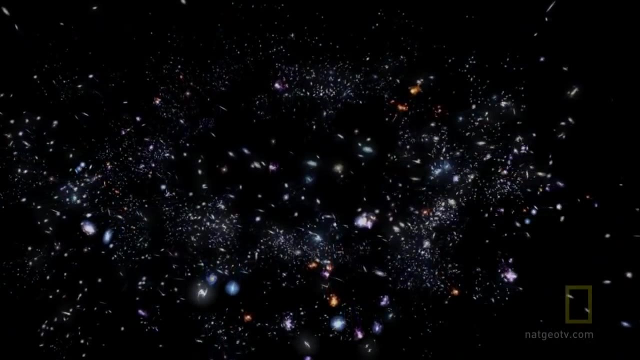 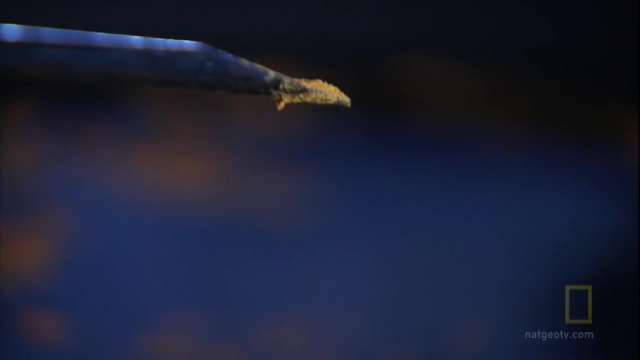 could account for an accelerating universe, and yet the data seem irrefutable. This has to mean that an invisible force is working against gravity. Cosmologists have come up with a name: dark energy. So when the universe was young, gravity was the most dominant force. 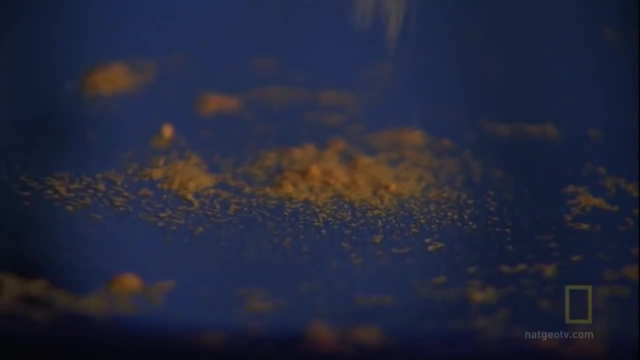 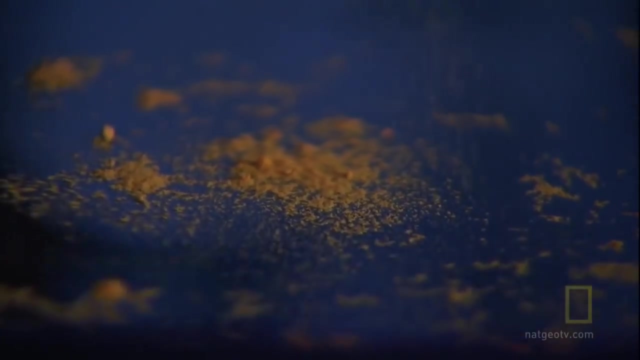 And so what we see here is galaxies, as particles on the surface of the water are bound together by gravity, And at a point about 7 billion years ago, dark energy and gravity are pretty well in balance, But the universe continues to expand. the density goes down. 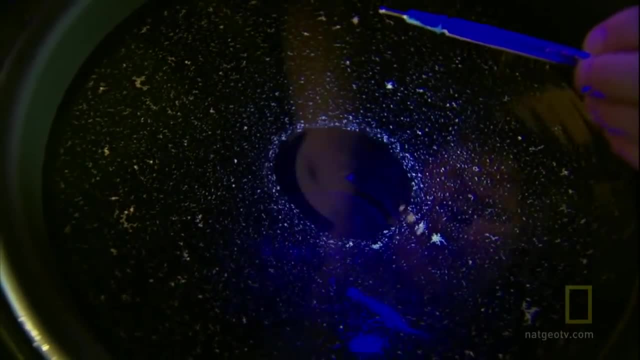 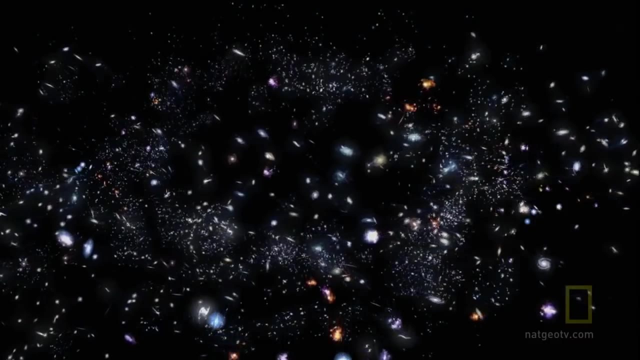 and so dark energy starts to take over And lo and behold, the universe starts to accelerate. So dark energy is now the dominant property of space. So the universe started out with a certain amount of energy, and we know we're trying to understand. 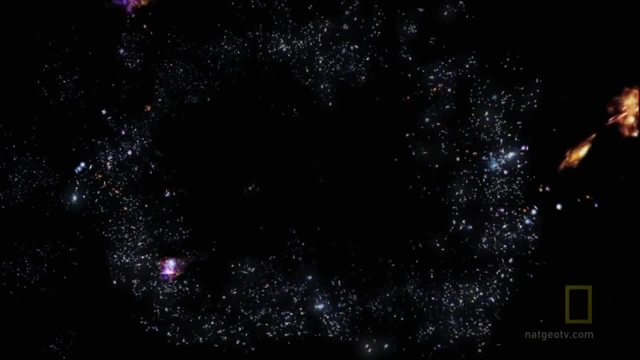 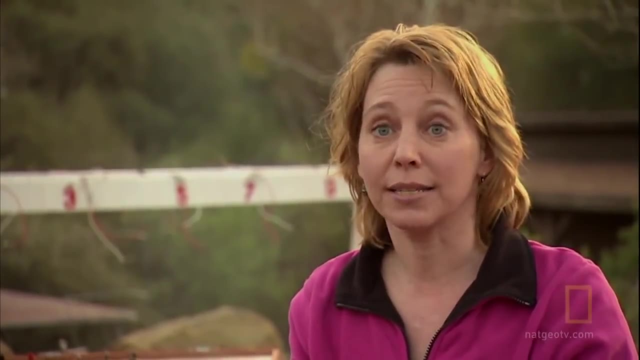 how much energy there is and we know the universe is expanding as it moves outward with time. We also know now that the universe's expansion is accelerating and we don't know: is that acceleration going to slow down or not? We're still trying to understand that. 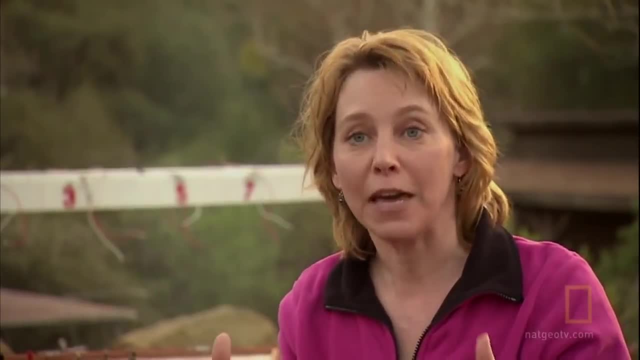 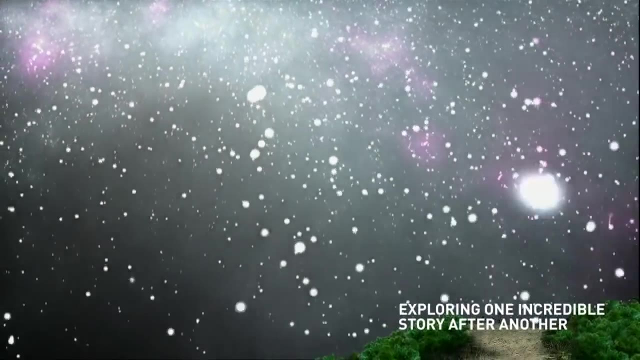 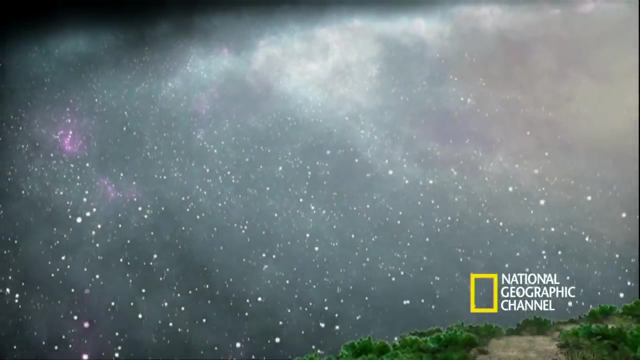 So, in understanding what's going to happen to the fate of the universe, we have to know how much energy is there, how much matter is there? The history of the universe is really a battle between dark matter and dark energy. These two forces are in opposition. 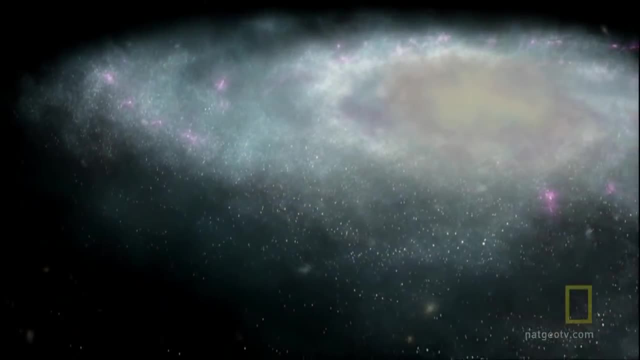 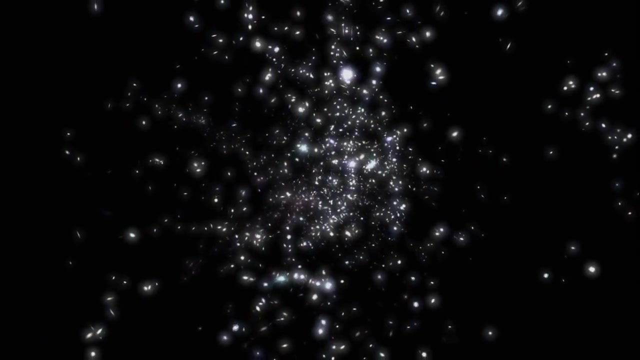 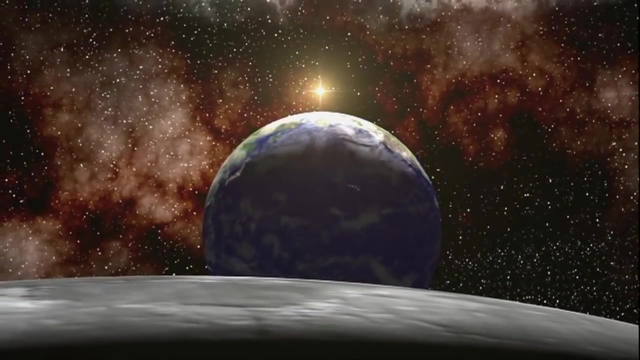 and so both the history of the universe and its ultimate fate is really the competition between these two forces. The Big Crunch theory was a result of scientists interpreting that dark matter is the dominant force, But astronomers now suspect that dark energy might be much stronger. 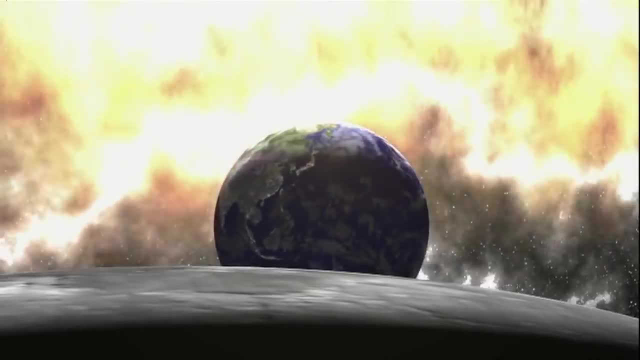 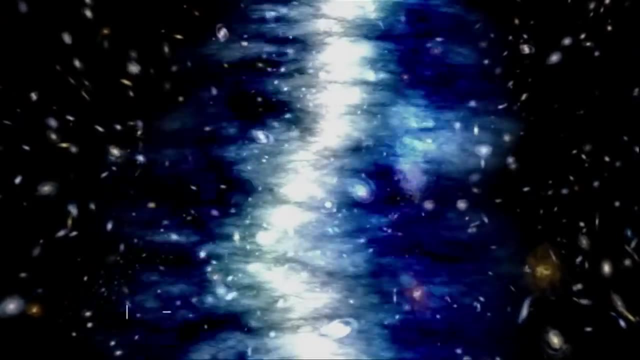 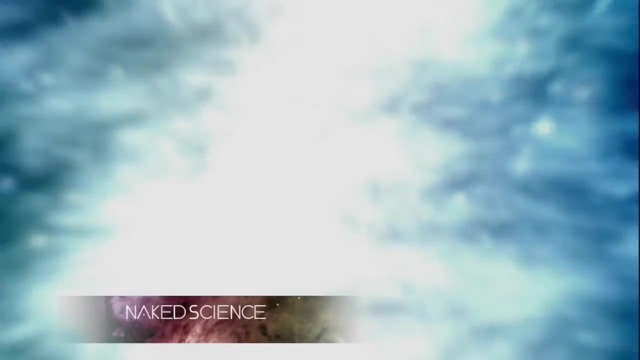 If so, the end could be dramatic and violent. It pulls apart solar systems, it pulls apart stars, and eventually it grows so strong that it pulls apart matter itself, breaks bonds, pulls apart atoms and reduces everything to fundamental particles, and that's the end of the universe. 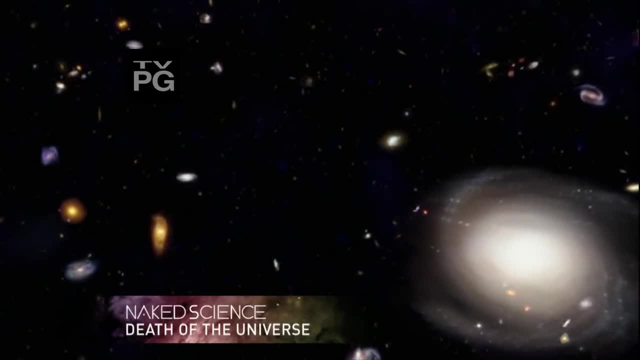 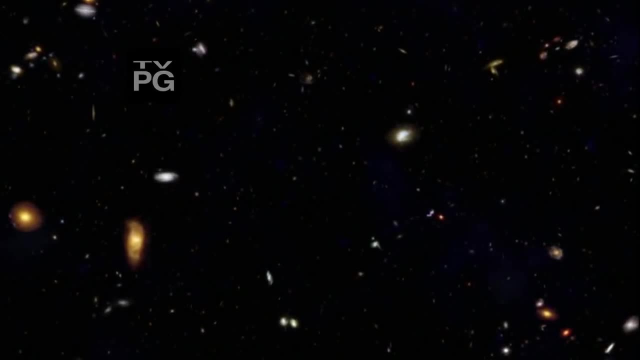 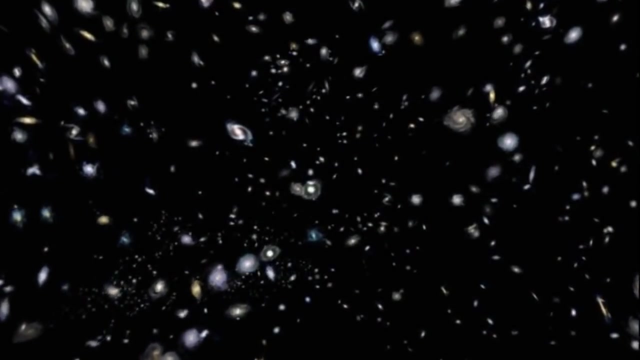 The battle between dark matter, the force that holds the universe together, and dark energy, the force seeking to tear it apart, has set the universe on a path of destruction. If dark matter is the victor, the universe might collapse If dark energy rules the cosmos. 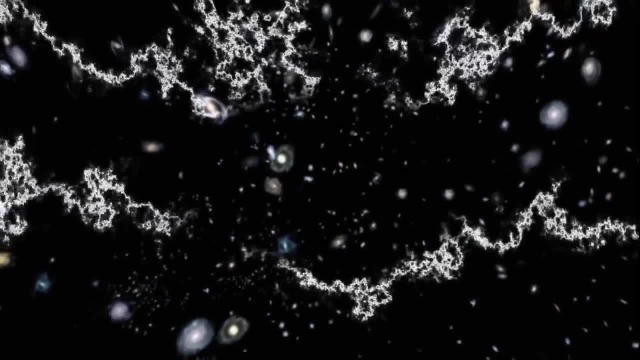 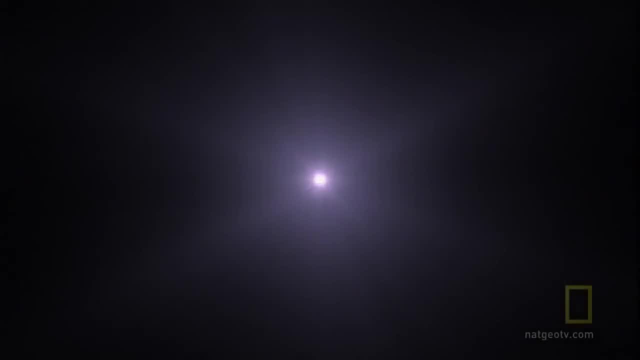 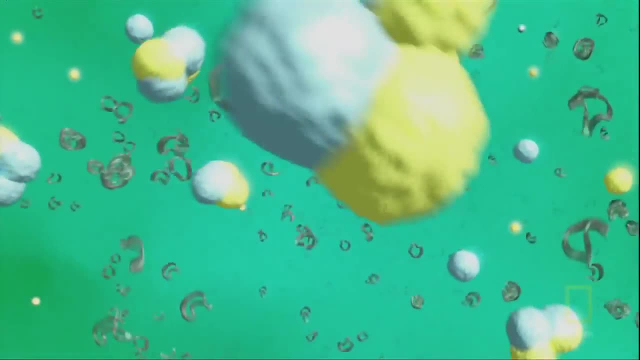 it could rip to shreds. The expansion grows so strong that it tears up the entire universe. It'll be a strange twist of fate. Dark energy, the force that propelled matter to form a magnificent universe, continues to push it outward and drives it to its demise. 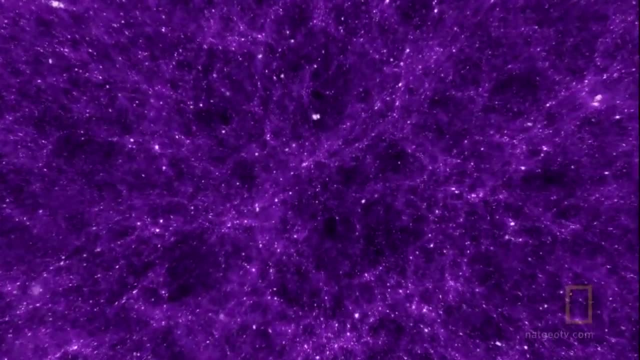 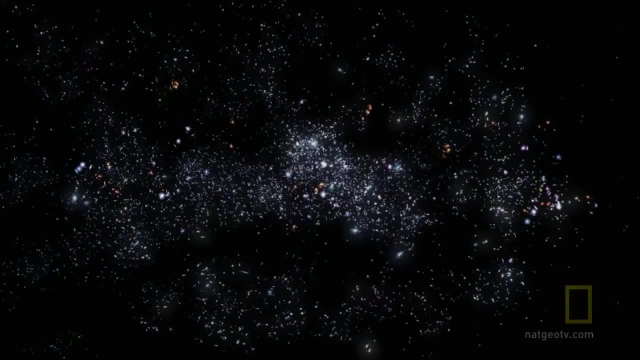 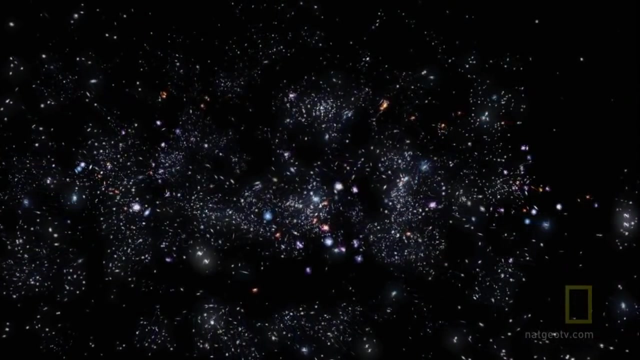 To find out if dark energy is in fact winning the battle, scientists will first need to know how fast the universe is actually expanding. The most remarkable feature of the universe is that it's expanding. Every galaxy is moving away from every other galaxy. When you look out into the night sky. 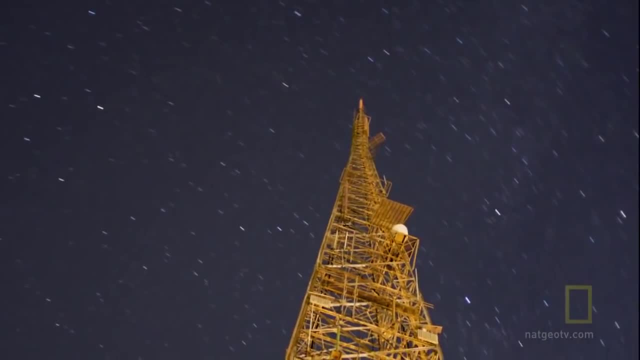 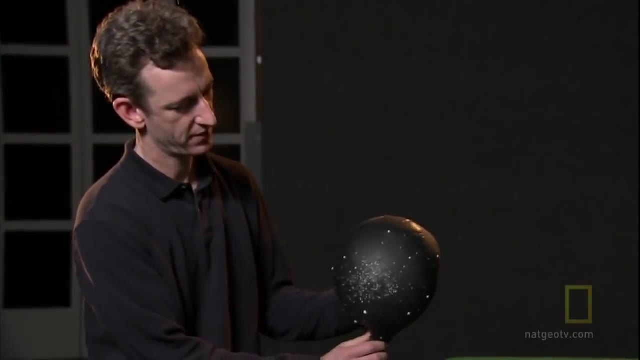 you see distant stars, galaxies, clusters of galaxies, the observable telescopes, and they're all moving away from us. We can illustrate that with this balloon. As we expand it, we see that every dot drawn on this black balloon like the night sky. 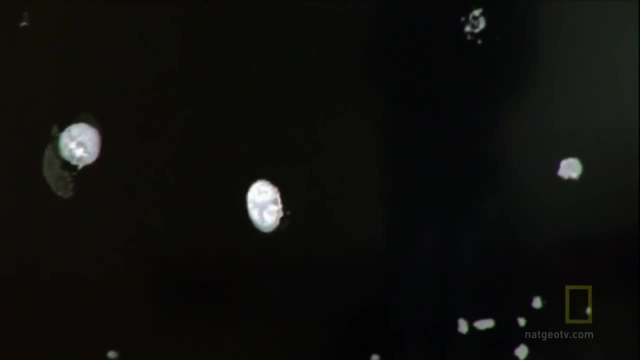 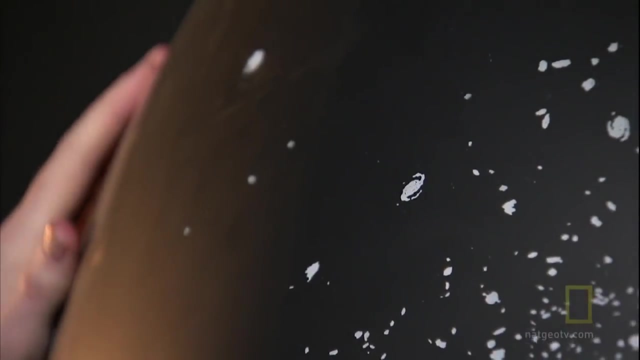 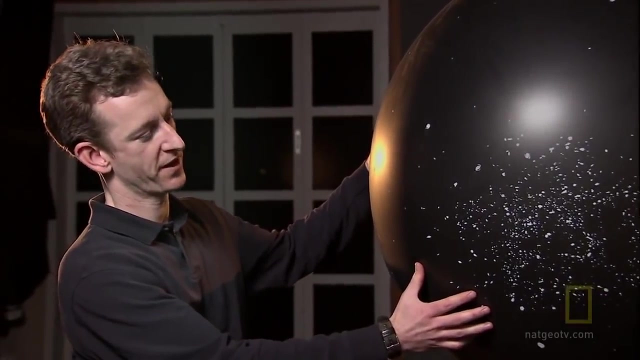 is moving away from every other dot. But there is something else that we know about the universe, something else that we know about the expansion. That is that the expansion is getting faster, The universe is accelerating, The size of the universe is getting bigger. 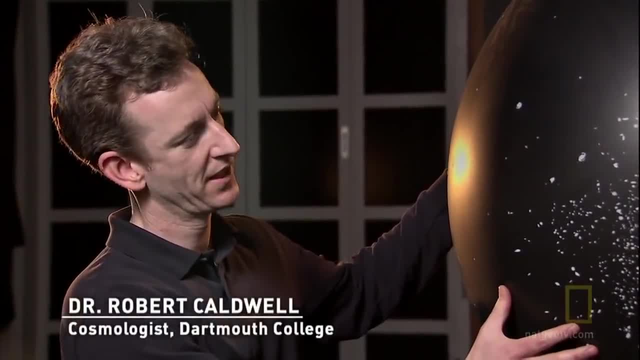 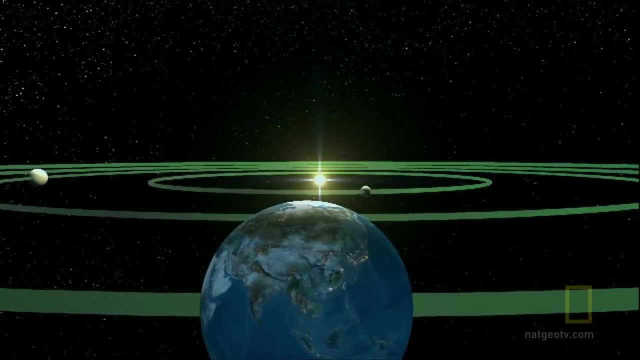 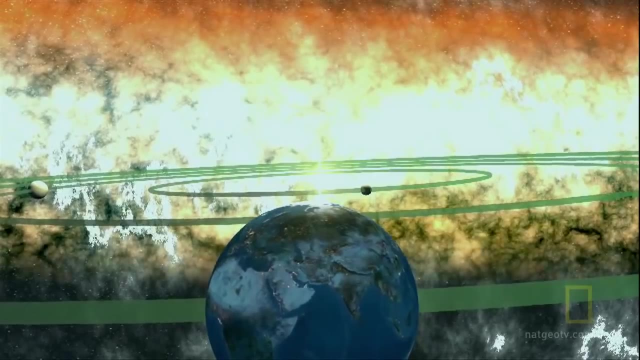 at a faster and faster rate, And we don't know exactly how fast it's accelerating. but if it's accelerating fast enough, then something really dramatic could happen: The universe could end up tearing itself apart in a big rip. This is perfect. 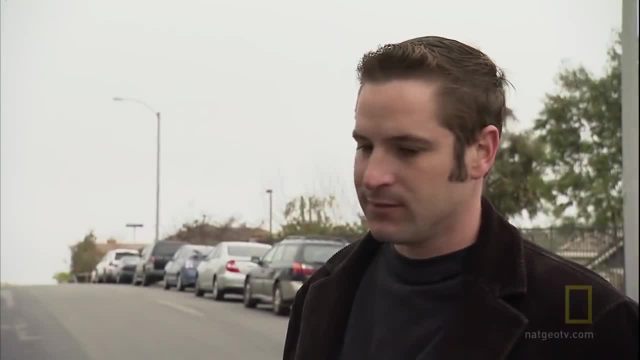 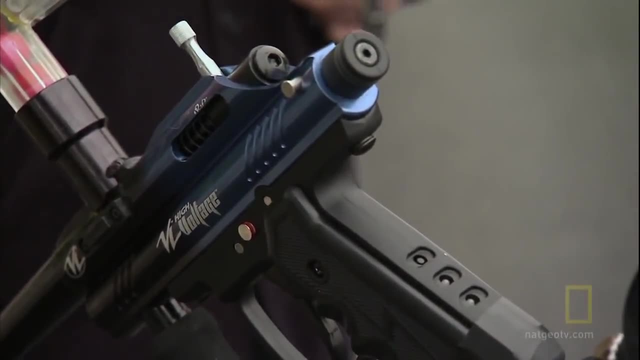 This is great that you rigged this up. So this is. this is a giant version of the demo that I do in class. Dr Robert Caldwell attempts an earthbound experiment: to show how dark energy affects the acceleration of the universe. He uses a paintball gun. 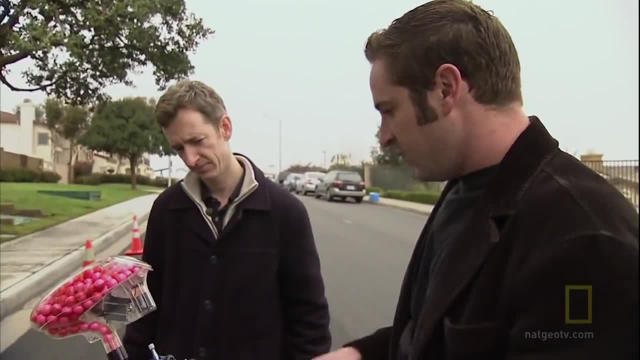 mounted on a truck? Yeah, and basically I mean we could adjust the angle in any way that you want it. What do you think about this? Yeah, I think, down at the ground, you know, is the best that we can mark. 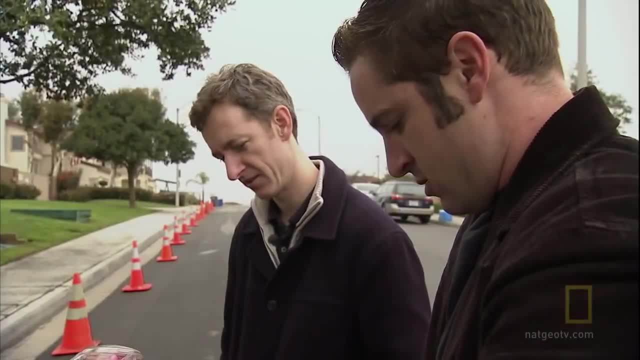 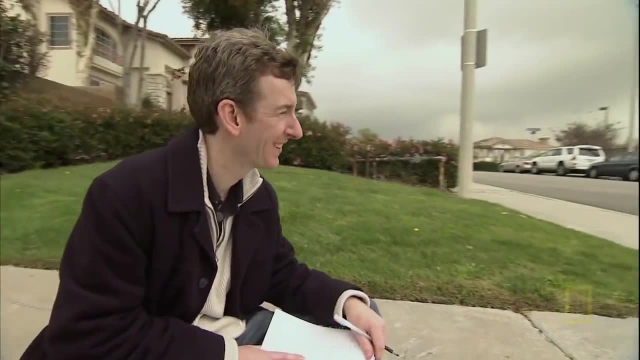 each time the gun fires. How's that? That'll be good? All right, let's try that. He sends the truck coasting down an incline. Earth's gravity pulls the vehicle downhill, which is similar to how dark energy propels the universe outward. 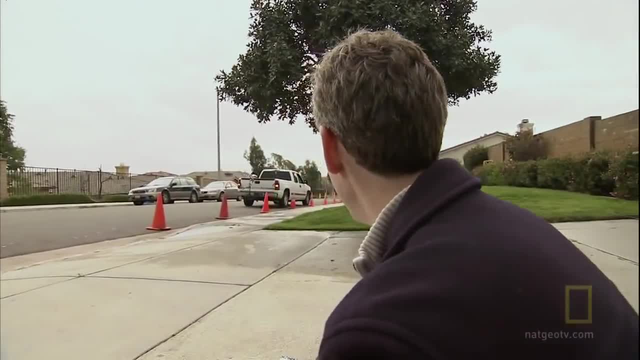 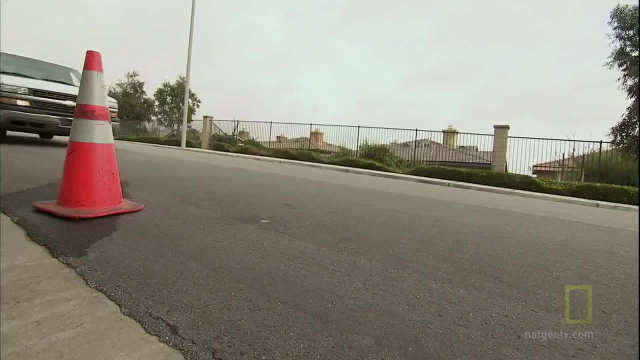 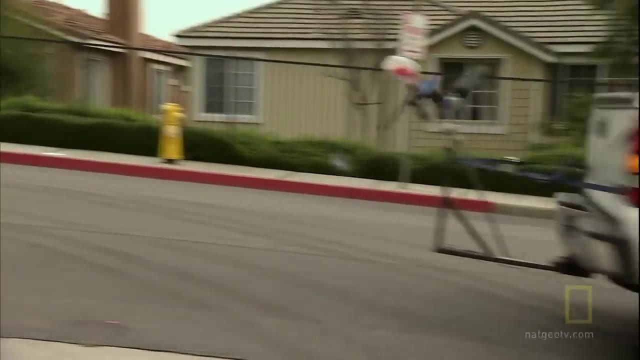 causing it to expand. Gravity pulls the truck forward at an increasing speed. The gun fires paint at the ground at regular one-second intervals. Caldwell measures the distance between the paint dots to calculate just how fast the truck was accelerating. He'll use the data from this experiment. 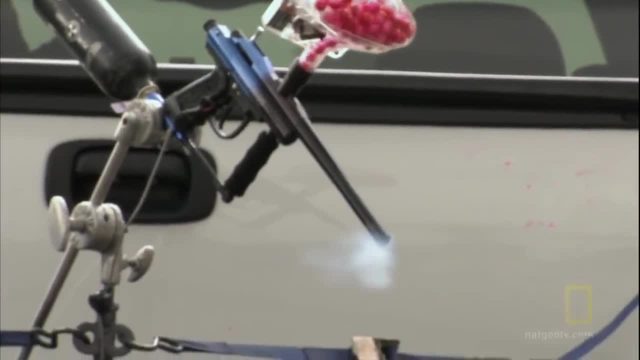 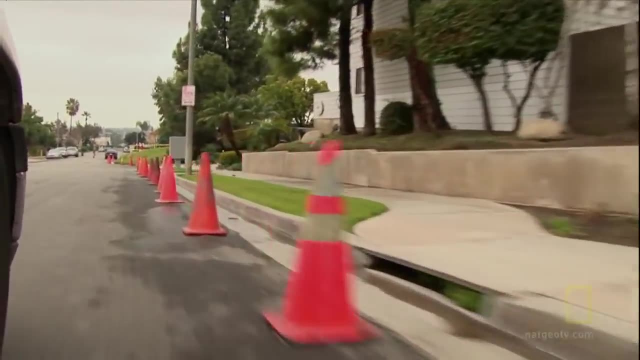 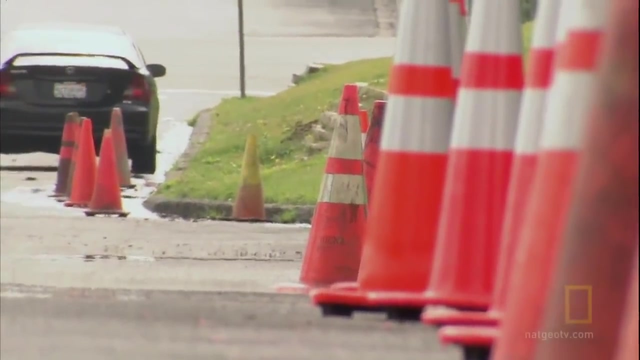 to see how gravity's force compares to dark energy's force in the cosmos. We started thinking about the Big Rip when it was discovered that the expansion of the universe was accelerating. The degree of acceleration is not known and it's the subject of a lot of effort. 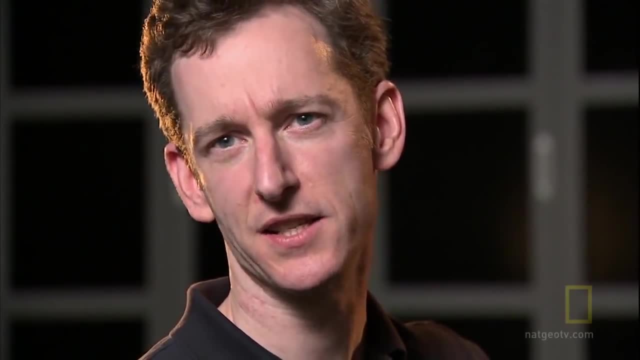 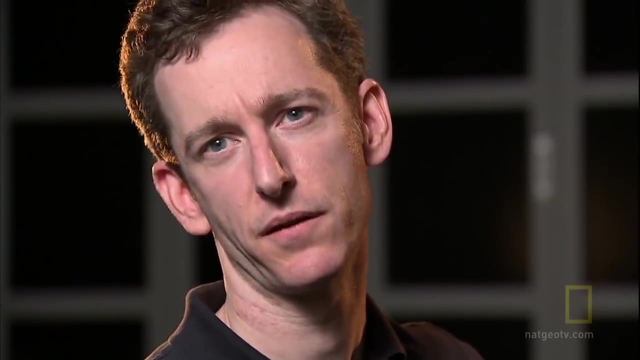 by astronomers today to try and figure out exactly how fast the expansion is growing. what is the past evolution of the universe in detail and, if we can glean from that, what is the future evolution of the universe? It's not known exactly how fast it's accelerating. 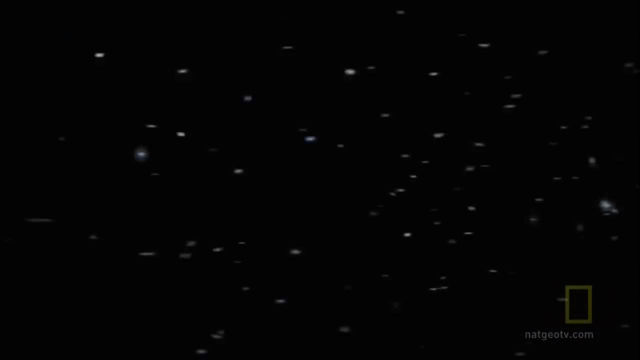 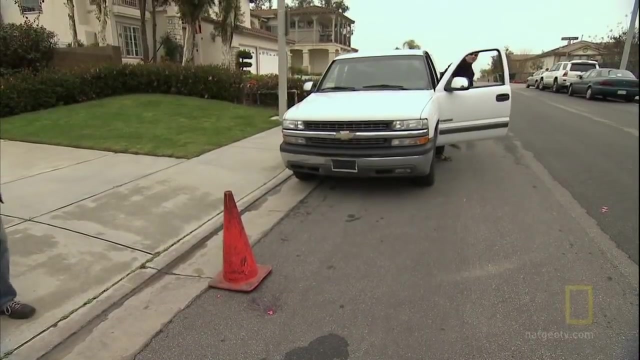 There's some evidence that the acceleration is beyond a certain threshold, and beyond that threshold there's a runaway effect that could take place and it would rip apart the universe. Good luck Fantastic. I think we've got some good data, Excellent. 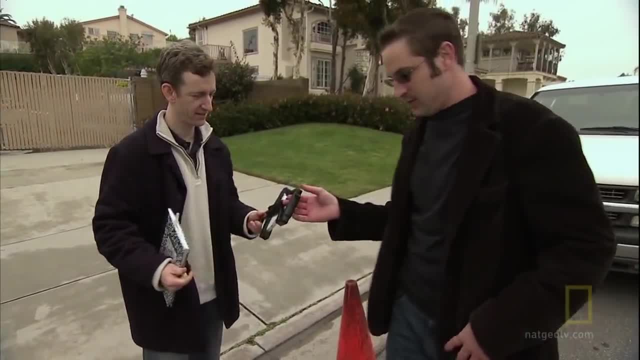 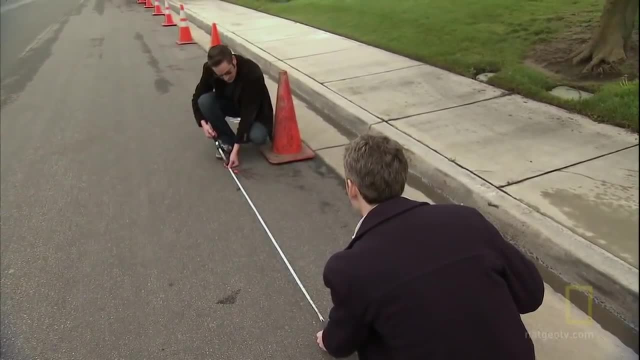 How do we measure this? Great, I'll give you that end. All right, I'll take this Five feet eight, Eight and a half inches. The point of the paintball experiment is to find parallels between the truck propelled by the invisible force. 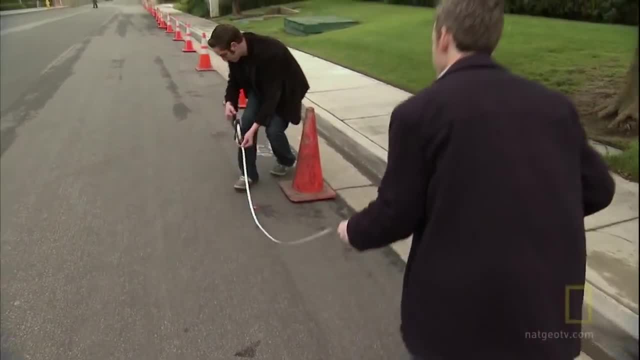 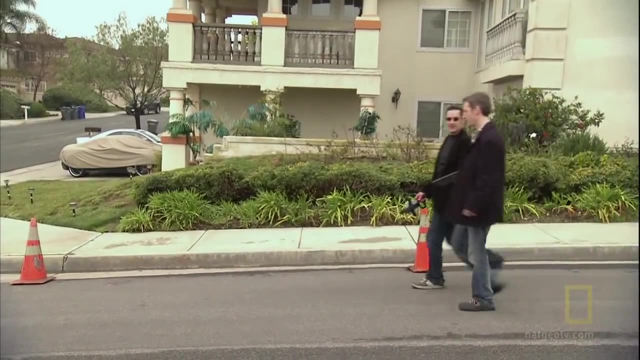 of gravity and the accelerating universe Got it. I'm glad we got the long tape measure because it's really growing pretty fast. the interval Within a few measurements, the distance between the paint spots, increases by nearly seven times If the truck were in space. 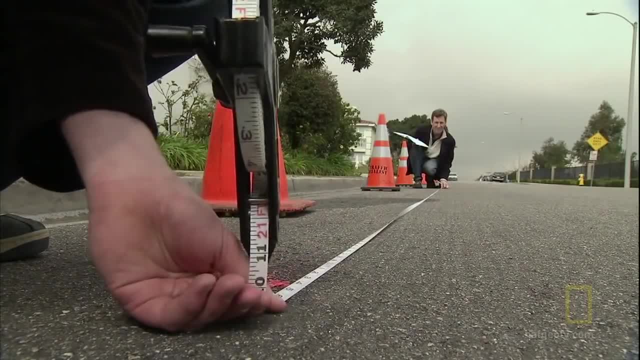 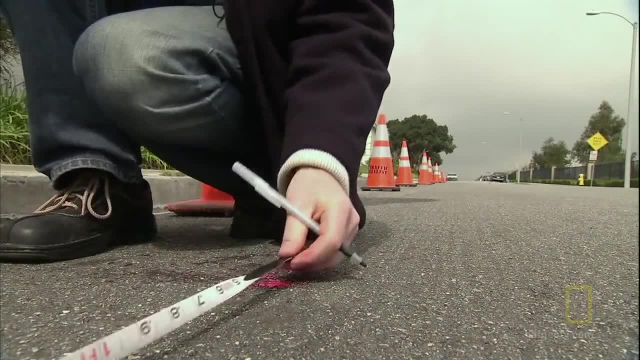 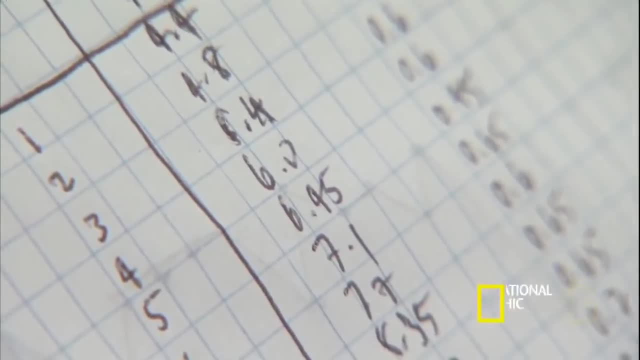 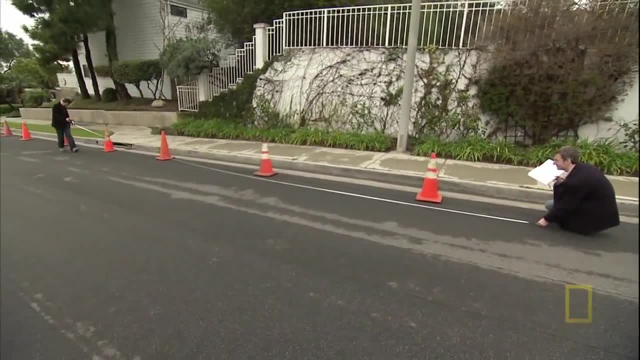 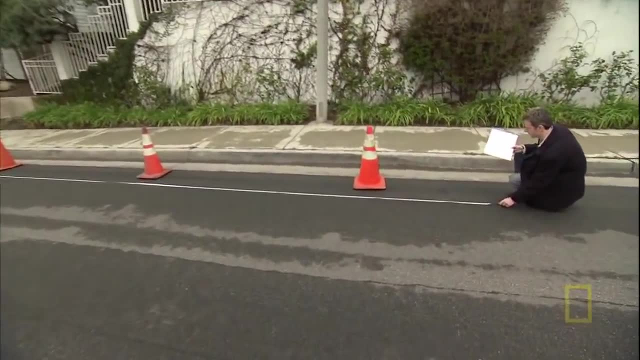 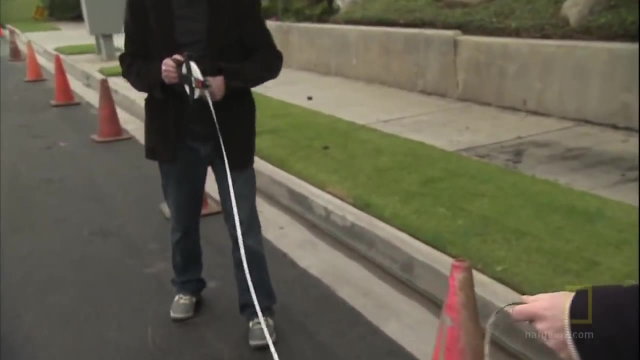 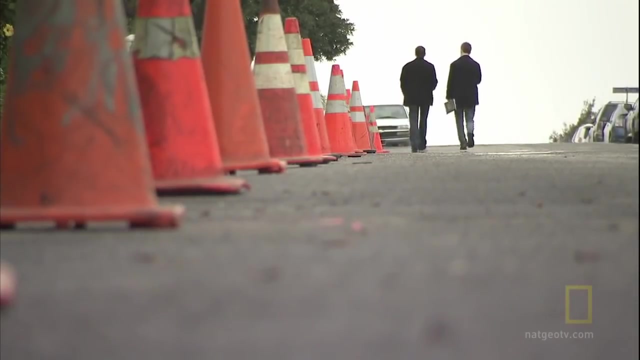 We've got 42 and a half feet 42,- all right, 0.5.. The question for Robert Caldwell is whether the same kind of expansion and acceleration are happening on a cosmic scale. What's the capsule made of? Is it plastic or something? 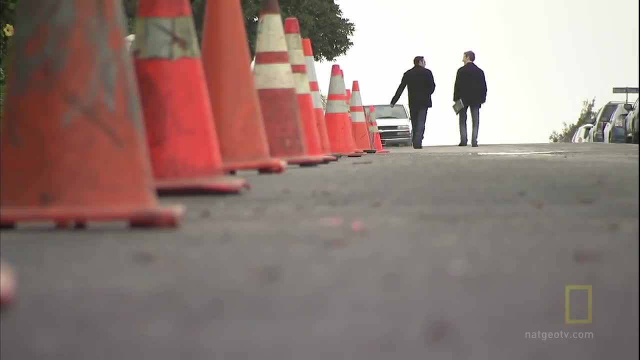 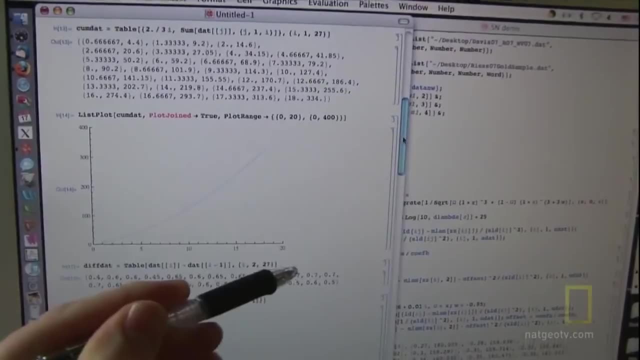 It's gelatin. It's all biodegradable. You could actually eat them if you wanted to. This right here is the data that I took with Eric: The cumulative distance traveled by the car as a function of time. and that's beautiful. It's this nice parabolic shape. 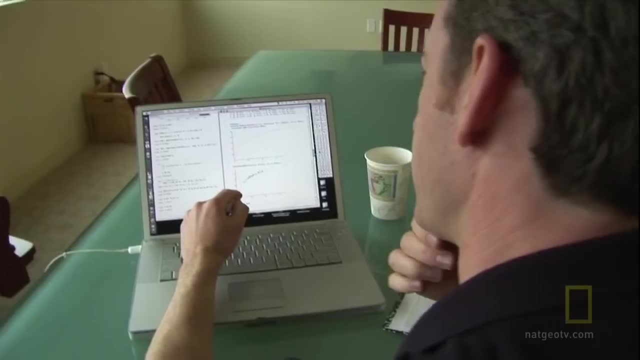 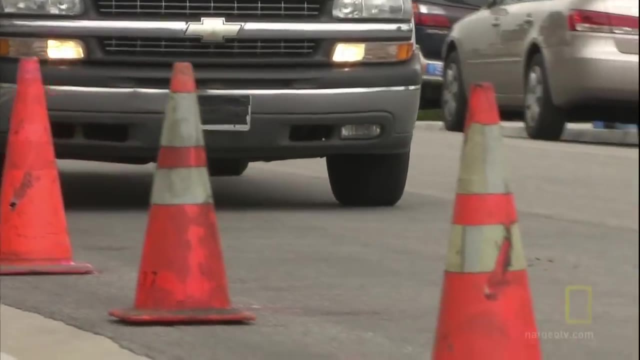 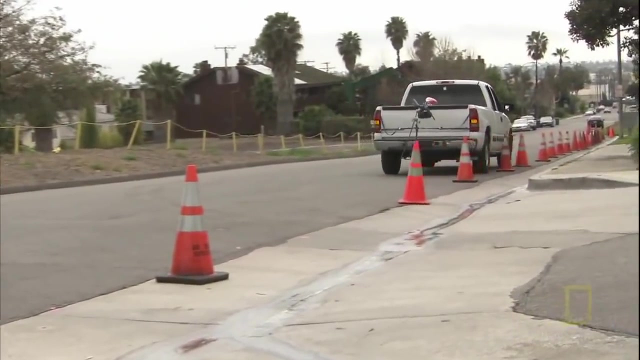 That's exactly what you expect for an accelerating body. Now over here I've got another calculation going on where I'm working out the acceleration of the universe. Robert Caldwell's calculation shows that forces on Earth are similar to forces in space. This demonstration then gives a sense of the dramatic rate of expansion. 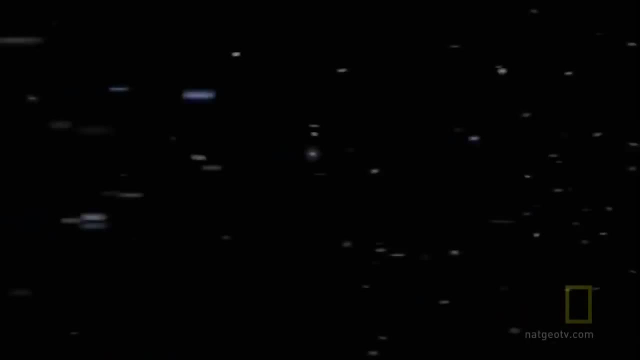 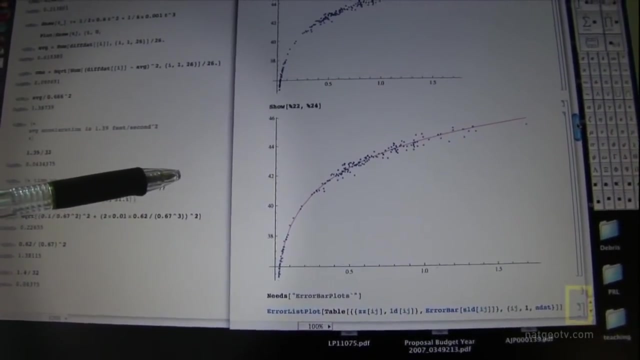 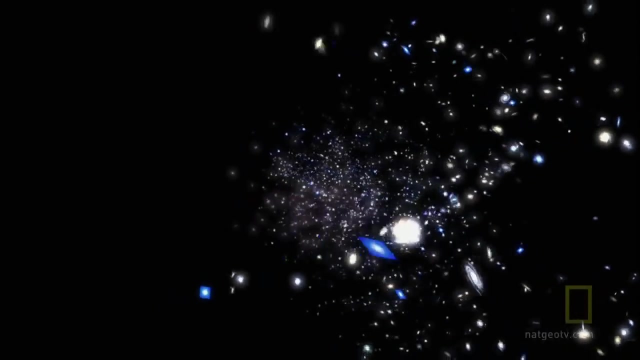 that appears to be happening in the cosmos. By eye, it might be difficult to appreciate how good a fit it is, but I can tell you that the weight of the statistics indicates that an accelerating universe is a very good fit to this data If, like the truck, the universe is continually accelerating. 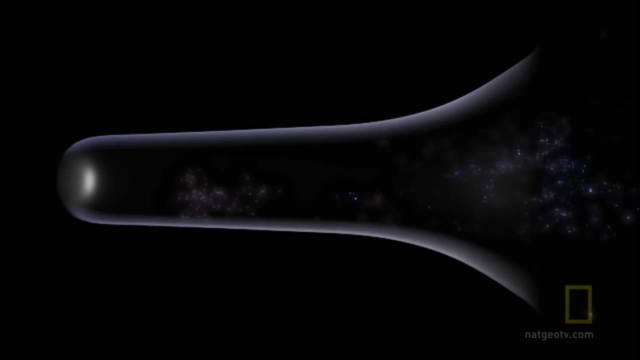 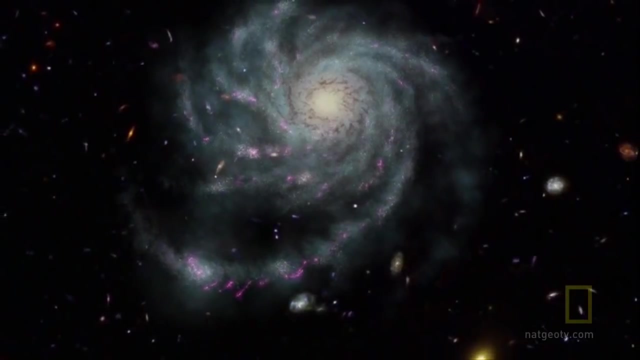 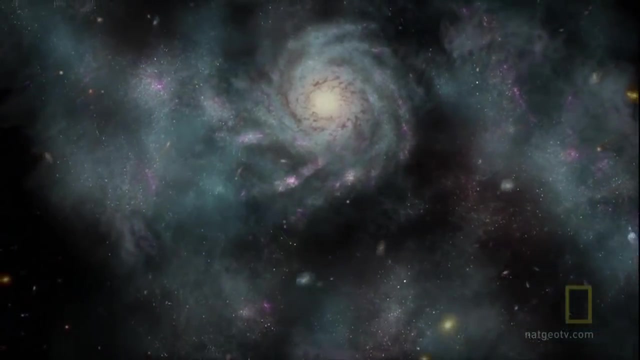 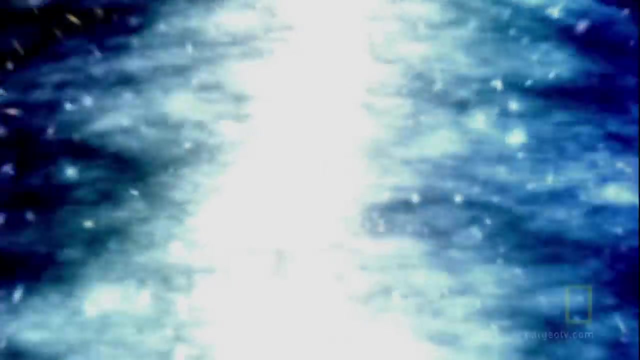 then, billions of years from now, the universe might tear itself apart. All the distant stars and galaxies will be pulled away from each other. They'll be pulled away from us, But, moreover, we won't have time to grow cold and lonely. It'll actually be pretty exciting and dramatic and violent. 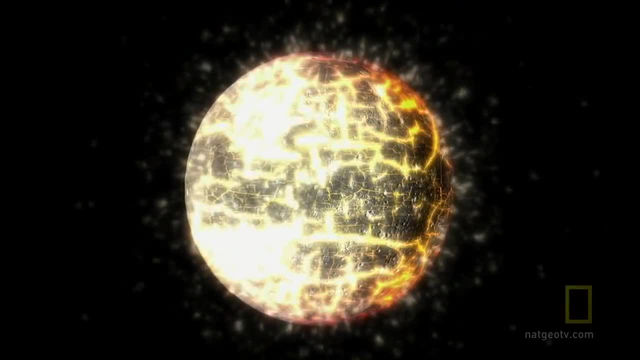 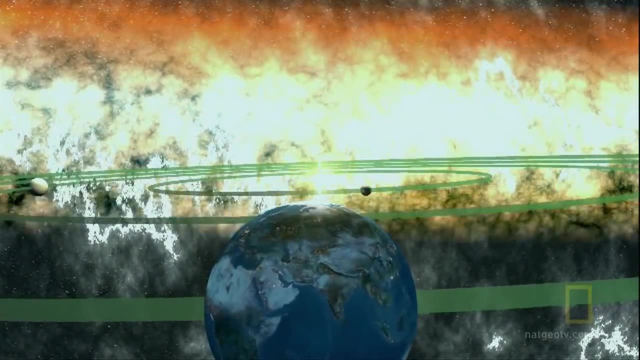 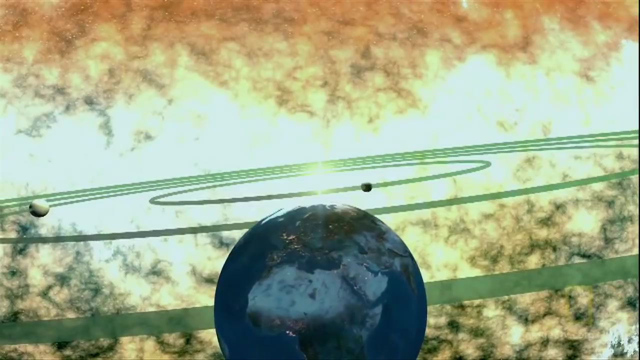 Stars are ripped apart, planets are ripped apart and even atoms are torn apart. before the universe ends, It wouldn't happen for at least 50 billion years, but still it's an interesting fate for the universe. What would atoms ripping apart look like? 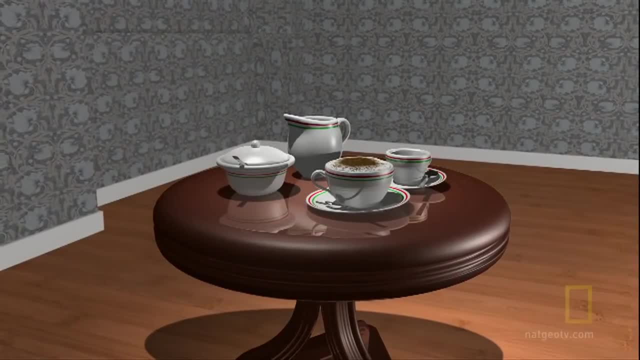 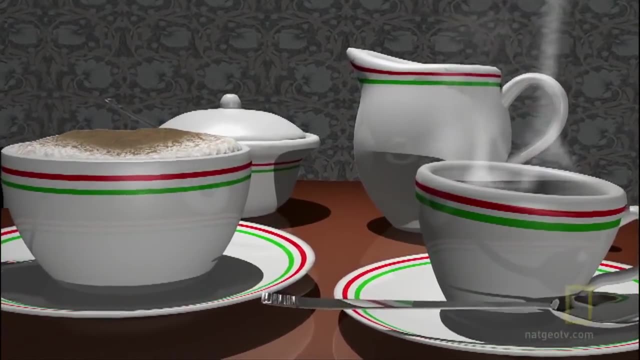 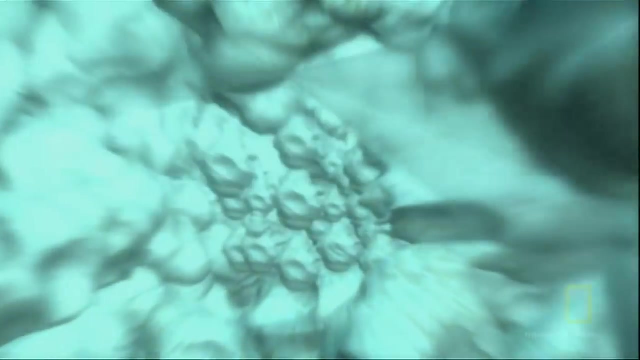 Things like coffee cups are solid Atoms join together to create something that will hold a cappuccino without leaking a single drop. Zoom in through the cup like sailing through the cosmos, past the molecules and into the atoms. The solid cup is nothing more than a fabric of atomic particles. 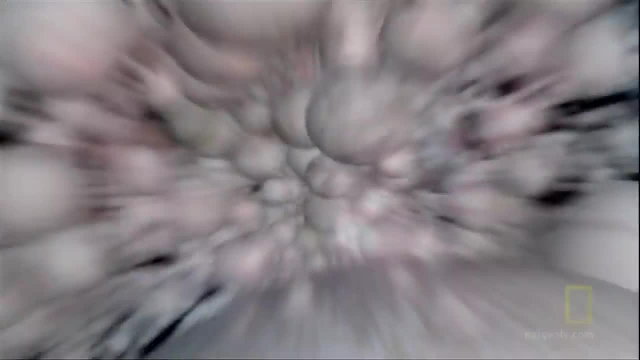 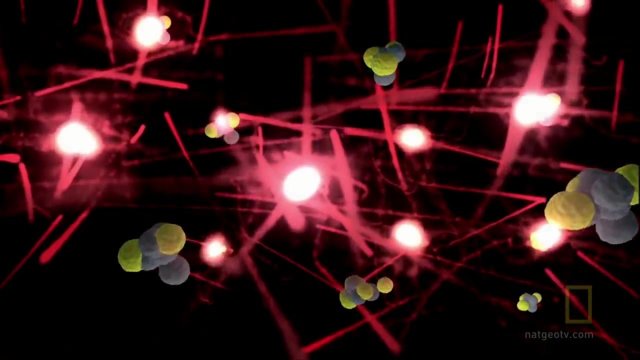 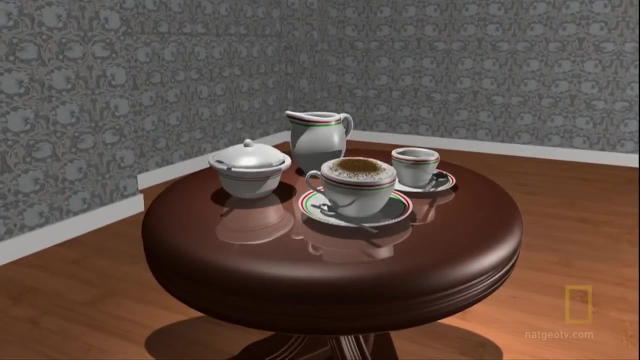 that formed a bond to become matter. If these particles were to move apart, the bonds that hold this cup together stop working. The atoms no longer support molecules. The connections between the minuscule particles dissolve. Matter in the form of this cup ceases to exist. 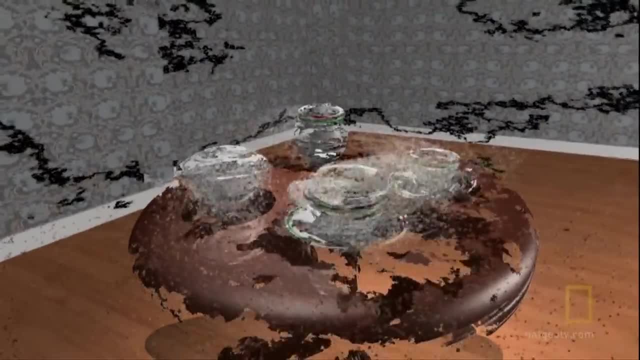 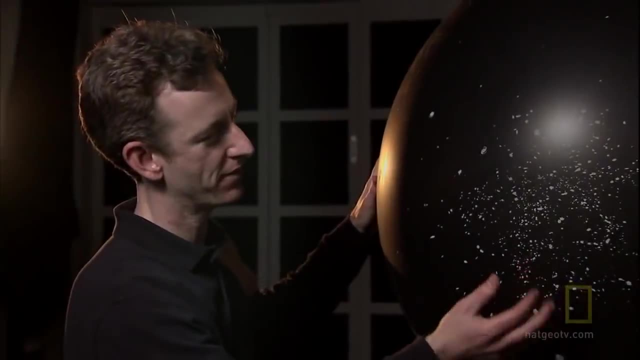 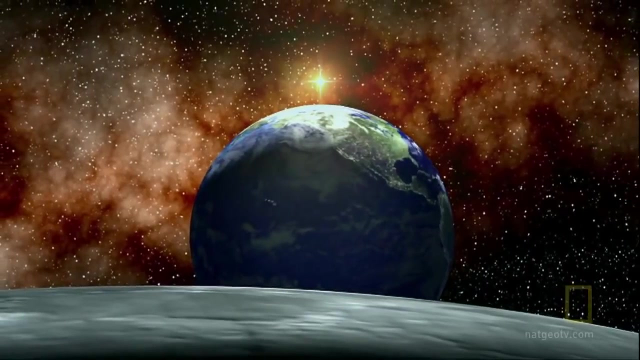 It disintegrates, gone from existence. This is the dramatic end that Robert Caldwell foresees for the universe. What you would see if you were standing on Earth or standing on some other planet that happened to still be around at that time? you would see something that looks like a wall of darkness approaching you. 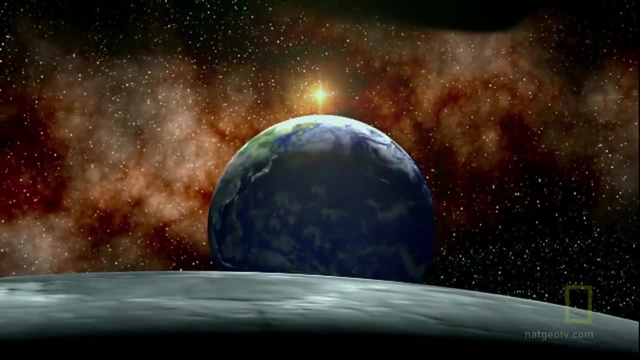 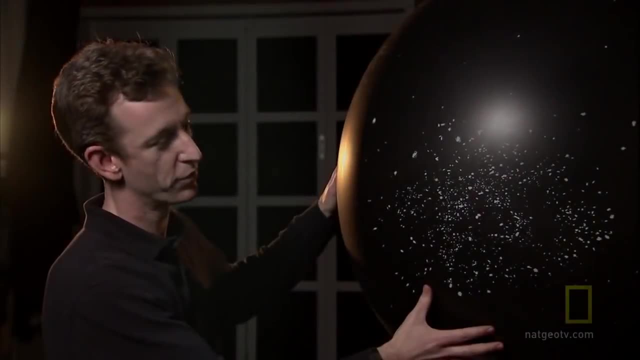 And as the wall of darkness approaches, stars would go out, galaxies would go out, and then eventually that wall of darkness would surround the planet, and then, pretty soon, atoms themselves are torn apart, and that's it Just the wall of darkness shrinks down to a point. 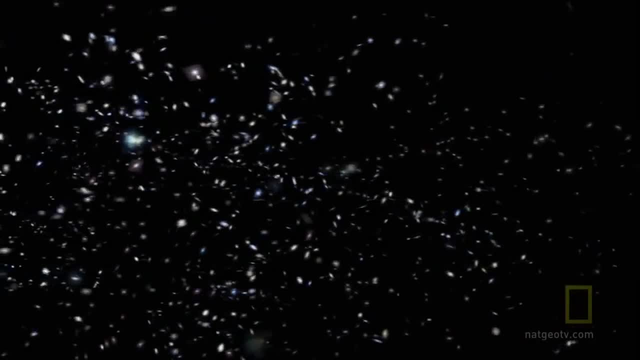 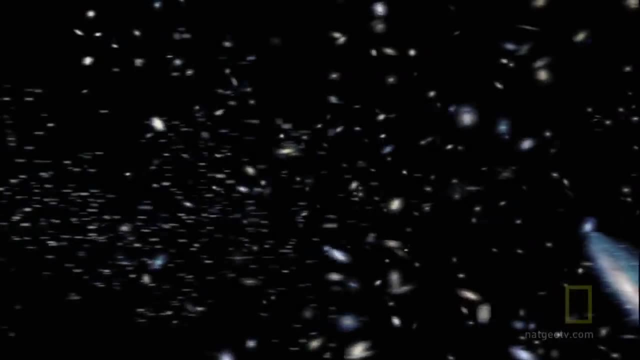 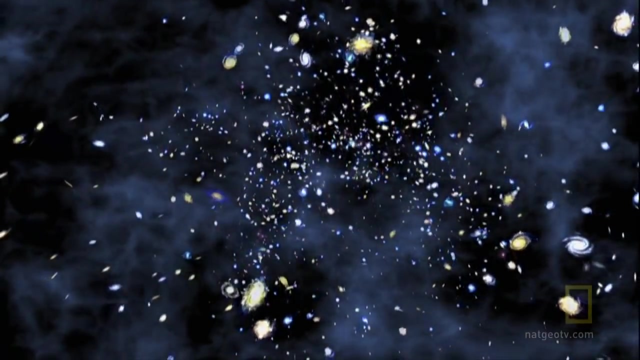 and that's the end of the universe. According to Robert Caldwell, that moment is still billions of years off, leaving plenty of time to refine the research. In a way, this is like a detective story: We're trying to figure out what is the culprit, or who is the culprit. 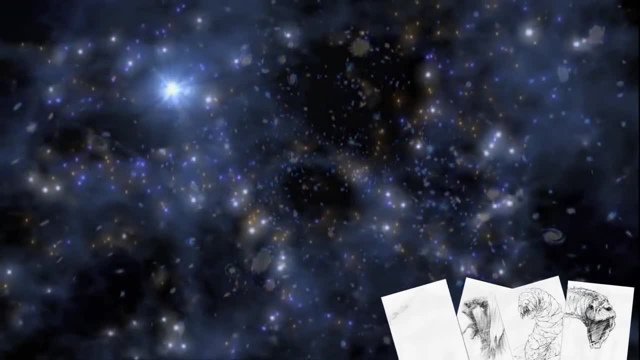 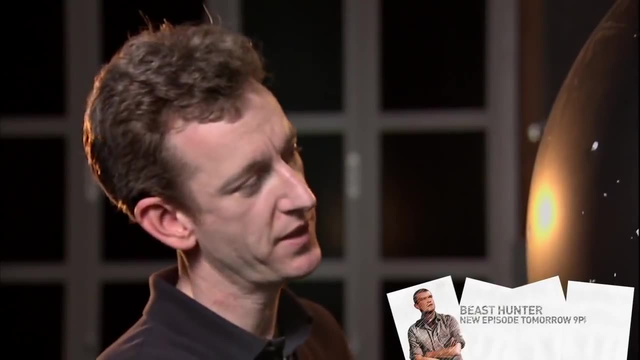 responsible for the cosmic acceleration. We think we know its name- We call it dark energy- but we don't know the modus operandi. We don't know exactly how it works. What's needed is more information, more information about the physics behind the dark energy. 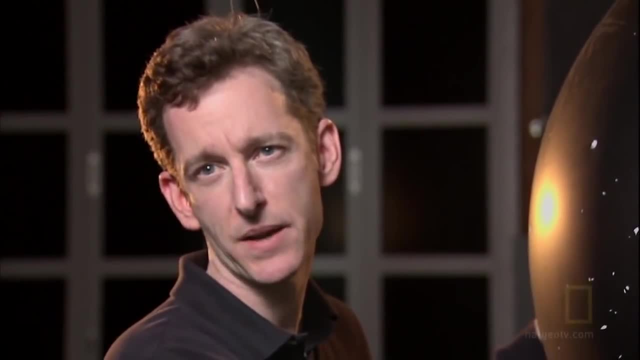 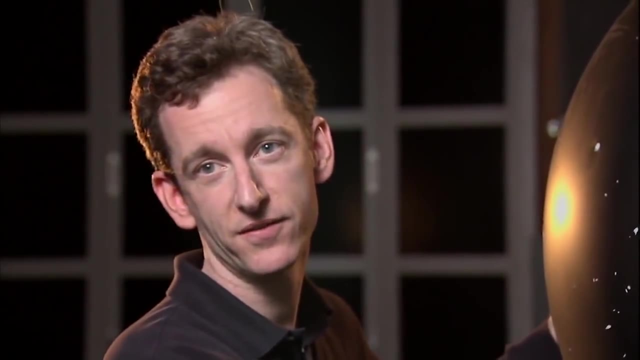 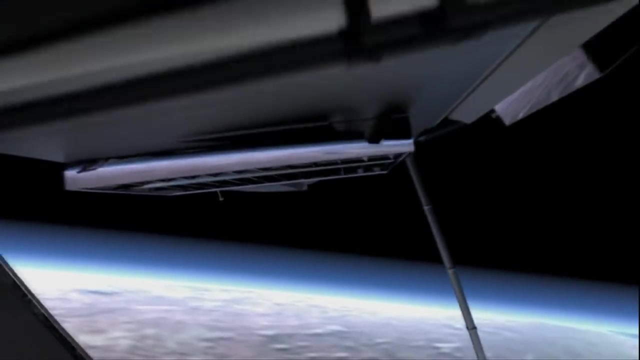 We want to know exactly what it does and exactly what it's made out of, And in answering those questions we'll be able to figure out exactly what is the fate of the universe. The Big Rip is one theory Cruising just above Earth's atmosphere and peering deep into space. 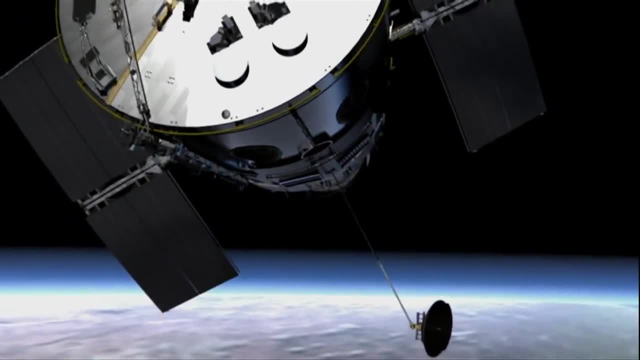 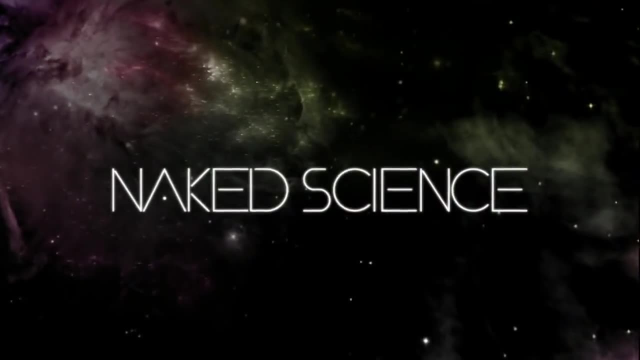 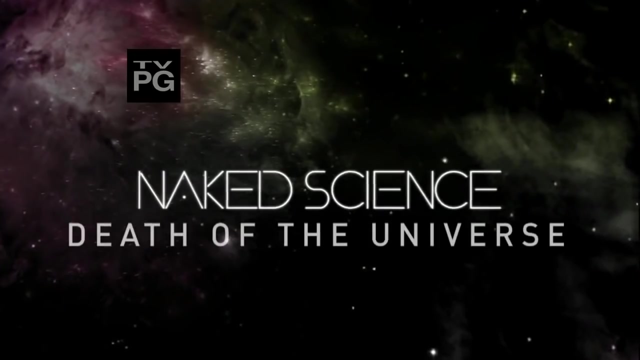 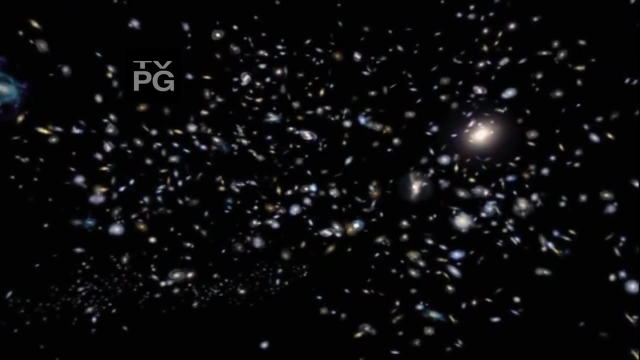 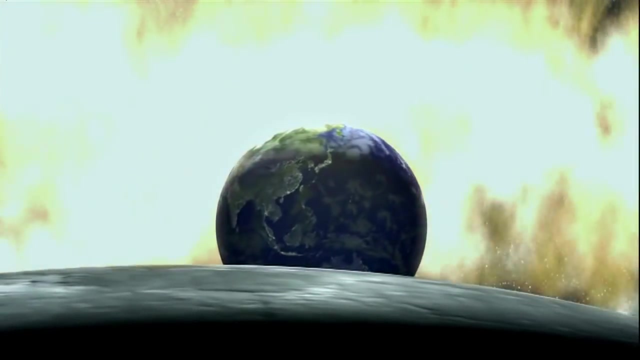 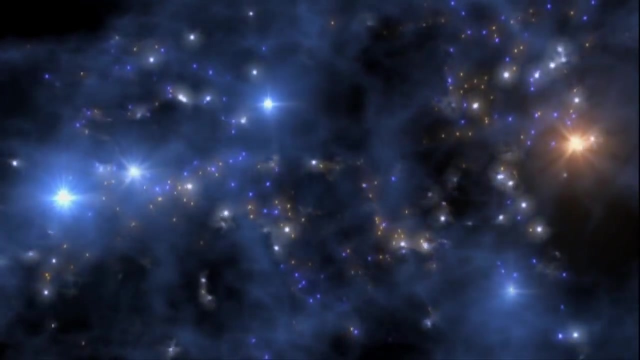 the Hubble telescope provides scientists with clues to a less violent but equally unavoidable end of the universe. Scientists now say the universe is expanding and that, depending on how fast it is accelerating, it might end in a big rip where everything tears apart. It's also possible that it will continue to expand, but at a slower rate. 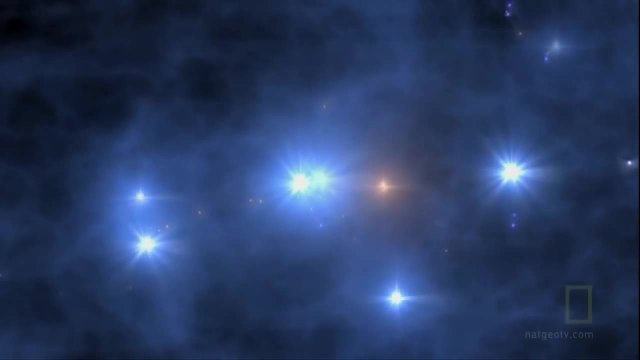 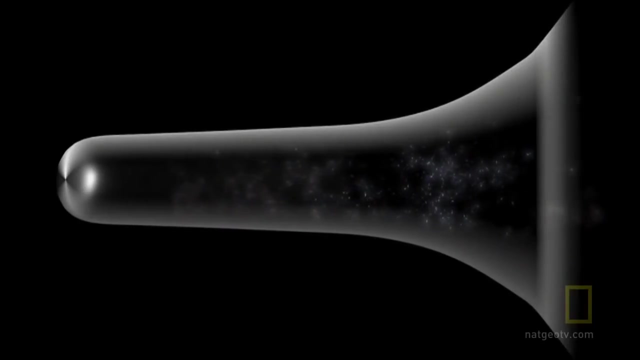 The universe wouldn't rip apart, but would become dark, cold and lifeless. If dark energy turns out to be constant, a constant property of space, and continues at the same rate that it is now, the universe will keep expanding forever, and it will be a very sad state, I think. 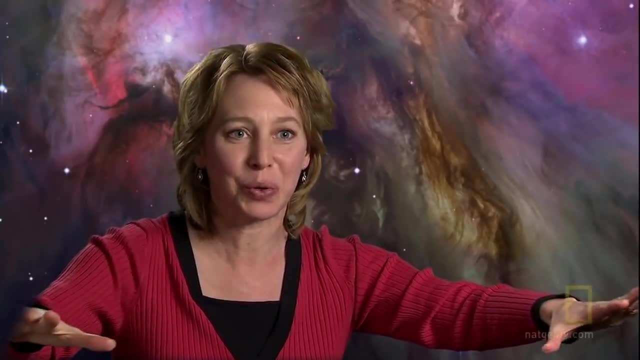 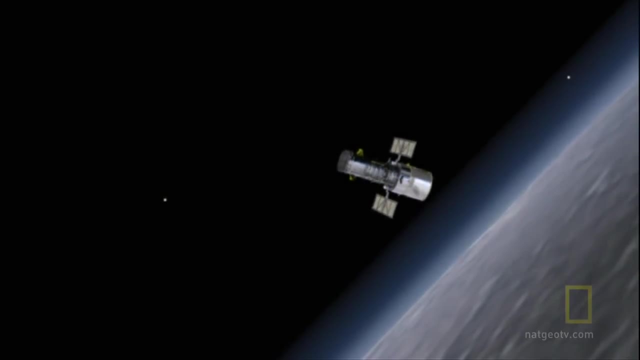 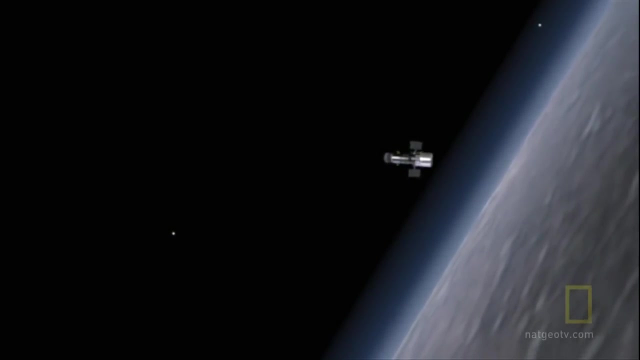 In the end it just chills out. Everything cools down. Evidence for the Big Chill. and all of the theories for the end of the universe in part come from the Hubble Space Telescope. It has been orbiting Earth since 1990 and has an unobstructed view of the cosmos. 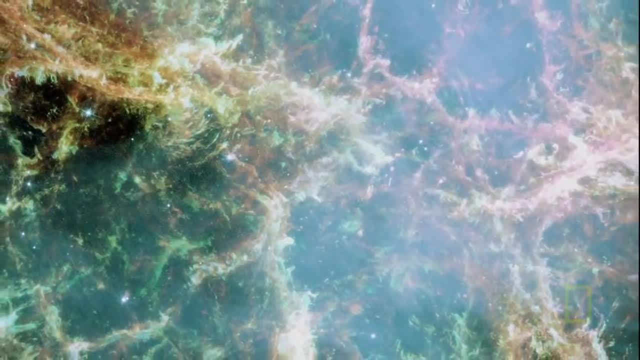 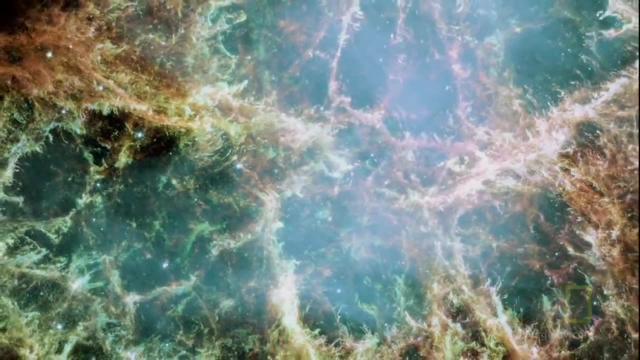 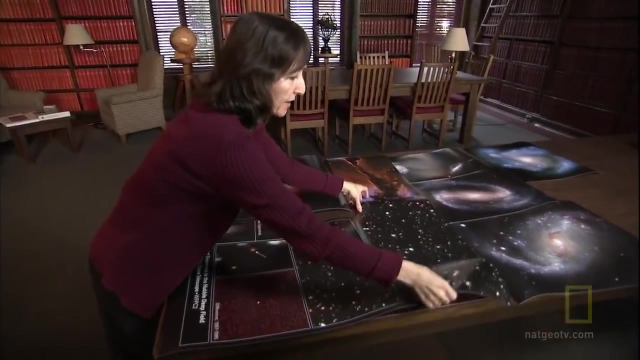 The extraordinary images it beams back to Earth are amazing in their clarity and detail And because of Hubble, scientists can make better predictions about how the universe will end. So here is an example of a very deep field that was taken by the Hubble Space Telescope. 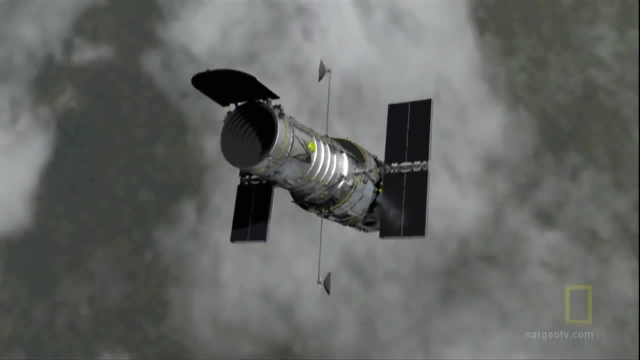 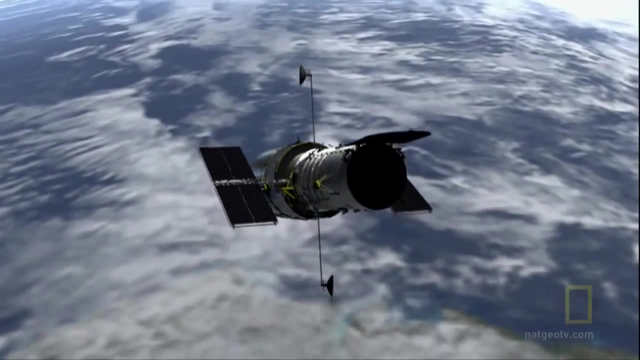 which, literally, you point the space telescope at a single region in space And if you looked at this from a typical perspective, a ground-based image before Hubble was launched first of all, it's literally almost the size of a postage stamp. 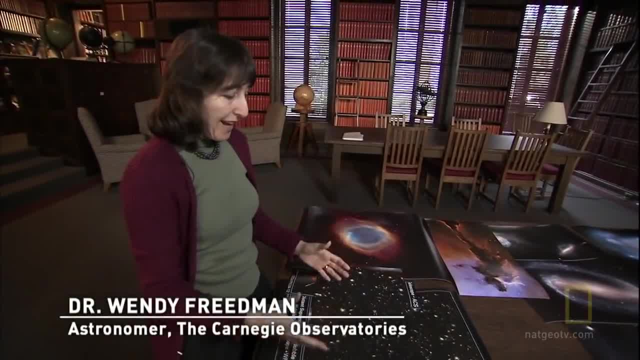 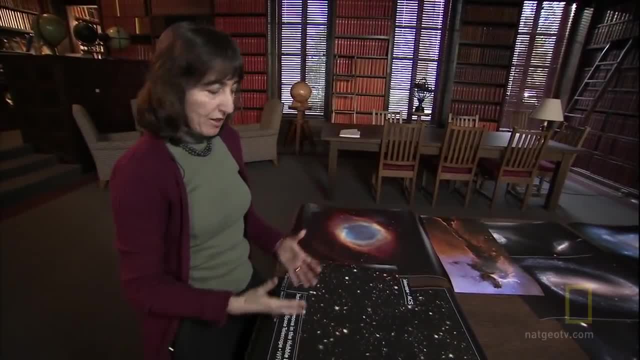 And so, suddenly, the first Hubble deep field that was ever taken had 4,000 galaxies that looked just like the galaxies here that were never visible before from the ground. Tremendous power. Each of these smudges in their own right is another galaxy. 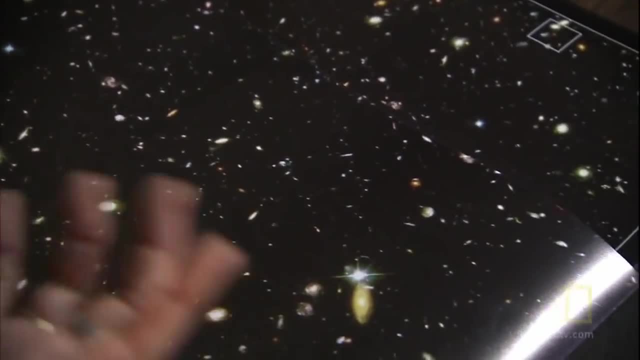 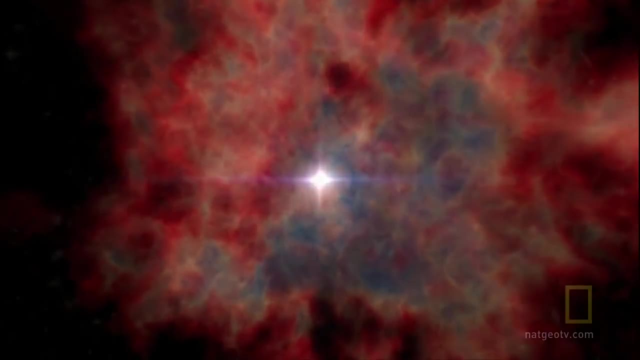 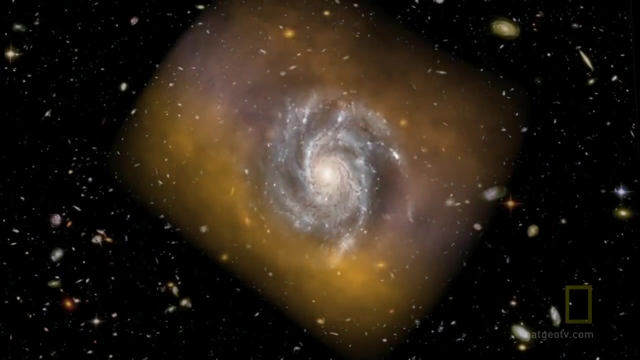 Each one of these galaxies contains about 100 billion stars. Hubble sees more than just stars and galaxies. It just might be on to one of the key ingredients of space, an invisible ingredient that could put the brakes on dark energy's effect and cause a big chill. 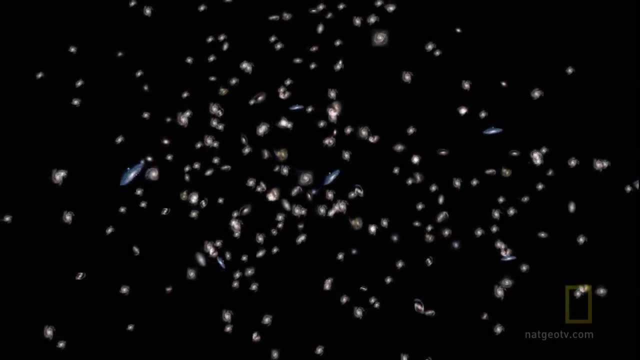 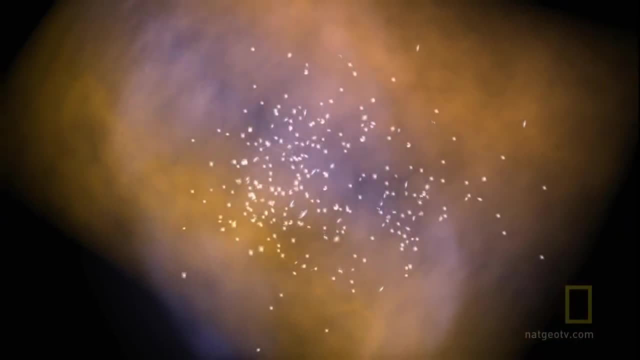 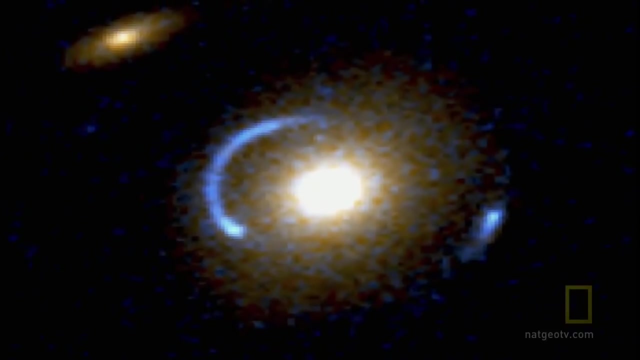 That's dark matter. Scientists talk about dark matter as the substance that holds the universe together and could prevent a big rip. Evidence that dark matter exists is seen in some of Hubble's images of nearby galaxies. It sometimes appears as though other galaxies surround them. 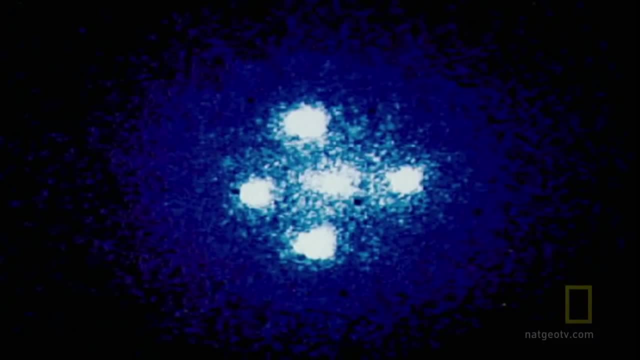 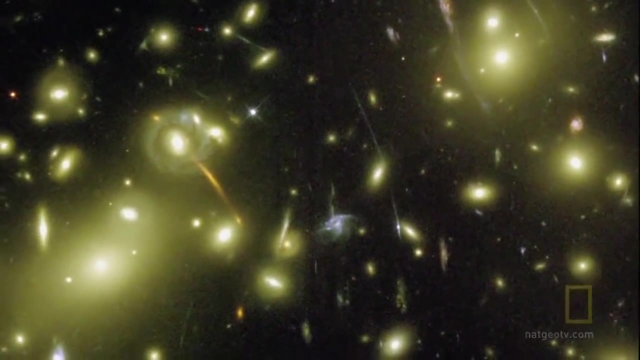 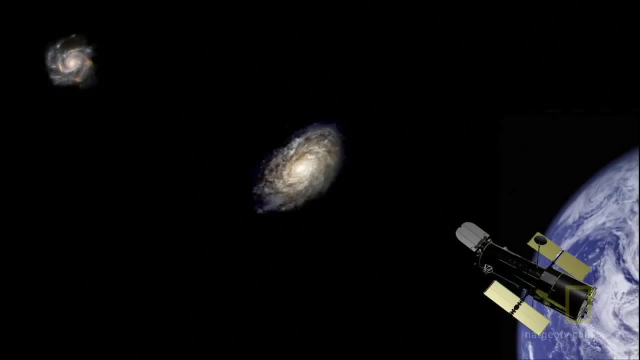 The other galaxies are not really there at all. Rather, they are reflections of more distant galaxies coming from behind. Astronomers suspect this optical illusion is dark matter, causing a weird distortion of light called gravitational, lensing The light from the more distant galaxies. 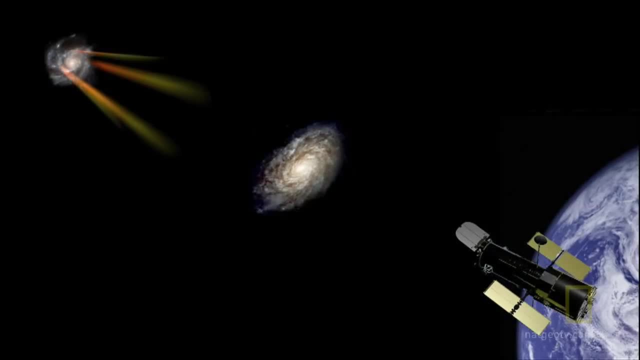 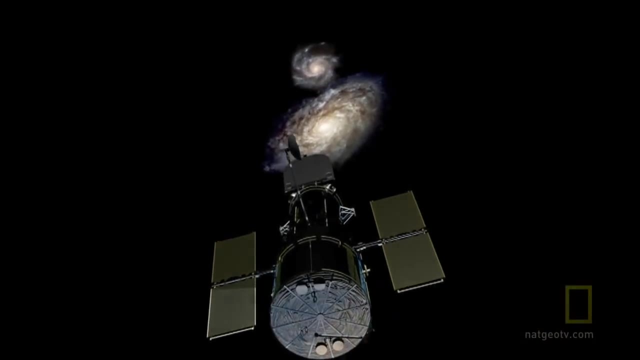 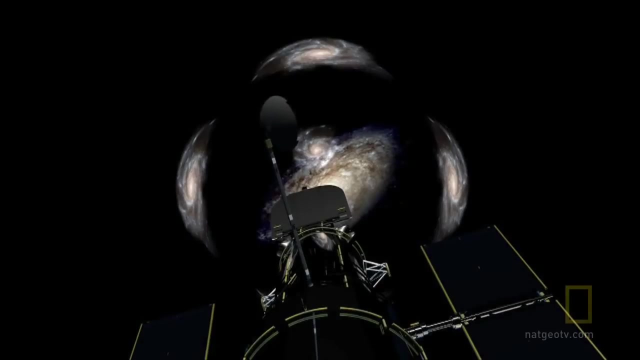 is literally bent by the curvature of space caused by stars and dark matter in its path. The more dark matter there is between Earth and the distant galaxy, the more the light will be bent and the greater the force to cause a big chill. The gravitational lensing is a tremendous tool for the astronomer. 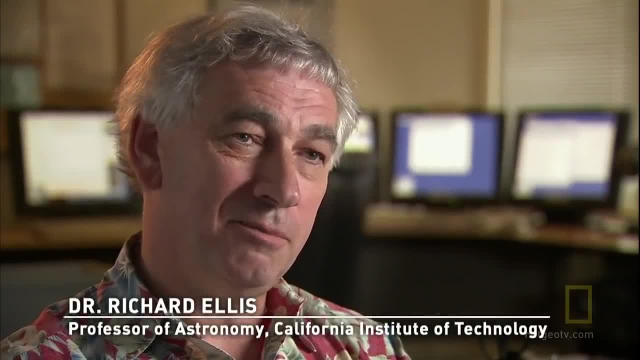 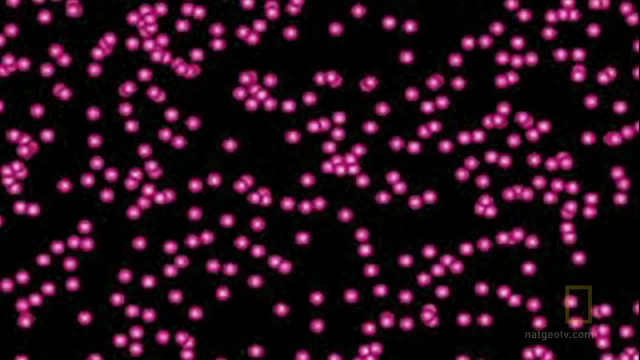 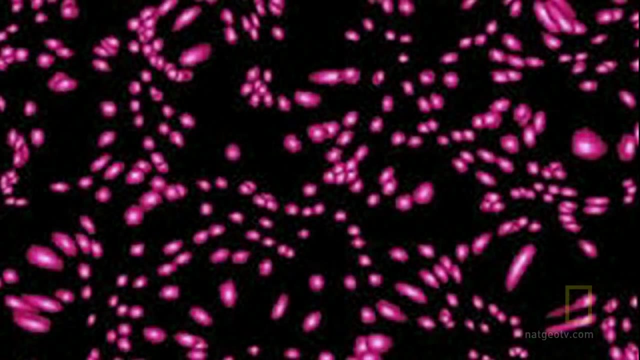 because we can measure the distortion in background galaxies and use it to trace the distribution of dark matter on various scales. We're looking at a distribution of idealized galaxies here on the sky, and the light from these distant galaxies is passing through clumps of dark matter. 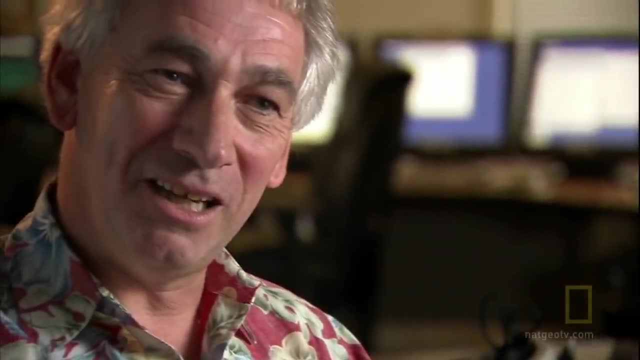 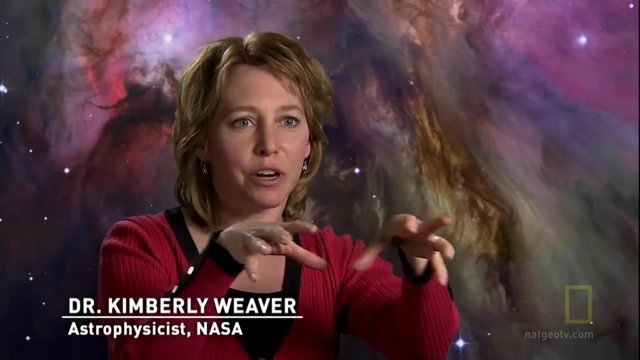 What you look at is not really what's happening. It's a bit like wearing spectacles and not knowing that you're wearing them. If you can tell how much that bending is occurring, you can map the dark matter and you can also see. well, if there's dark matter, there is the universe around that dark matter behaving the way it should, given the gravity or not? If it's slightly gravitating less, then dark energy might be changing in those places, Identifying which energy force dominates: dark matter or dark energy. 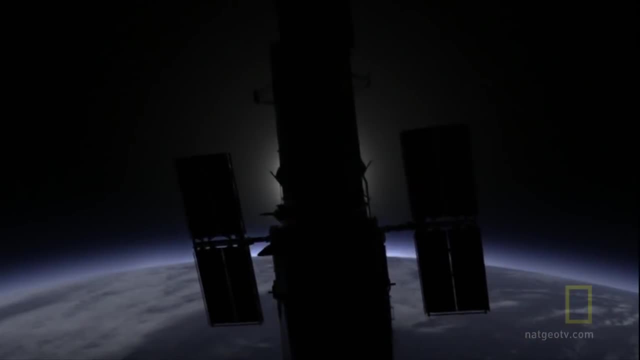 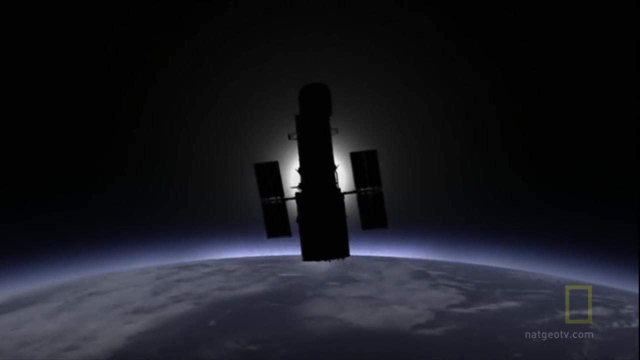 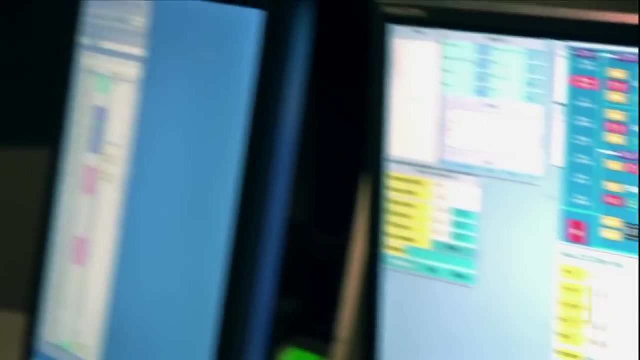 will give scientists more confidence about whether a big chill or a big rip will be our fate. The best evidence shows dark energy as the driving force, but by how much? Solving this mystery depends on astronomers finding ways to measure how fast the universe is moving. 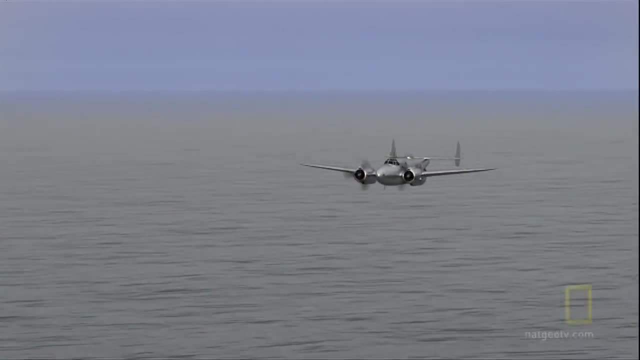 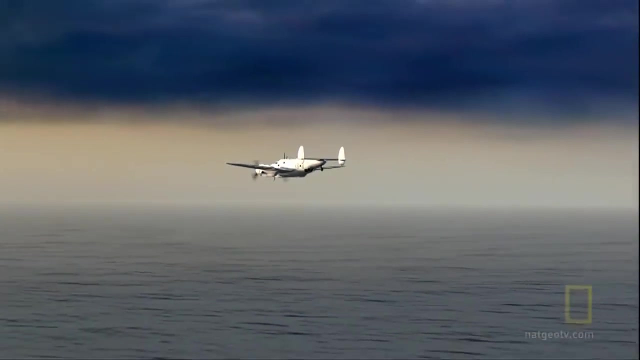 On Earth. it's simple to determine how fast something moves. An airplane, for example, is relatively close. We can look at it and calculate its speed by estimating the distance it travels and timing how long it takes to get from one point to another. 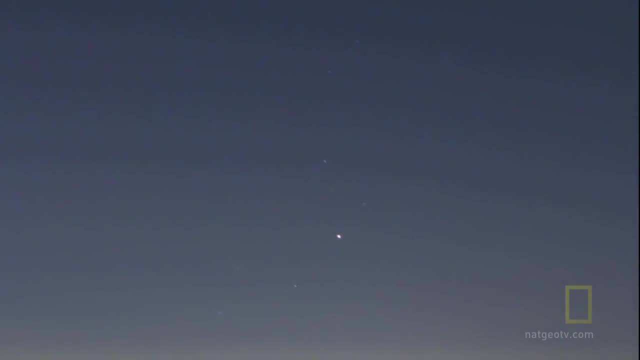 But a star's light can travel for millions or billions of years before it can be seen on Earth. By the time its light gets here, the star will be long gone and it's too far away to gauge its speed or distance traveled with any certainty. 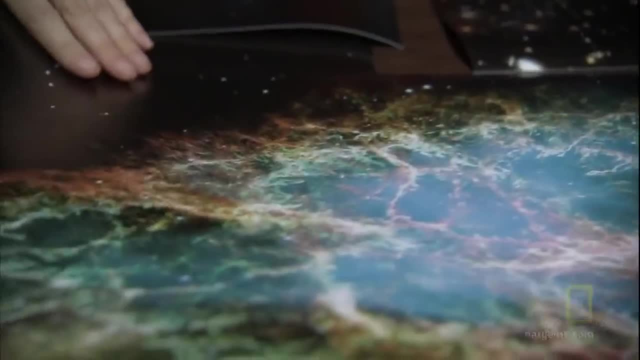 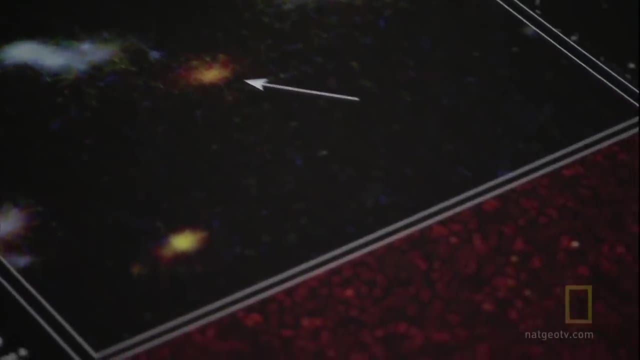 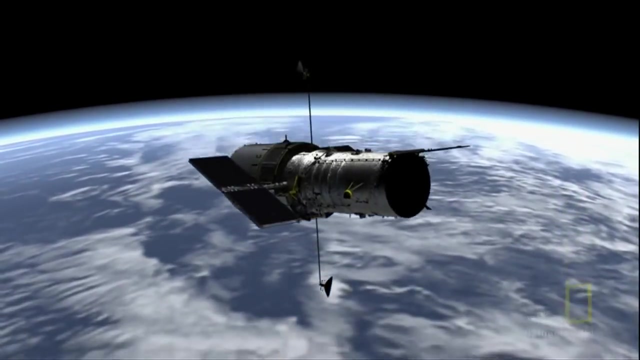 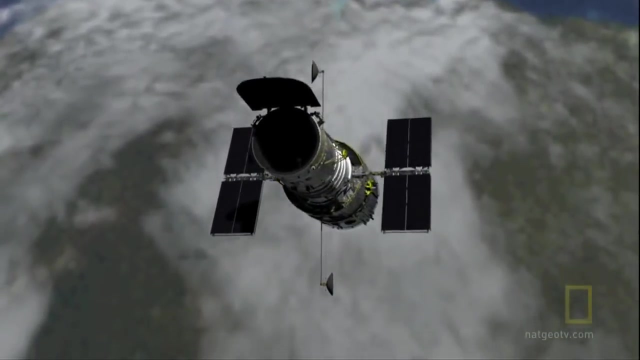 The universe is expanding. only scientists cannot give precise answers about how fast. The mystery moves closer to being solved by imaging the cosmos with greater precision. Clearer images from space make it easier to estimate the rate of expansion If the universe continues to expand with time. 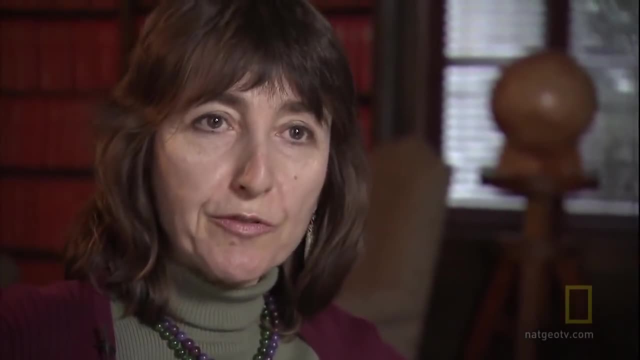 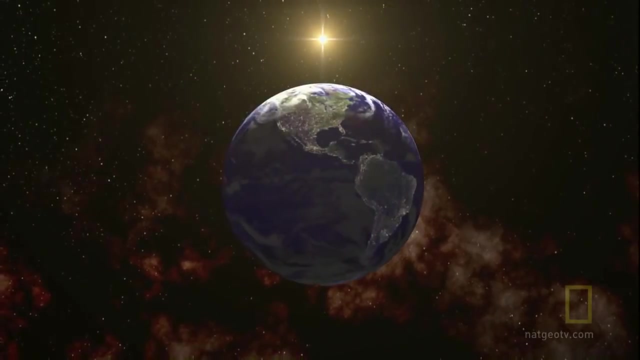 then ultimately, all of the energy sources, the nuclear furnaces and stars would run out and die and the universe would actually get very cold and there'd be something called a big chill. In the big chill scenario, Earth could become a lonely cold planet. 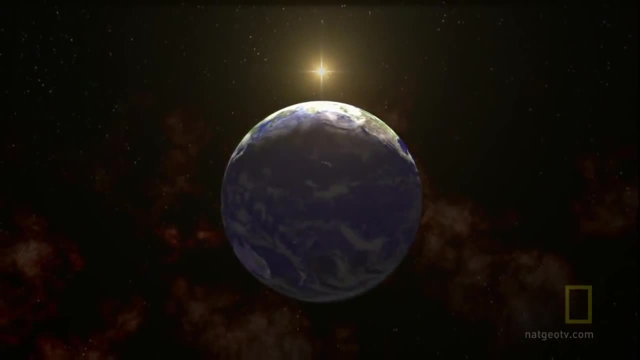 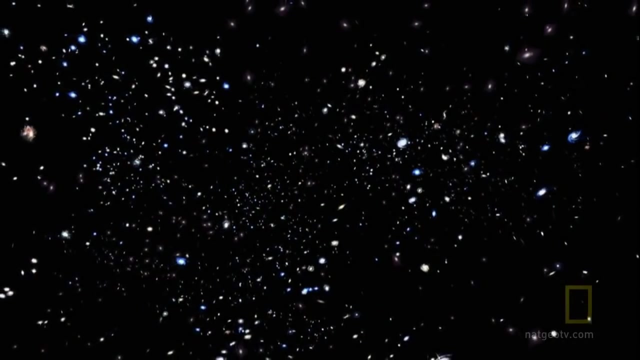 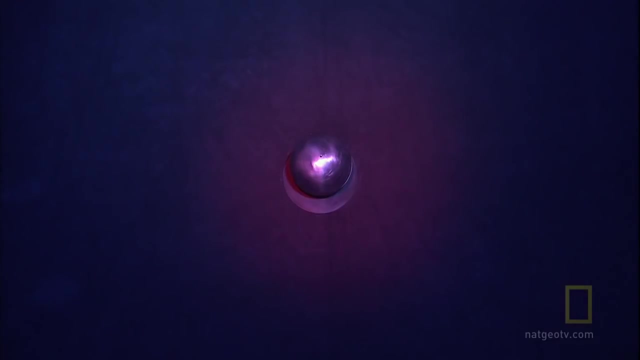 as the universe expands, Distances between stars grow so vast that they nearly disappear from view. Over time they burn out and eventually the entire universe ends in a frozen state. This sphere demonstrates the principles behind a big chill. The marbles coming out of the sphere. 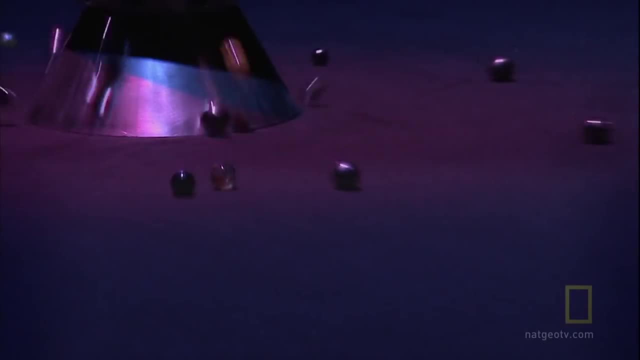 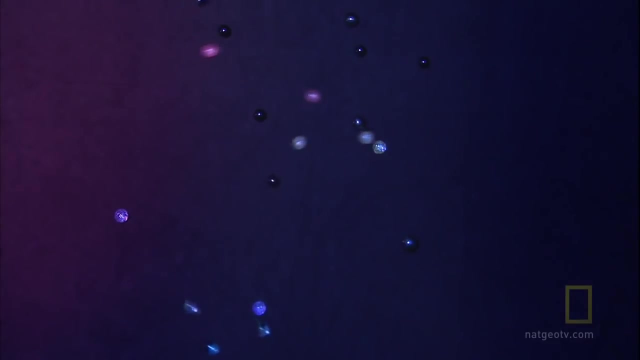 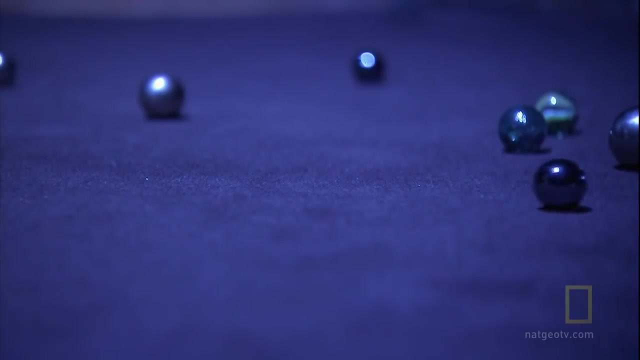 are like stars that were formed following the Big Bang. Dark energy propels the stars away and the stars outward. Dark matter slows them down In a big chill. the expansion would continue, but the nuclear fuel that causes the stars to burn will eventually run out. 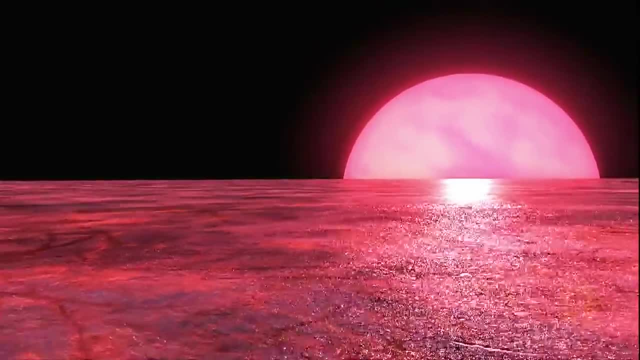 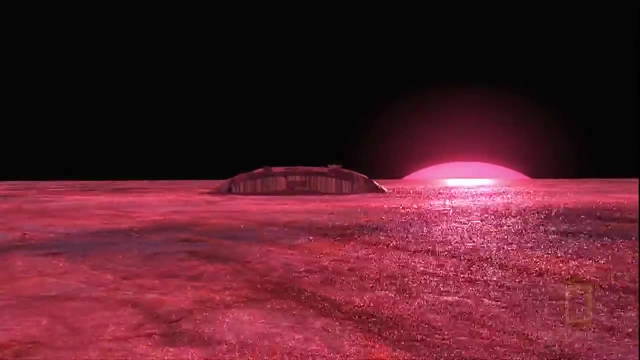 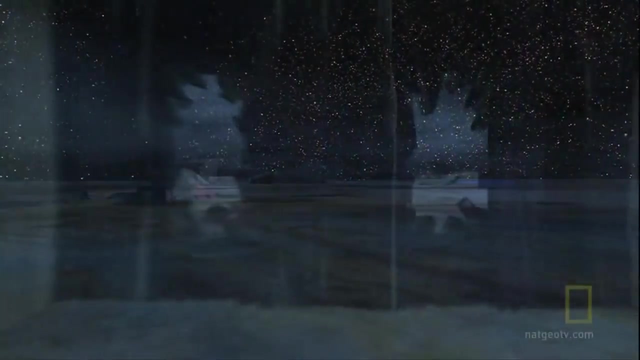 From Earth's perspective, the first thing to go would be sunlight. The sun dims as it exhausts its last bits of nuclear fuel. Earth would freeze and become lifeless And billions of years after humans are gone, the cosmos expands out of view. 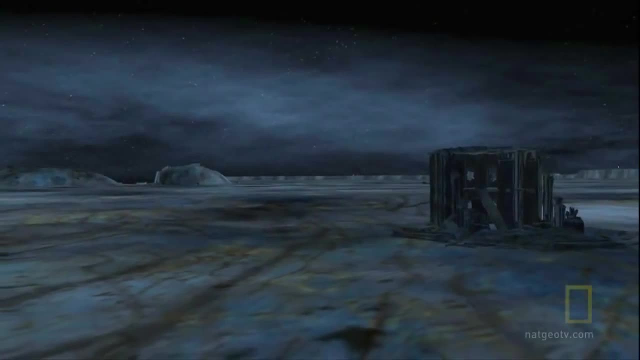 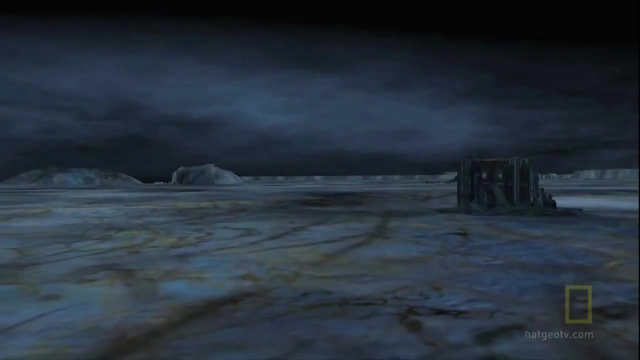 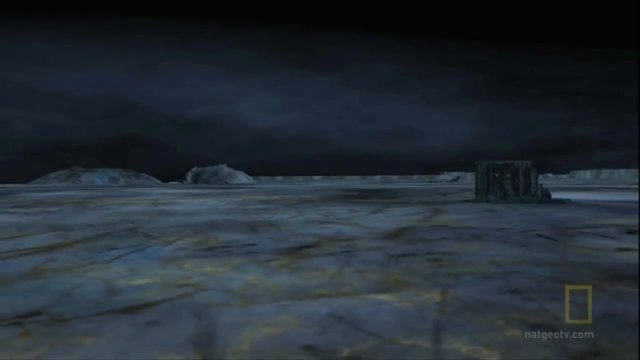 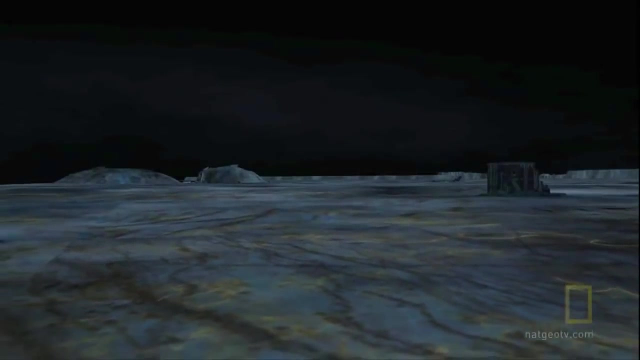 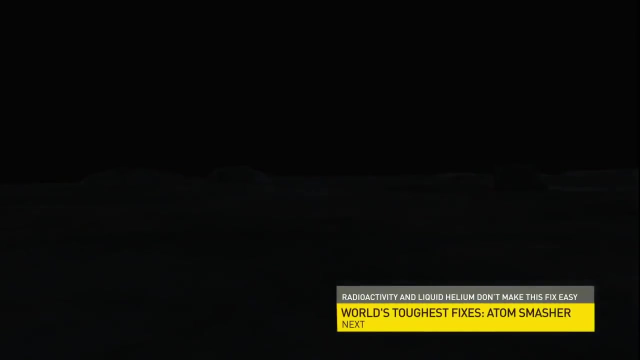 A few newer stars might remain, but most would have long moved away. The furnace powering the universe burns out. The darkened universe continues to expand a frozen and lifeless remnant of its once vibrant existence. Eventually, if this keeps going, if nothing changes in the composition of this energy density, 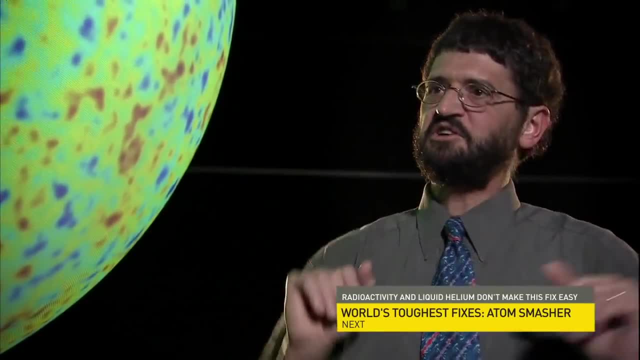 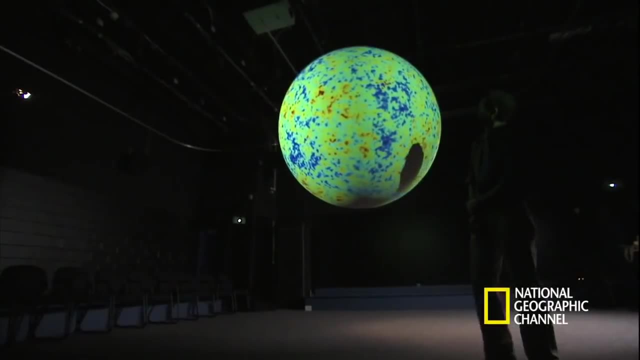 the universe will continue to expand forever. It's going to get colder and colder And eventually even our neighboring galaxies will be receding from us so fast that we won't be able to see them. So the universe is going to get cold and dark. 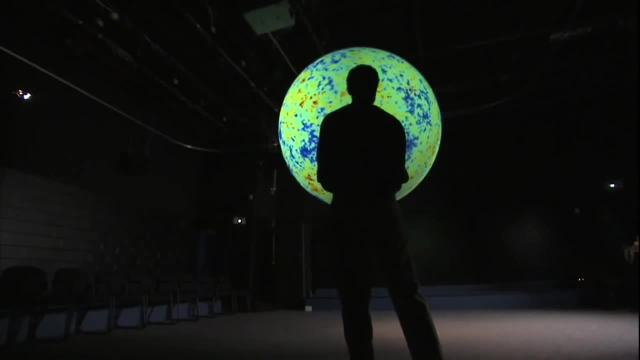 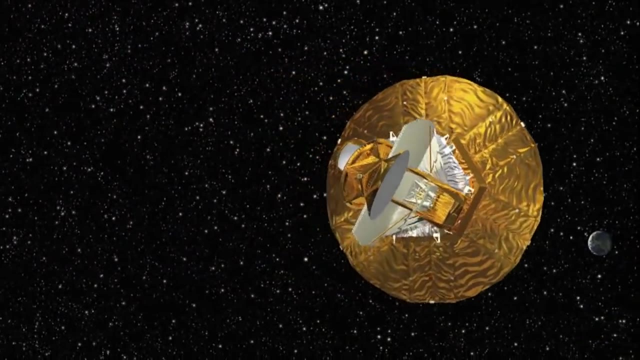 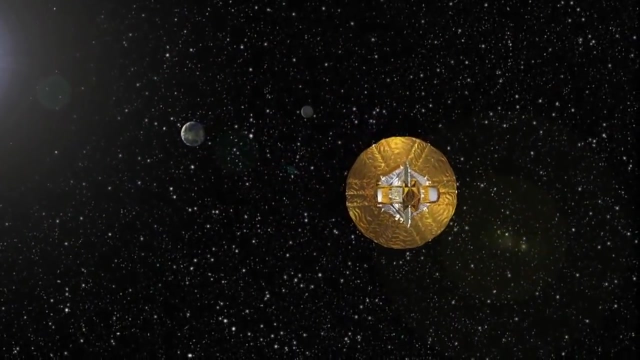 and it will be a very lonely place. Astronomers have much to learn about the influence of dark energy and dark matter, And much of the newest information is coming from this probe in deep space. It's sending back information that's helping scientists to interpret the history. 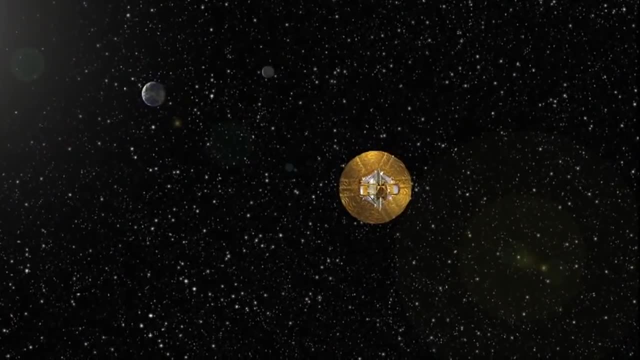 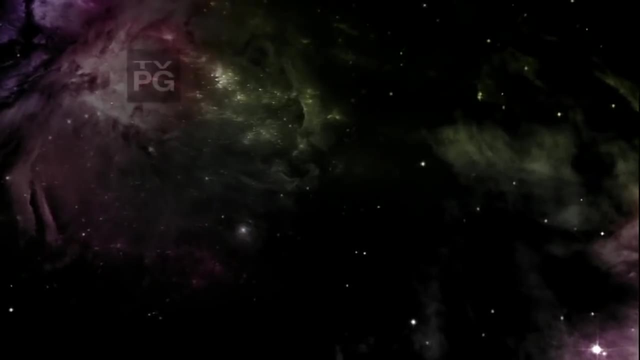 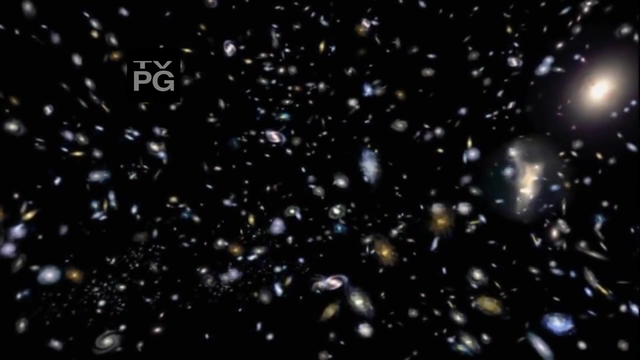 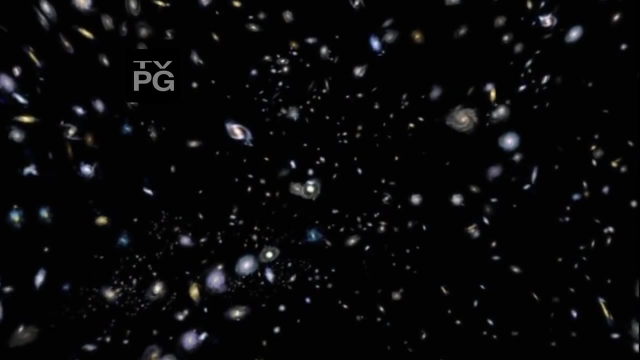 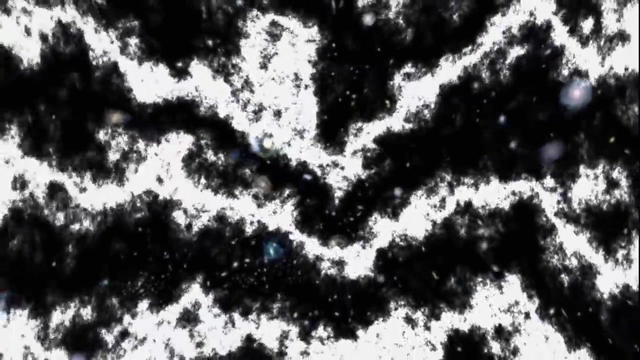 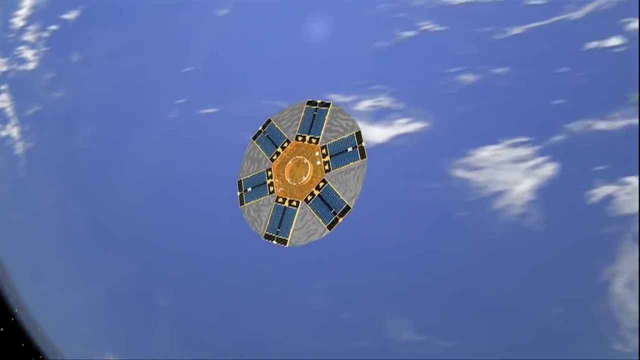 and the fate of the universe. The night sky, by all appearance, is a quiet and peaceful place, But in reality there are forces that are driving it to an end. Big science moves astronomers closer to deciphering the universe's great mysteries. 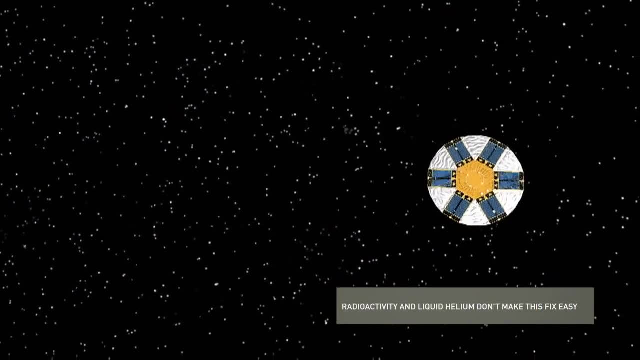 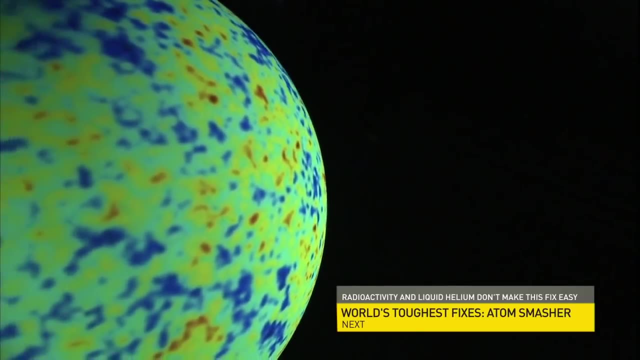 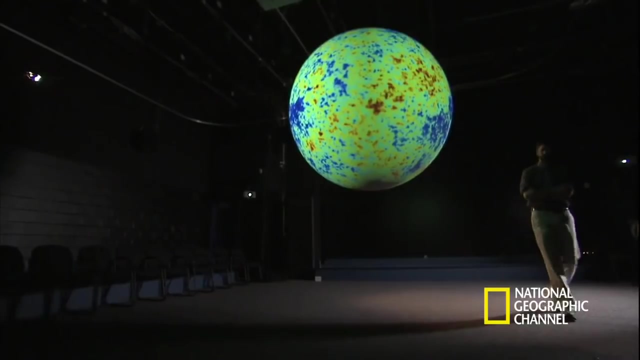 Including its ultimate fate. The solution to the universe's riddle may well be hidden in this multicolored image. What's incredible is that it's a map of the early universe, from the moment it was conceived And, even more fantastic, it reveals a great story. 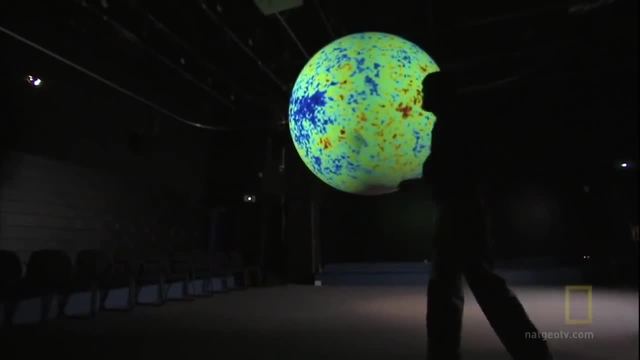 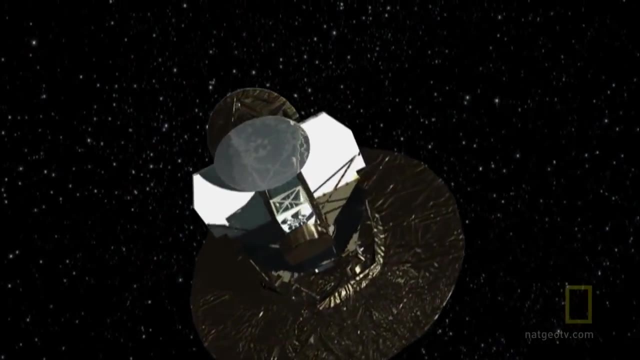 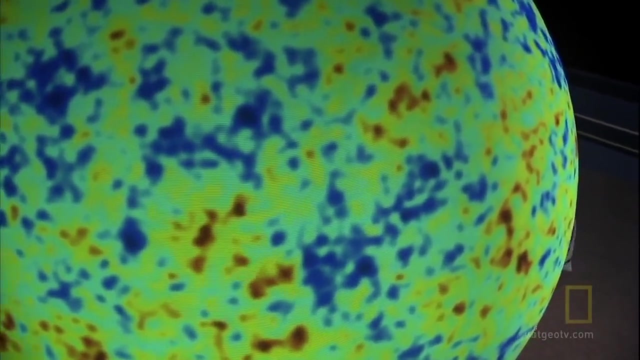 that helps cosmologists predict how it will end. The machine that captured this is called WMAP, a NASA satellite that's working around the clock to chart the cosmos. What we're looking at here is the edge of the visible universe. It's the light that WMAP measured. 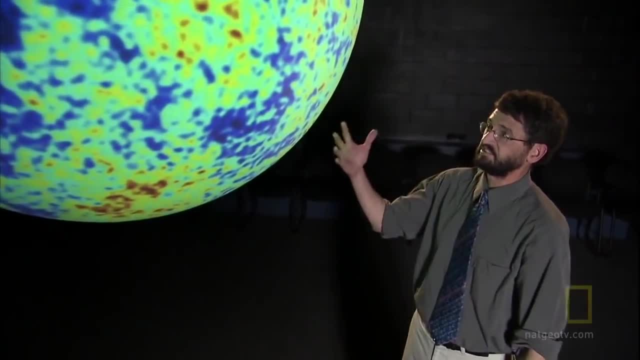 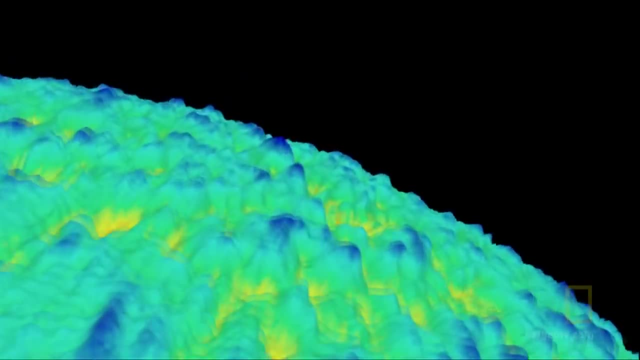 it's the remnant heat from the Big Bang, and this is literally the oldest light in the universe that we can see. This fossil relic from the early universe tells us a great deal about what the composition of matter was like, what the expansion rate was like. 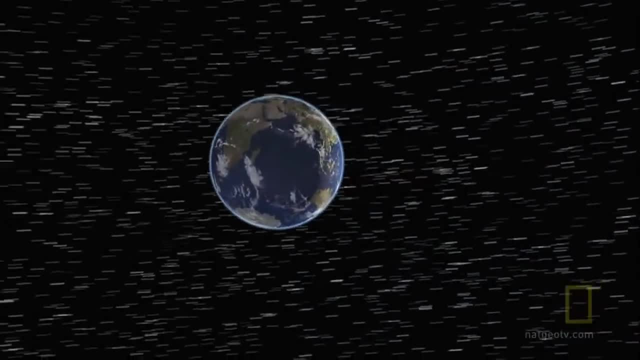 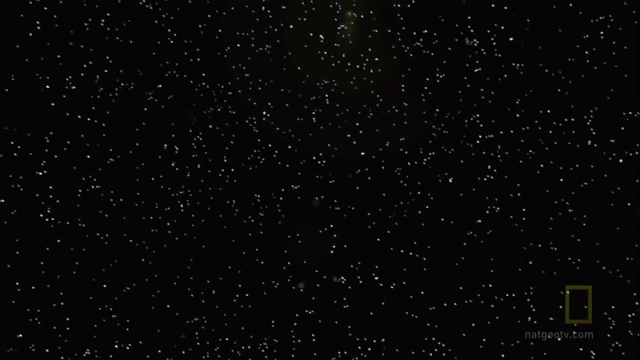 and really what the conditions were at the birth of our universe. WMAP is one of the great astronomical breakthroughs of the 21st century. Nothing before could give us such a clear image of the energy left over from the Big Bang, energy that scientists call. 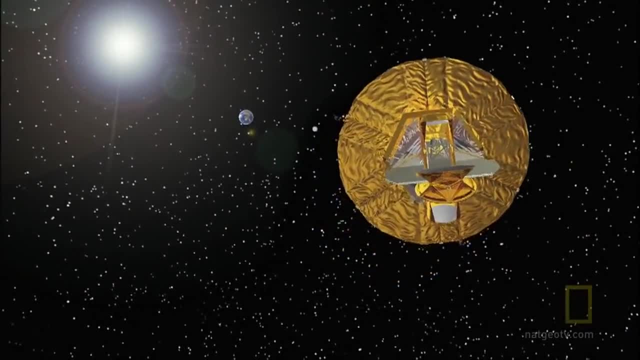 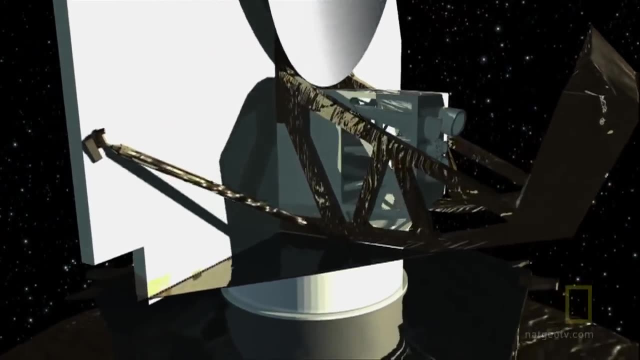 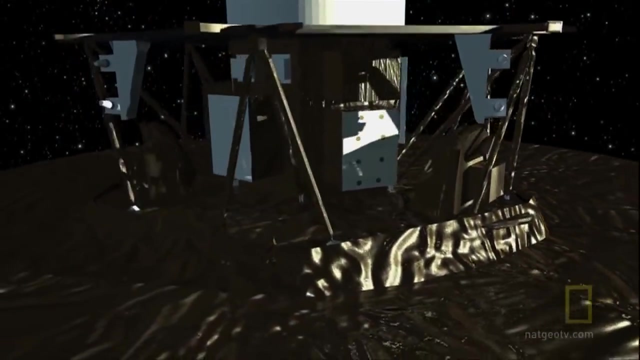 the Cosmic Microwave Background. WMAP is measuring temperature differences in the Cosmic Microwave Background, which may finally make it possible to predict which force will dominate the universe and how that force will change. WMAP is also able to predict which force will bring the cosmos to its end. 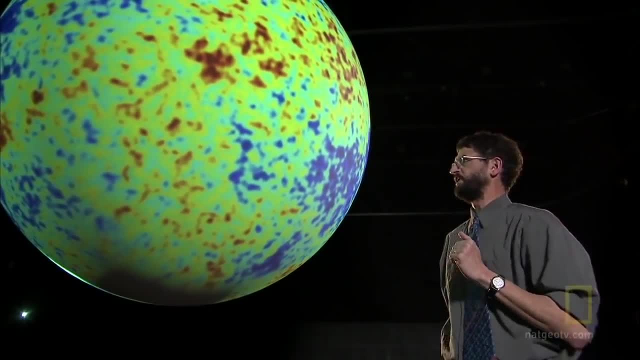 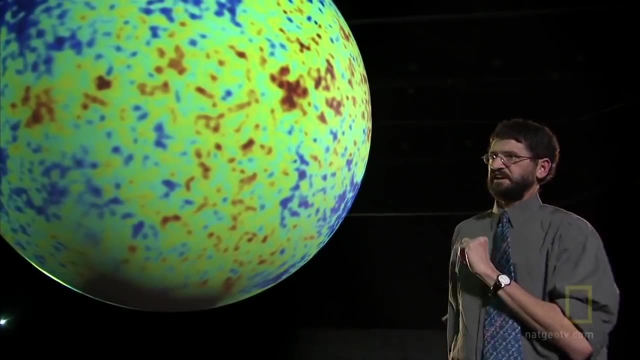 The blue spots are regions, in the microwave light that was produced by the Big Bang, that are slightly colder than the average temperature, and the red spots are regions that are slightly hotter than the average Temperature. differences revealed by WMAP tell scientists about the nature of the matter. 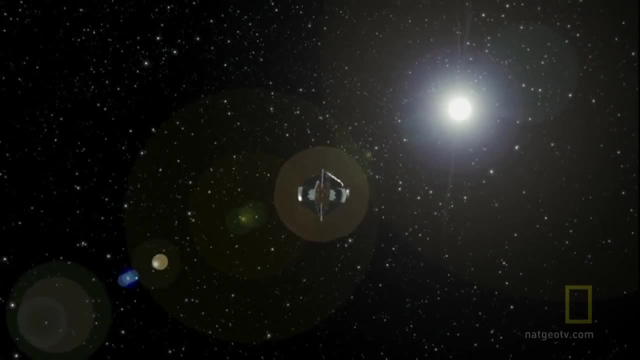 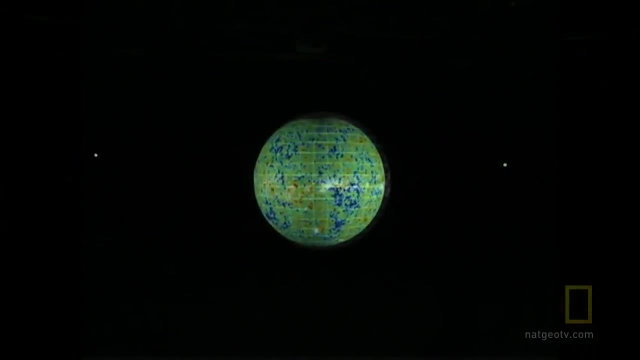 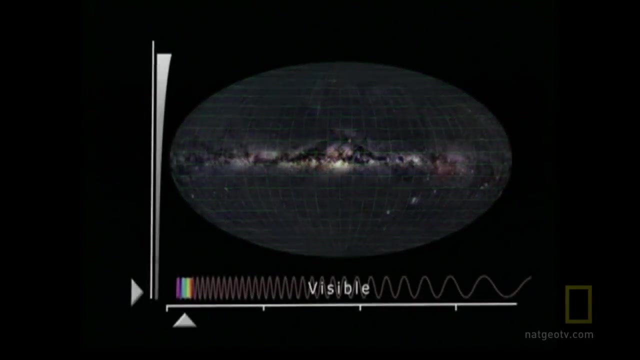 and energy that is contained within the universe. They're able to analyze the light patterns and find clues not only about the substance but also the fate of the universe. We only capture a tiny part of the electromagnetic spectrum with our eyes, and we have to go to much longer wavelengths. 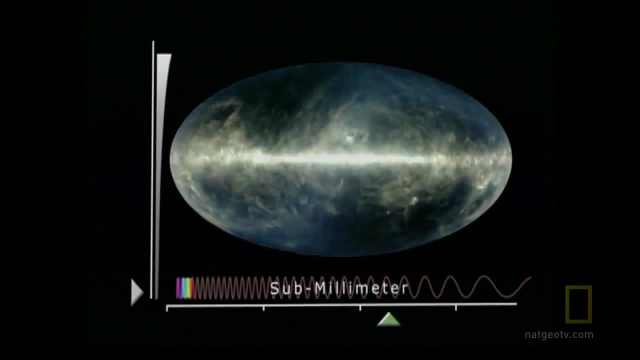 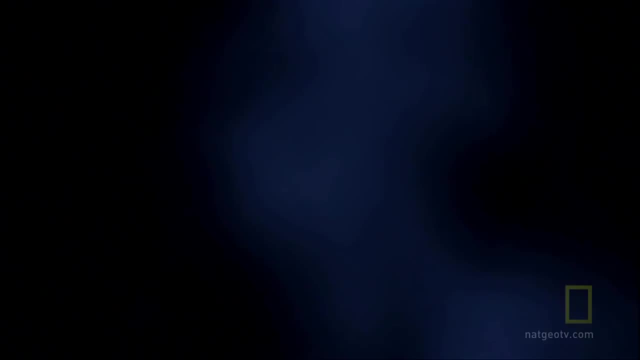 The same wavelengths that are used to heat water in a microwave oven are what we're measuring here with WMAP. WMAP is so precise that it can detect differences in temperatures as small as one one-thousandth of a degree. This sensitivity helps scientists. 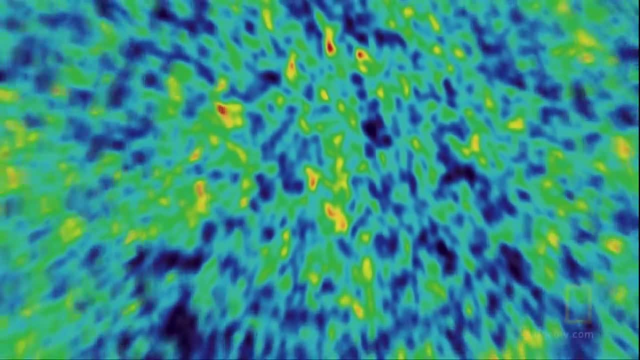 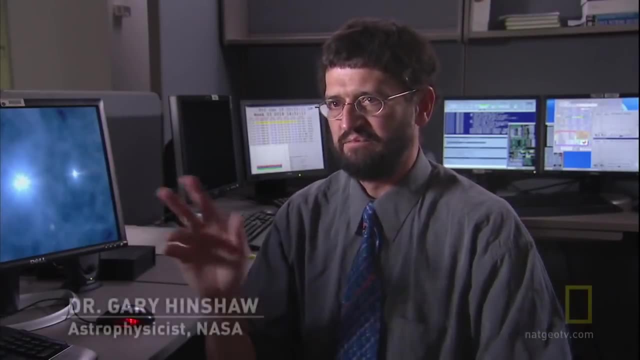 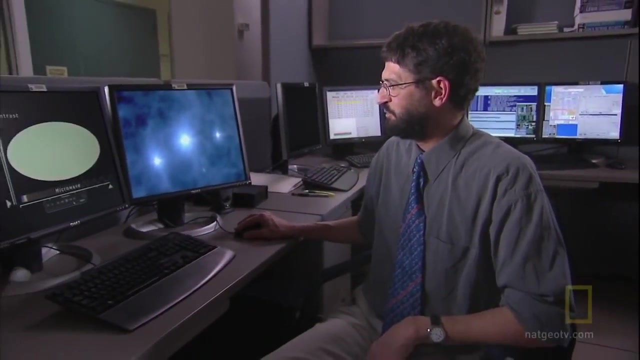 to calculate the ratio of dark matter to dark energy forces that will determine how the universe ends. We assemble all those difference measurements and make a map of what the variations look like, And by turning up the contrast we can basically subtract off this uniform glow from the Big Bang. 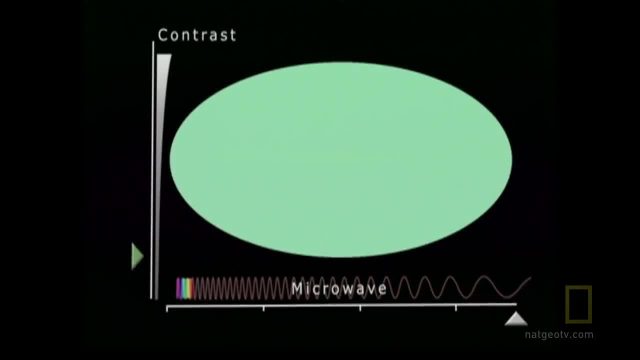 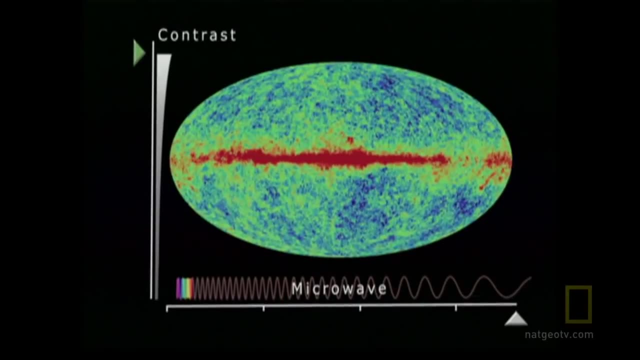 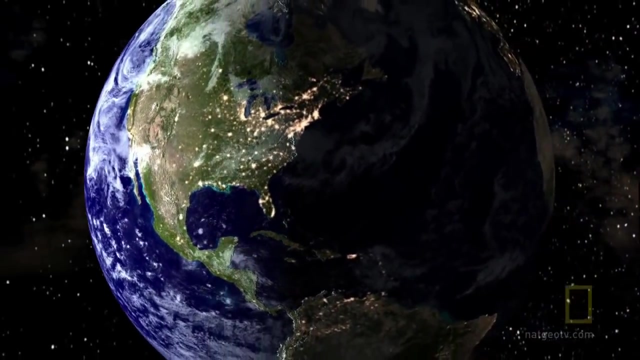 and look for variation. It doesn't look like much until Gary Hinshaw adjusts the contrast. Then the WMAP image comes. Looking at WMAP imagery is, in essence, taking a journey back through space and time so that we might get some new ideas on the fate of the universe. 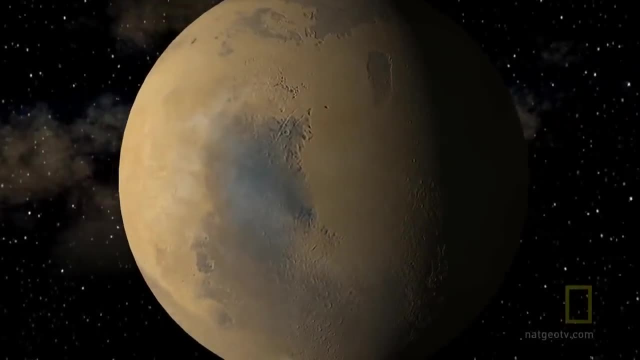 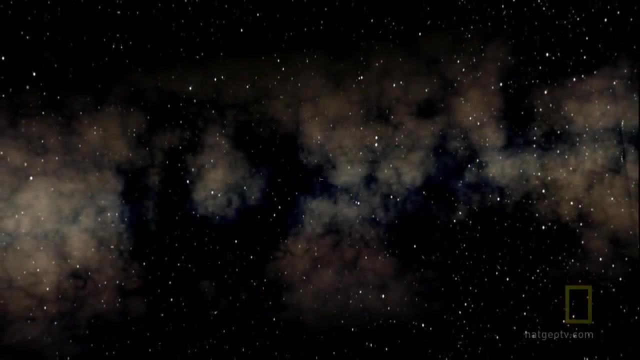 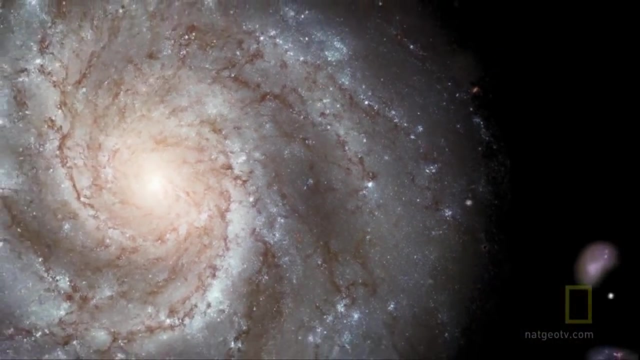 Pulling away from the probe and following the path of the light it is collecting. we pass Mars, Jupiter and Saturn, whose reflected light takes over an hour to reach Earth. Then, leaving the Milky Way, we pass Andromeda, the next nearest galaxy. 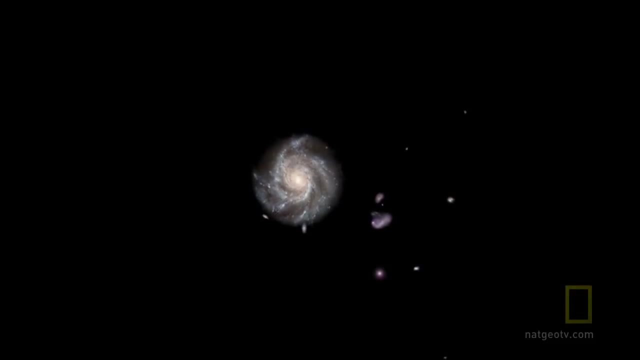 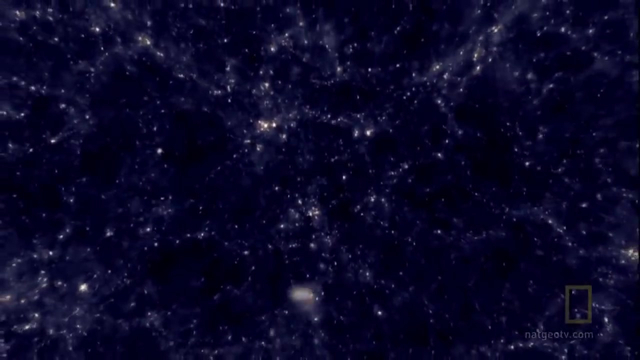 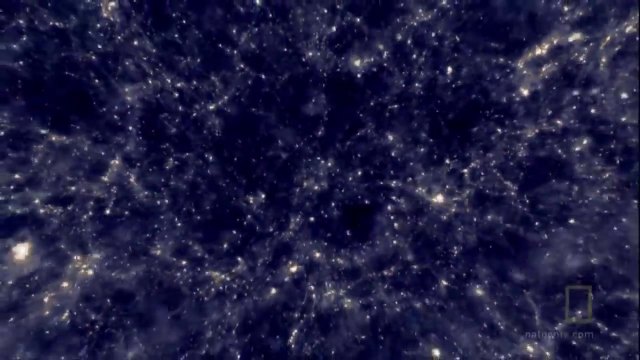 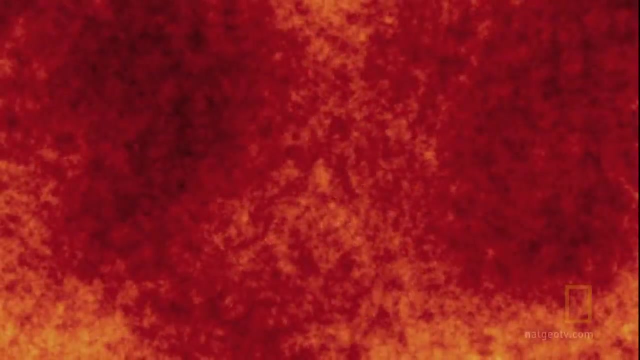 whose light takes 2.3 million years to reach us, which means we have traveled 2.3 million years back in time. And finally we arrive back 13 billion years ago, at the beginning of visible light. Before that, superheated hydrogen gas is everywhere. 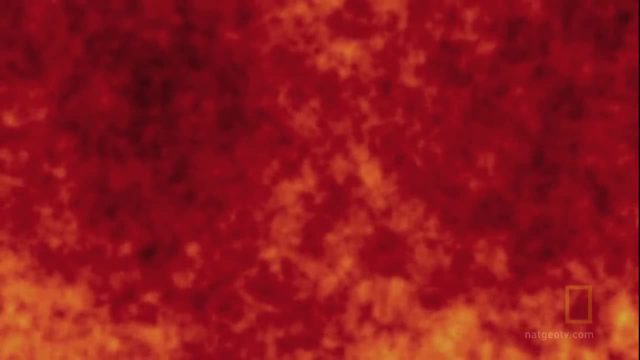 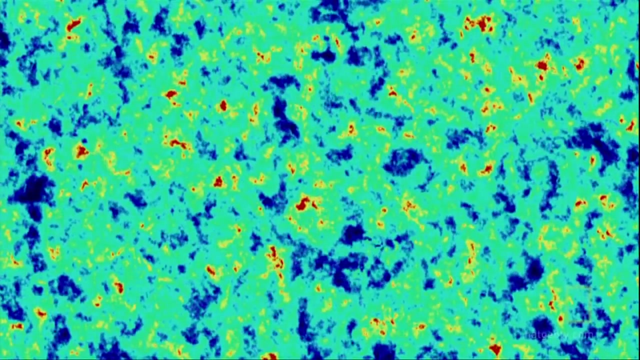 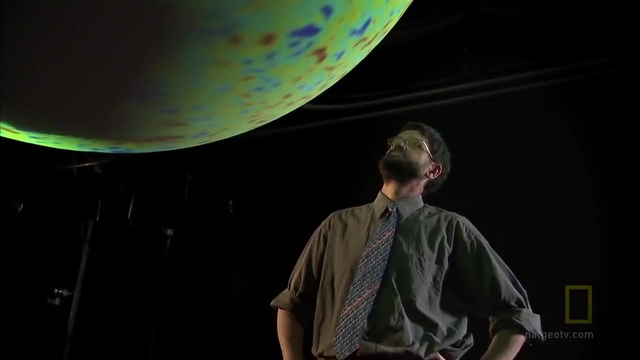 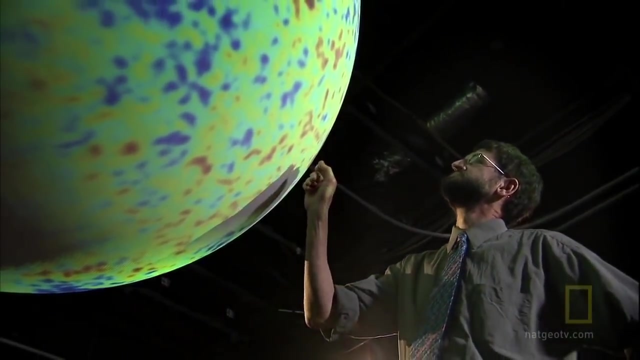 WMAP can see this far back in history. It's confirming important facts about the universe and what's driving it to its demise. The final act for the universe becomes more easily predicted thanks to WMAP Its information combined with the work of astronomers. 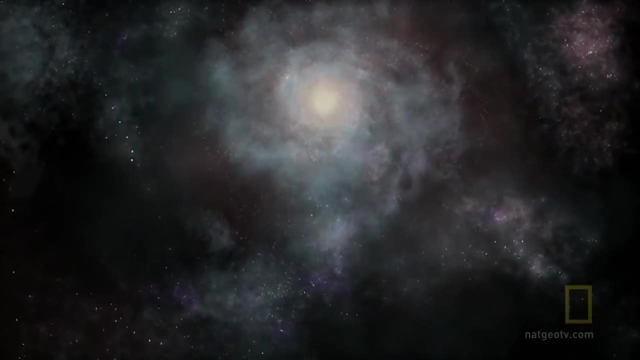 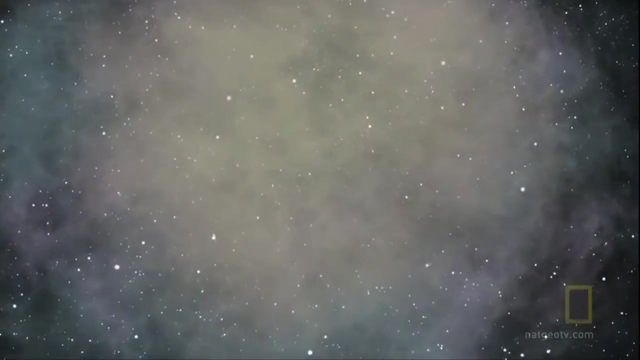 has led to some astounding discoveries concerning a rapidly expanding universe. Rapid expansion supports the dark energy theory and the possibility of a big chill or big rip. We now know from all the data we've had in the last ten years that there's by a factor of two to one.